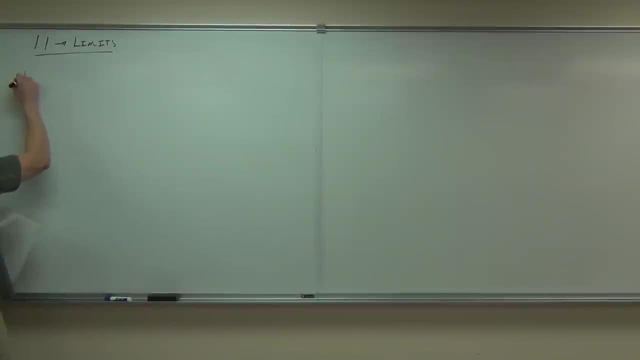 this introductory course to calculus. So here are some of the goals. Goal number one, the first goal and the one that we're gonna spend most of our class on- at least the first half of our class on- is to find the slope of a curve at a point. 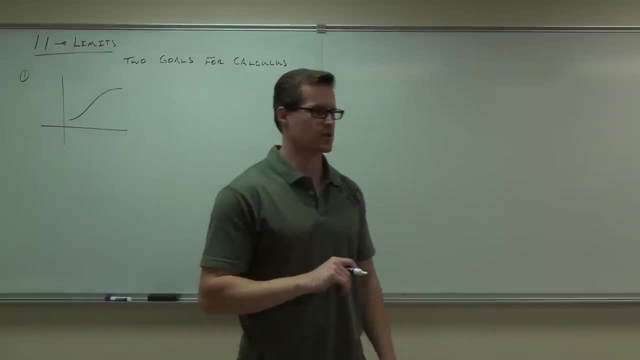 So, given any curve, given any curve, not straight lines. straight lines are easy, but given a curve, I want to be able to find the slope of a curve at a point. Isn't that an interesting idea? If I say to you, I want you to go ahead. 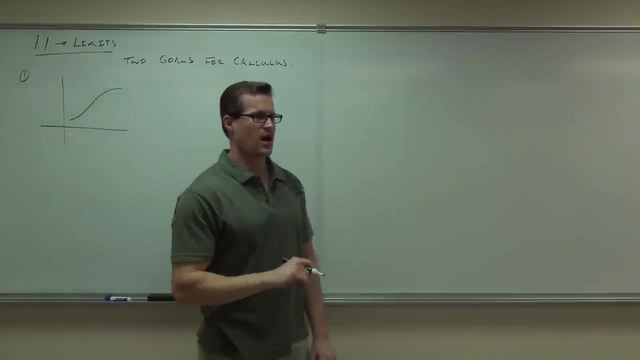 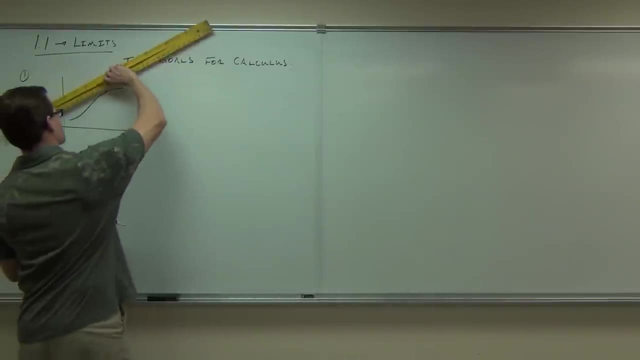 and find me the slope. at that point Right now, we really have no idea how to do it. I mean, you can approximate it, you can go. oh, okay, I'll find the slope. Let's see, slope is. 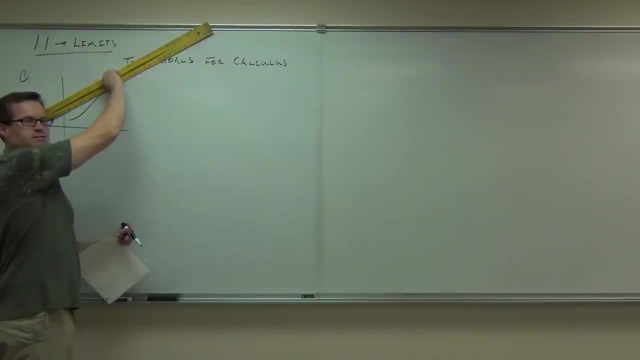 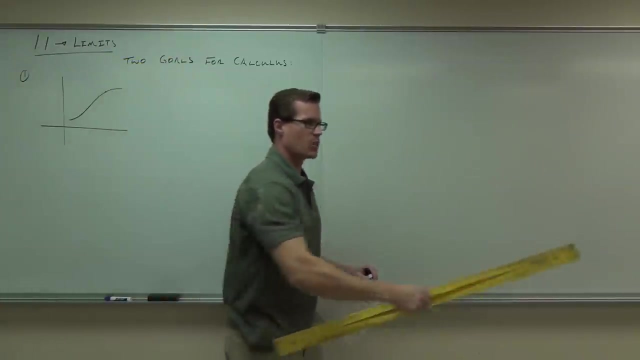 1 1⁄2,. is that accurate? No idea. but we can't really just kind of approximate slope. What we're gonna do is find out a really good way using calculus on how to find the slope of a curve at a point. 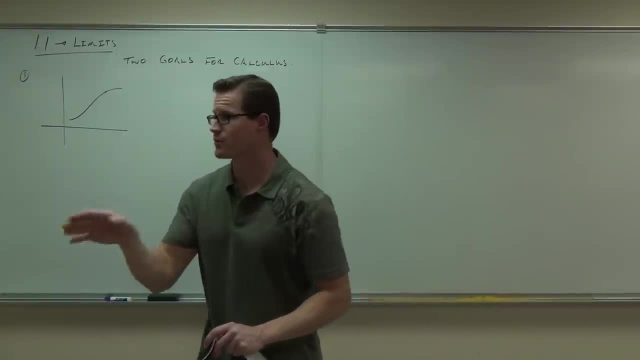 In fact, when I ask you a certain thing in this class, you're gonna say, oh, it's the slope of a curve at a point. We're gonna talk about that for a long time. That's goal number one. Goal number one is to find the slope of a tangent. 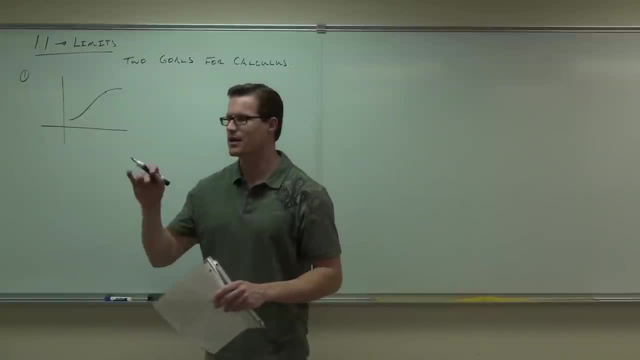 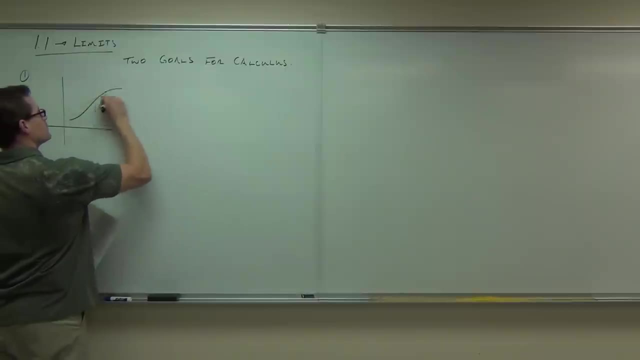 or to find the tangent to a curve at a point. The tangent is the line that intersects a curve at one and only one spot in an area. So goal number one: find the tangent which involves the slope of the curve at a point. That's goal one. 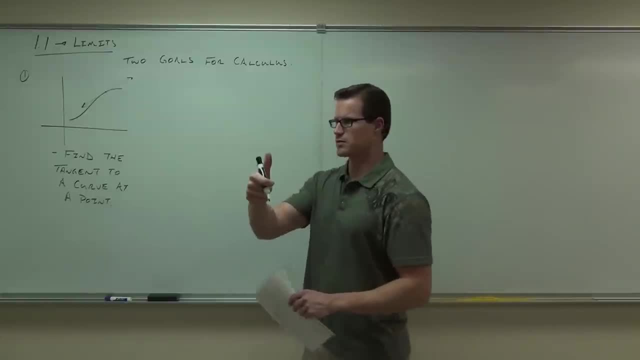 And if we can do that, we're on calculus, fast paced. fast pace. that's good. So we want to take the curve, be able to find the slope of that curve at a point that's gonna lead you to tangent and vice versa. tangent and slope go hand in hand for us. 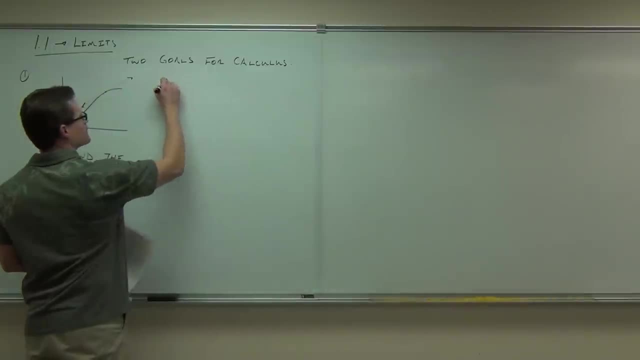 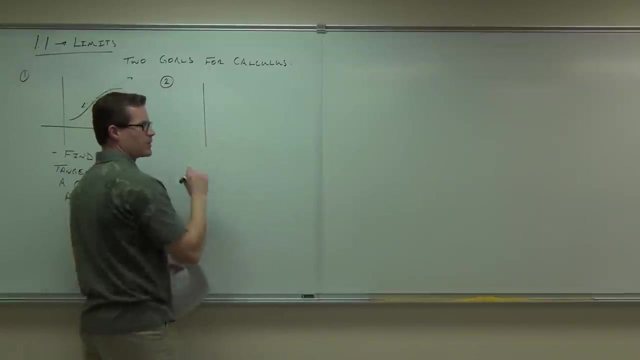 Goal number two, which is the last half of our class, maybe a little less than that goal number two. that's also a really interesting question, So cool, By the way. this stuff is stuff you can't answer in any other class, right? 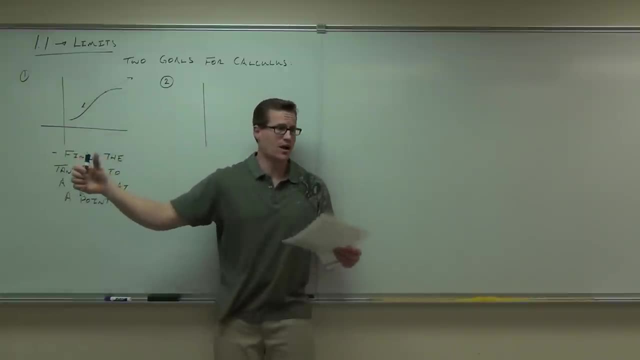 You can't do that, that with algebra. there's no way you can do that with algebra. You can't find the slope of a curve. are you kidding me? Slope of a straight line- easy Slope of a curve. wow, it's weird. 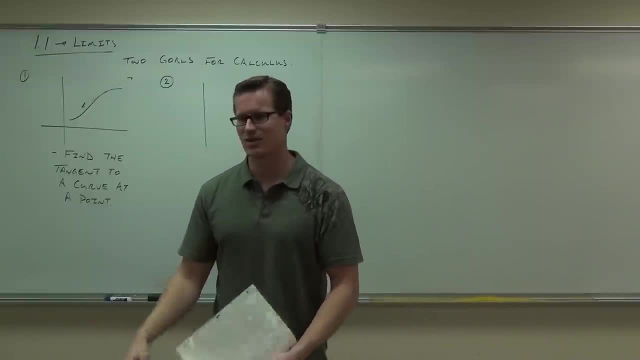 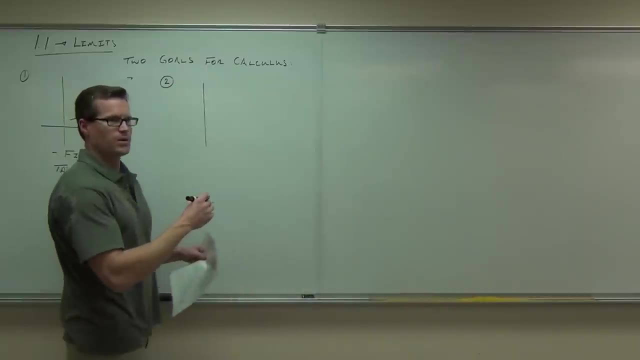 Is that not an intriguing idea to you? It should be. If you're in this class you'd be like that's kind of cool. How are we going to find the slope of a curve? I don't know calculus. The next question is probably even a little bit more interesting. 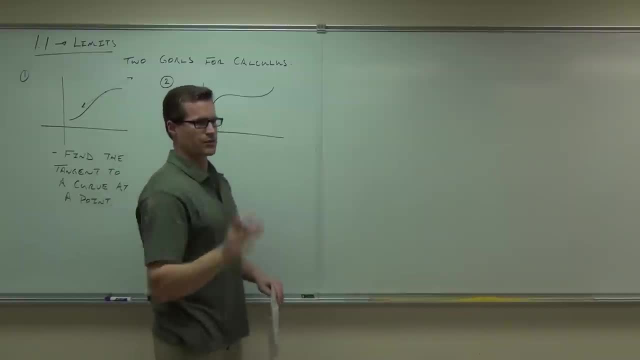 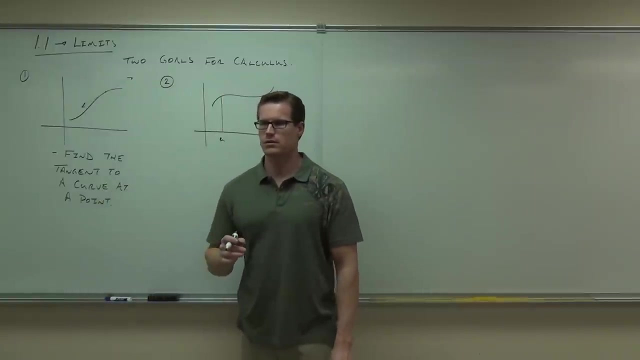 Next question is: let's suppose I have some funky any curve that you can think of, as long as it's defined by a function, Can you, between two points, find the area under that curve? Can you do it? The answer is: right now, with what you know, can you do that with geometry? 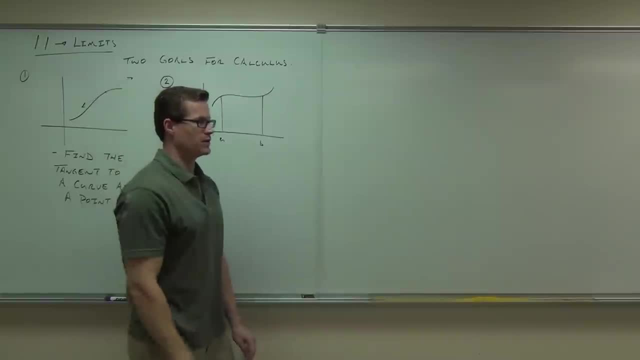 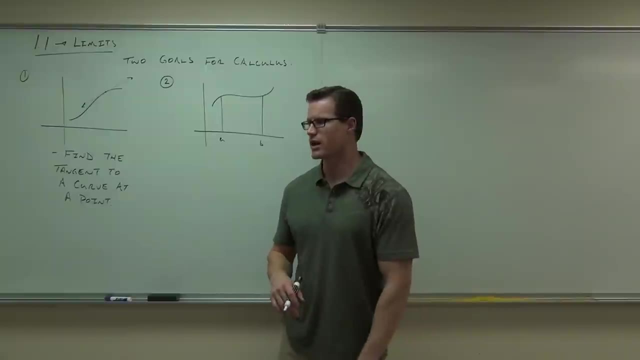 Because I could say, okay, great, find the area of something that's curving. Can you do that? No, No, you can't use the area for a rectangle. that's not a rectangle. You can't use the area for a triangle. that's not a triangle. 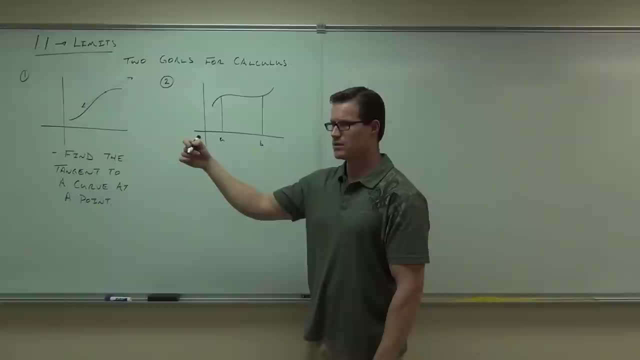 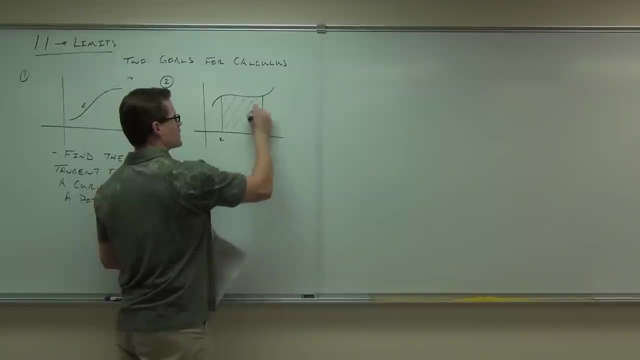 You can't break the triangle, You can't break this up in any way that you have geometric figures can you, Not even circles, not even with radiuses, because the radius is changing. So the next question is: can you find the area under a curve? 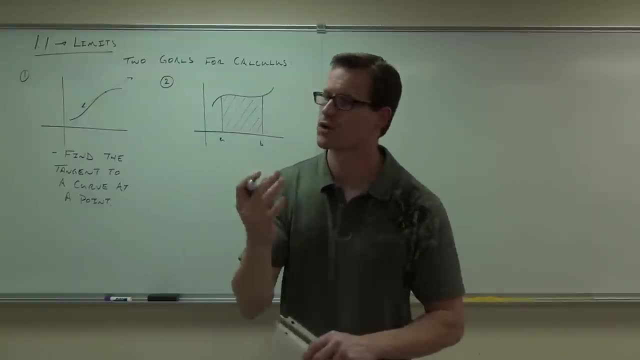 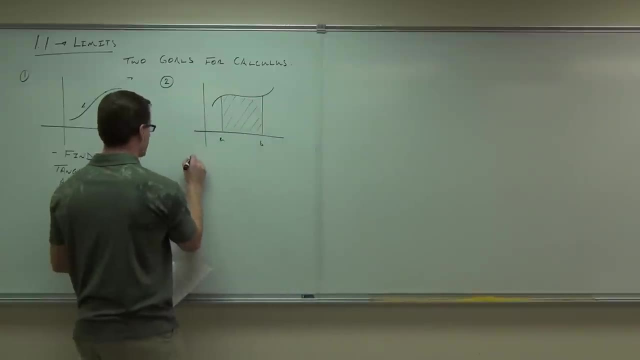 Those are the two goals of calculus: find the slope or the tangent of a curve at a point and secondly, can you find the area under a curve between two points? Interesting stuff, weird stuff, right? It's a crazy question that's going on here. 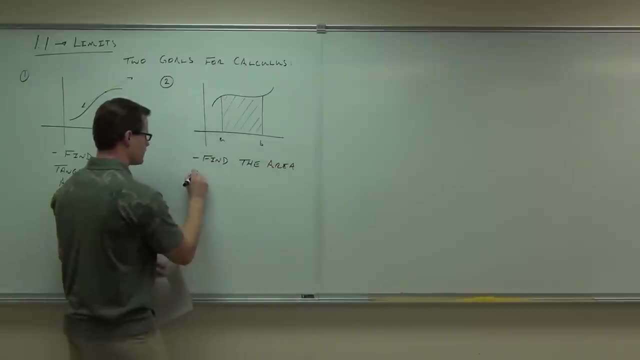 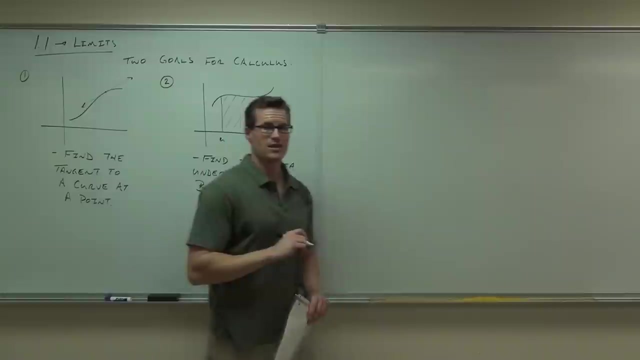 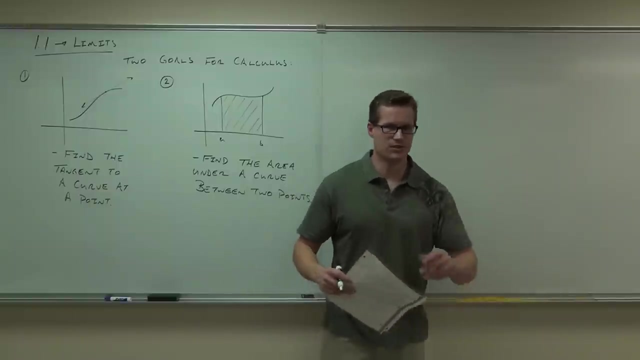 I can't figure we've all. And amazingly it's actually not that hard. This is, I think it's easier than pre-calculus. It's easier than math- Maybe not easier, but if you know pre-calc, this is not such. 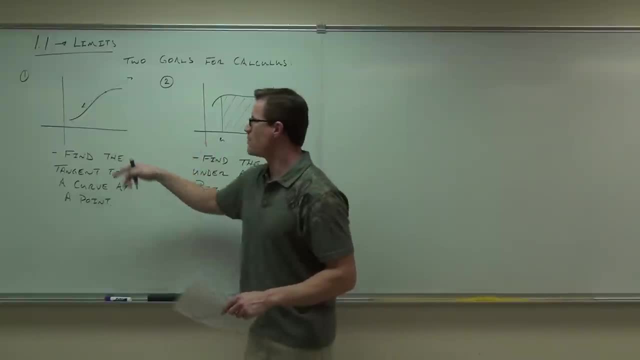 Well, thank you for the lecture. What we're going to talk about first. we're going to talk about the tangent problem. I'll give you a very intro to this, but I'll talk about it later on. We're going to talk about this for most of our day-to-day. 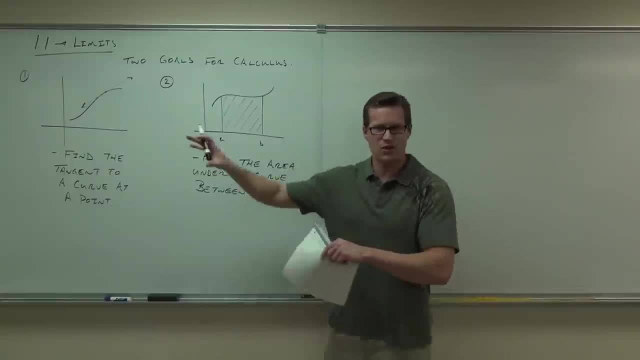 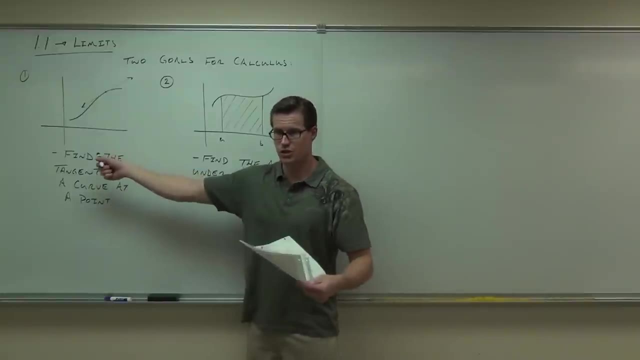 So let's talk about the tangent problem. Are you ready? Do you have any questions on the goals of calculus? Do you understand what the goals are? The goals are A find, the tangent or the slope of a curve at a point. That's what we want to do. 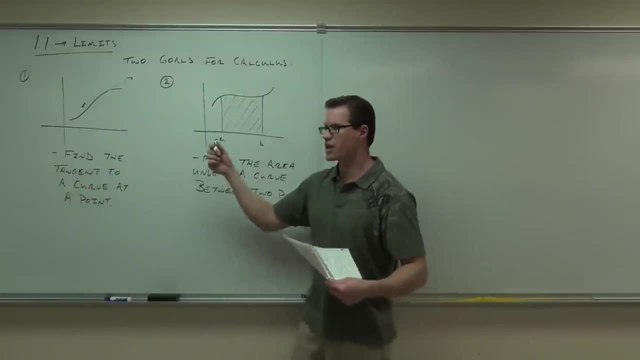 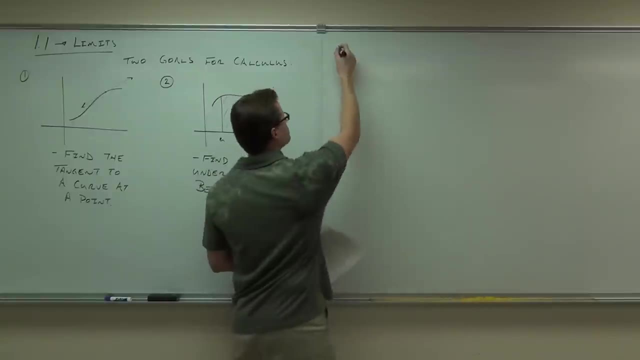 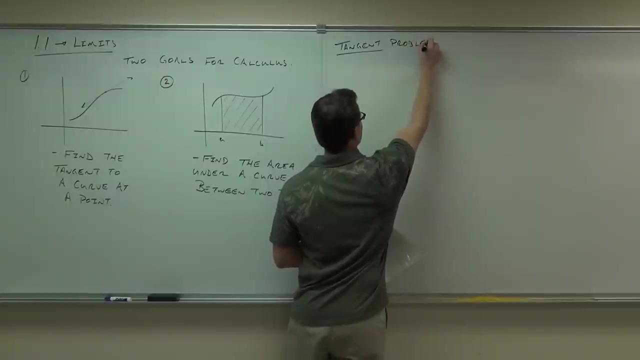 Goal number two: after we finish this, we're going to move on to find the area under a curve between two points. Very cool ideas, So let's work on the tangent problem right after that. You're lucky you're here today. This is it. 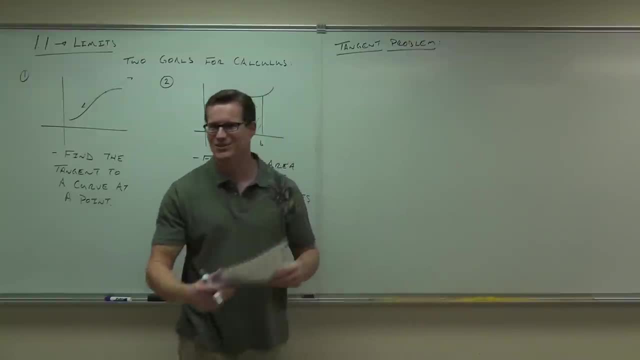 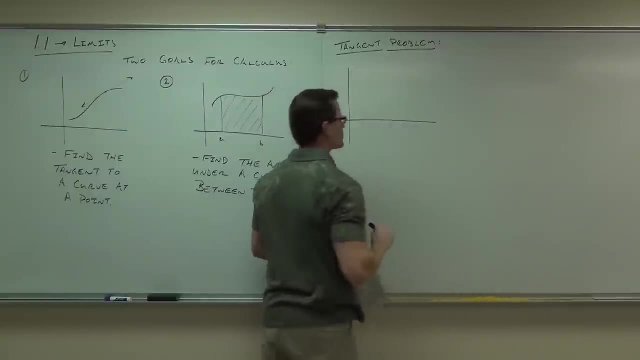 This is like the fundamental idea of calculus. It's so cool. We're going to figure out what a limit is from doing this idea right here too. Here's the tangent problem. The tangent problem says: If you give me anything, If you give me any arbitrary curve. 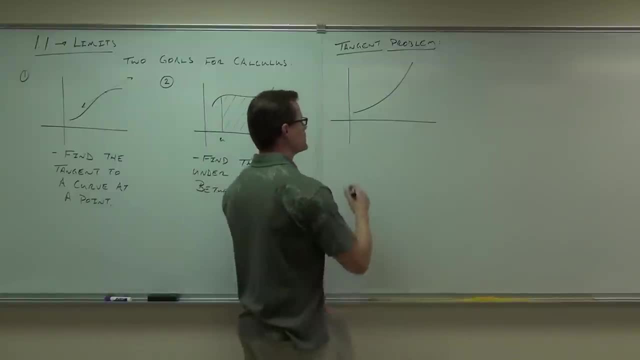 So I'm just making it up. I don't even know what that is. It's just an arbitrary curve. And you give me a point, Let's call that P. Give me a point, Call it P. I want to be able to find the slope of that curve at point P. 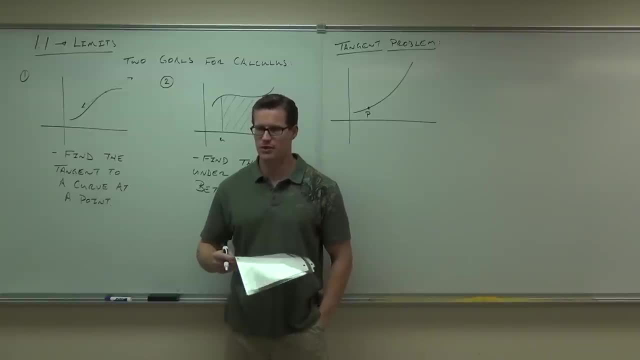 Do you get the idea? We're talking about the tangent problem right now, right Slope of that curve at that point. Because if we have the slope and we have the point, we can make the equation of the tangent. Do you get me? 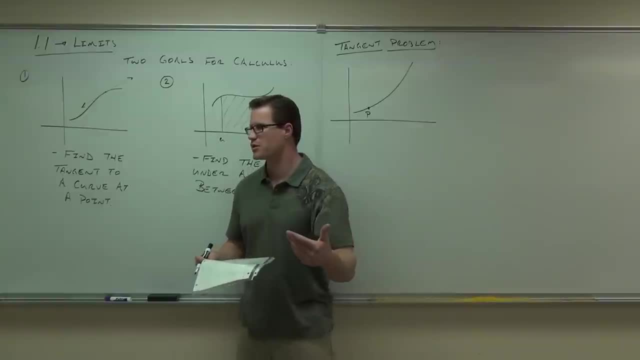 That's pretty easy. That's just y minus y1 equals mx minus x1.. So right now we have the point. What we're worried about is the slope of the curve. at that point, Do you follow? Now the problem is this. 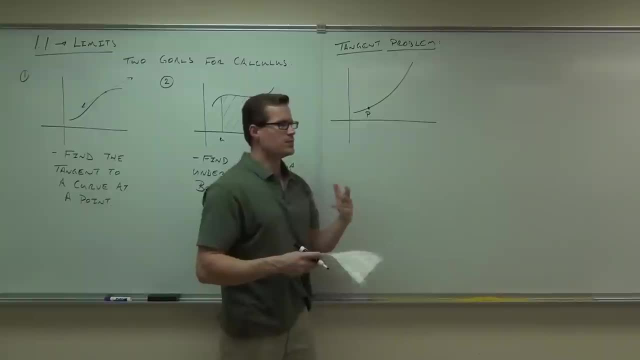 If we're going to make a tangent line. how many points do you need to make up a line? How many points do we have One? That's the problem, right? How are you supposed to make the equation of a line when you only have one point? 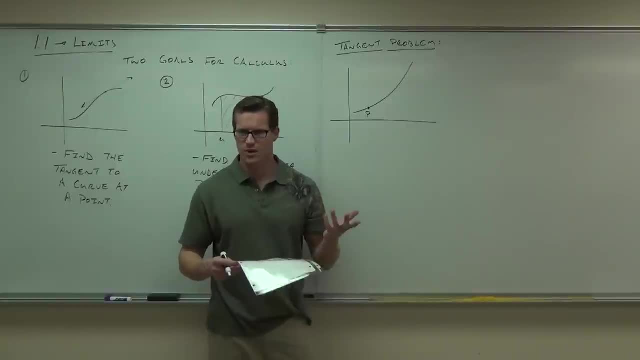 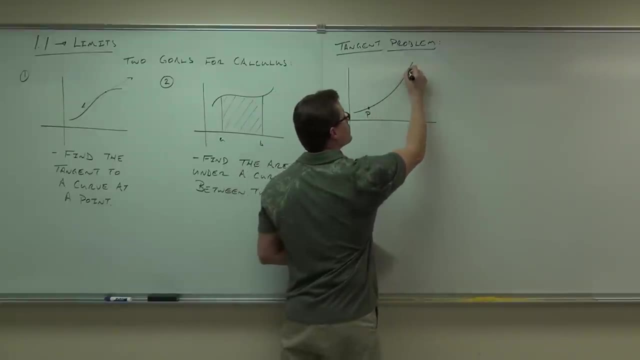 and you don't know the slope. Do you see the issue? That's the problem. So here's what we're going to do. We're going to say: okay, well, let's put some points somewhere else on this thing. How about q? 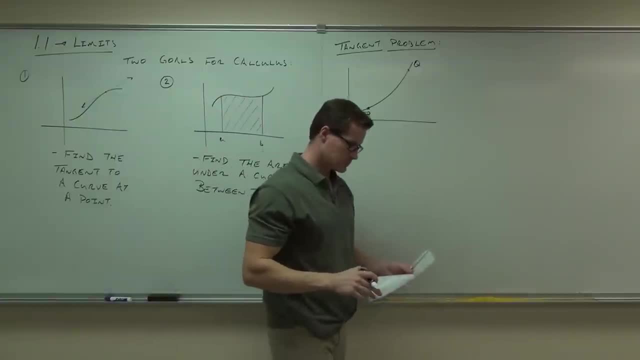 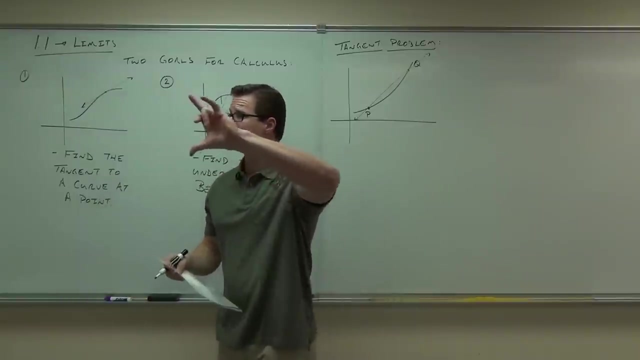 Okay, If I connect these two things, if I connect those two things, do you remember what it's called when you connect two points Together? It's not a tangent, It's a. do you know? It's a secant line. 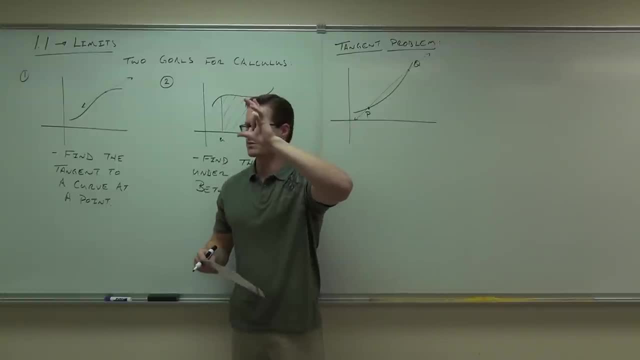 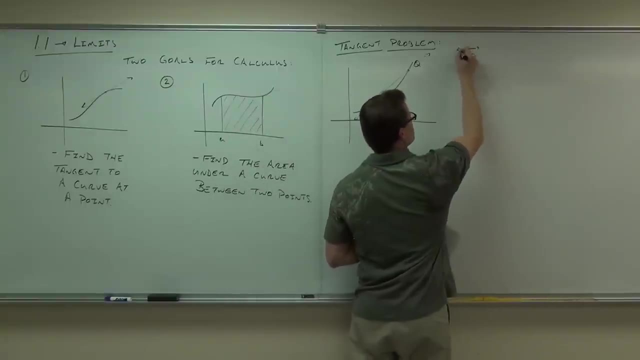 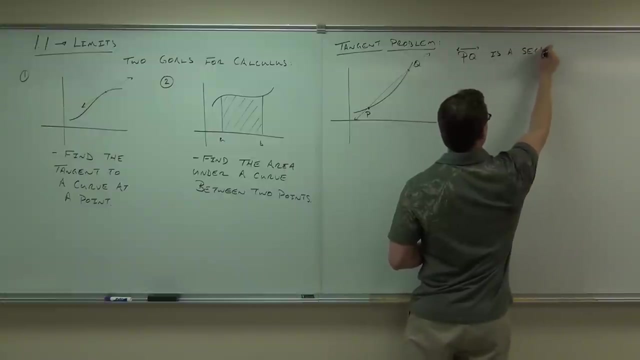 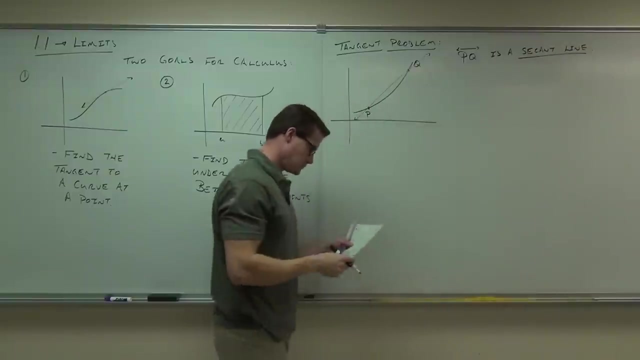 If you've had some geometry, a secant connects two parts of a well, usually a circle, but of any function. So we would say that pq is a secant line. It touches two points of this curve. Now here's the question. all right, 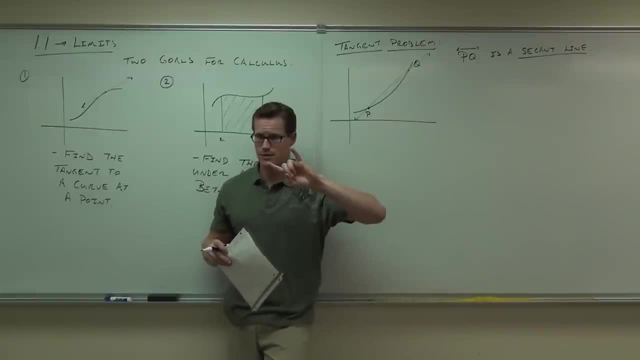 You agree that we need two points for a line- yes, But we also agree that we want the tangent of point p. That's the ultimate goal here. So my question to you is: is pq a good approximation for the tangent? Is this a good approximation for this? 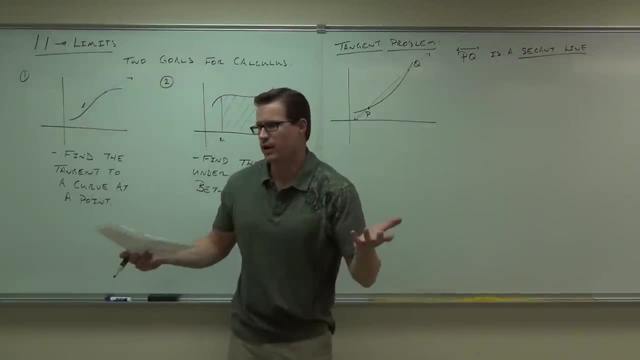 Okay, It's an approximation right. They're both positive. Okay, sure. What I'm asking you is: is there a way- think about this for a second- is there a way that I can make this secant approximation better, to make it more approximate the tangent? 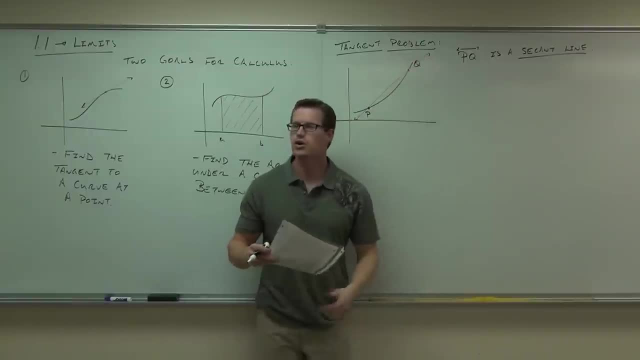 Can I make this a better approximation? How could I do it? Let's assume for a second that p is fixed but q is movable. You can move the point q. I can't move p, but I can move the point q. 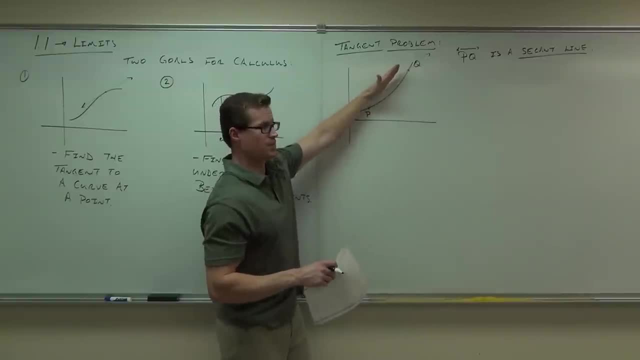 Can you move q to make this? Can you make this secant line a better approximation to our tangent line? Can you think of that? Where would you move q? Would you move it up? Would you move it down Towards the middle? 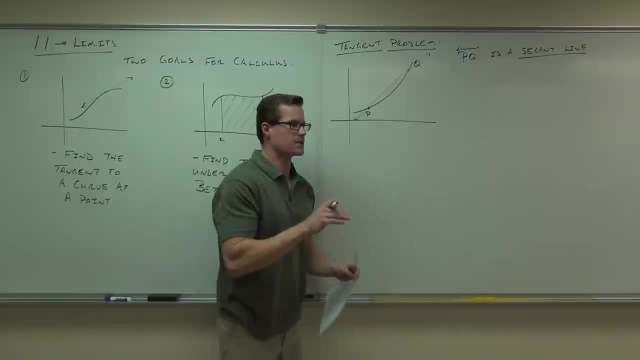 Let's see what happens. It's going to be interesting, So we're going to find out what happens as we move q down this line. So if I move q here, is that better or worse? Better, Better, because I'm going to have- let's use different colors here- that. 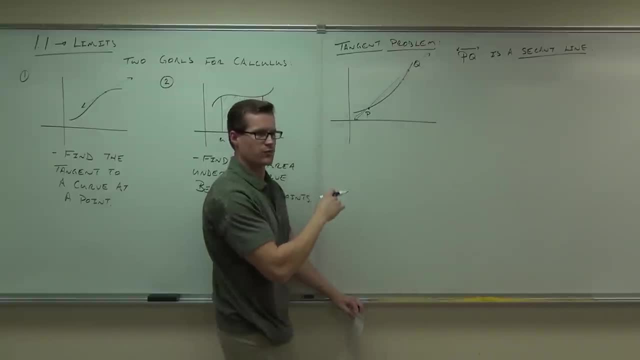 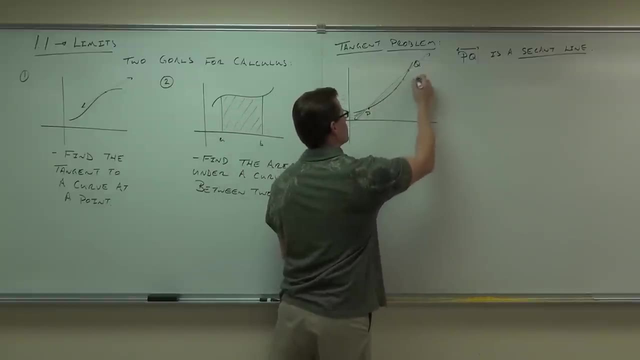 This would be like q, sub 1.. Maybe a different point for q. If I move it closer, is it going to get better or worse? Better, Better, Okay, If I move it closer, it's going to get even better. 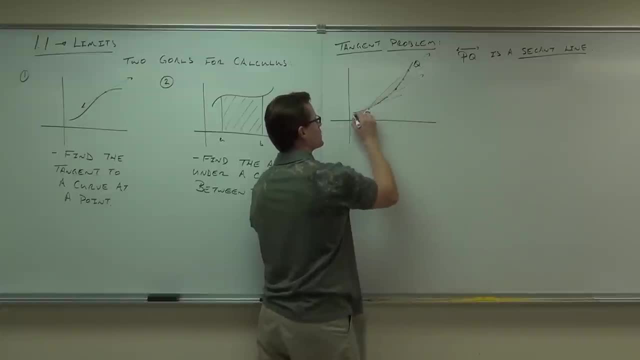 If I move it closer, it's going to get even better. If I move it closer, it's going to get even better. When do you stop? Can you move it really really close? Can you move it? so q and p are the same point. 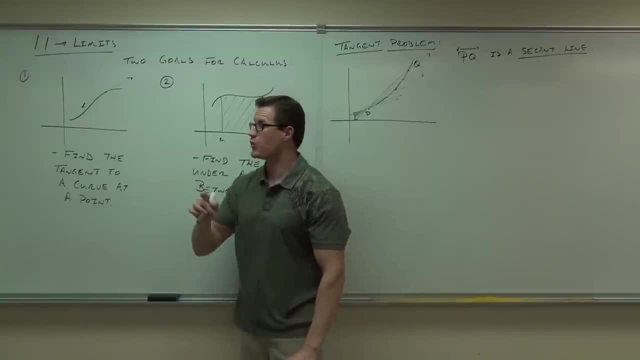 No, Why not? No, Why not? Because then you only have one point. How many points do you need for a line Two? We need two, So can we move it close? The answer is sure. We're doing it right now. 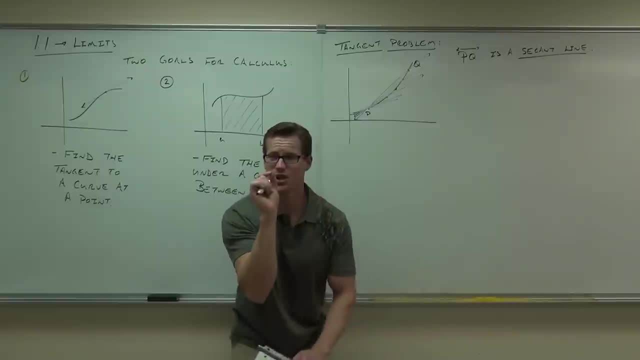 Can you move it close? Yes, Can you move it so close that there's no difference between them? Yeah. Can you make it the same point? No, That would fail because we need two points. I don't care how close they are, but you need two different points, right? 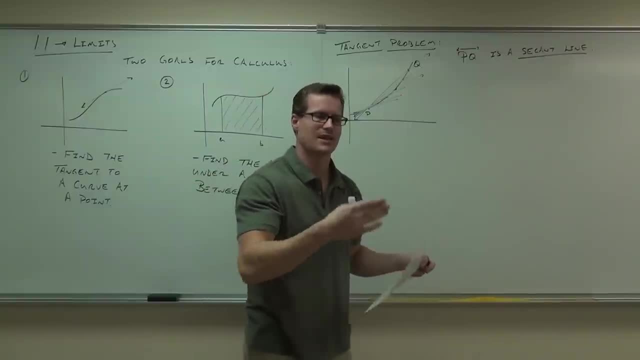 If you have two different points, you can make the equation of a line. That's great, That'd be fantastic. That's our idea actually. So we're going to try to move the point q really, really, really really. 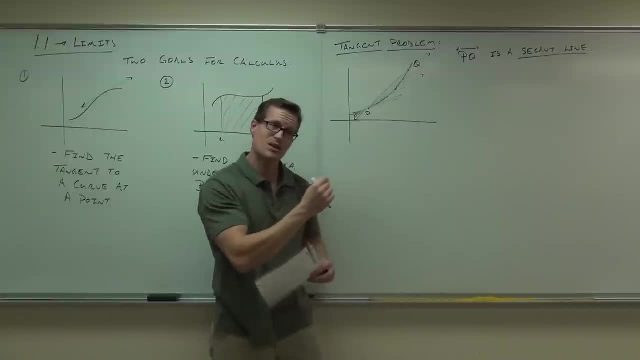 really close to the point p, If we can move it really really, really, really, really close- that's math speak, by the way- really, really, really, really. That means very, very, very, very, And if we can move it really, really, really close. 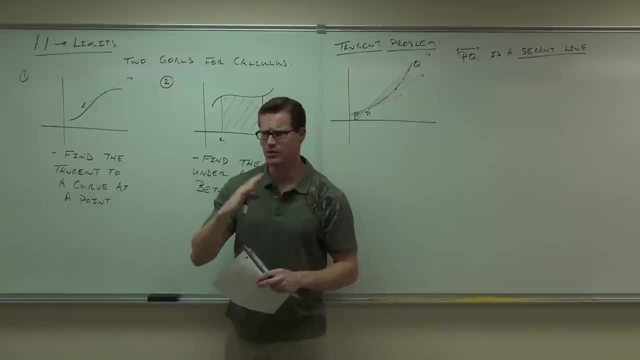 then our secant line is going to be really, really, really, really close to a tangent line. Do you agree with the idea? So you take this point, You go, let's move it really close, Not really far away. That's a sucky approximation. 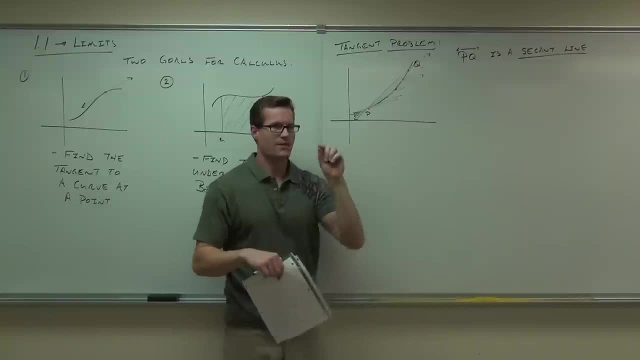 Well, if you move it really close, move that secant really close, that point really close, that secant is so close to a tangent line that it's not going to make a difference. That's the idea. So let me write some of this stuff out for you. 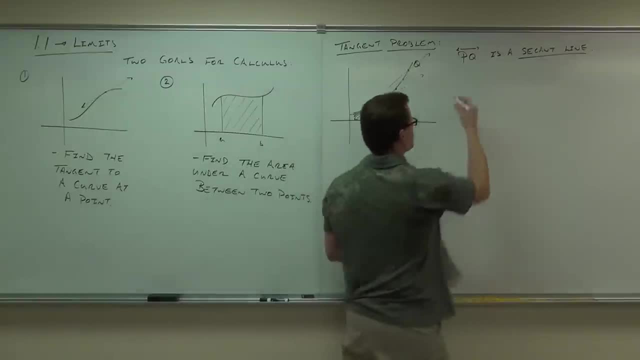 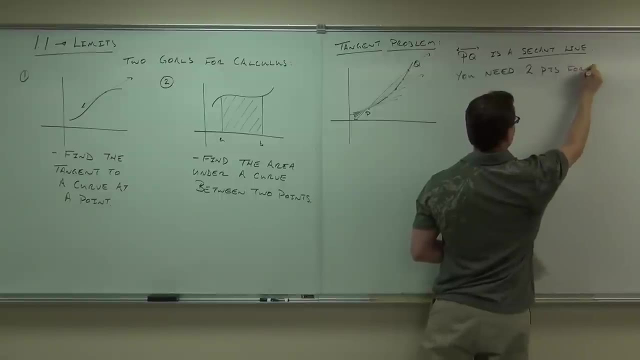 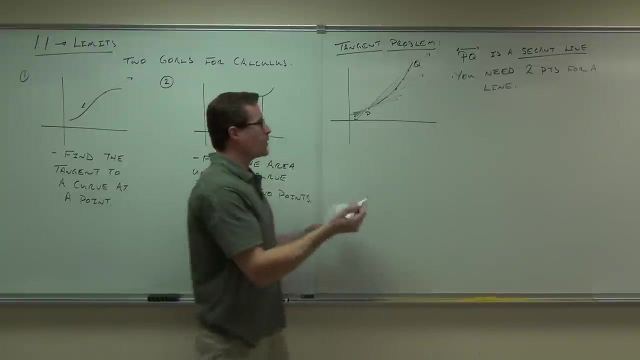 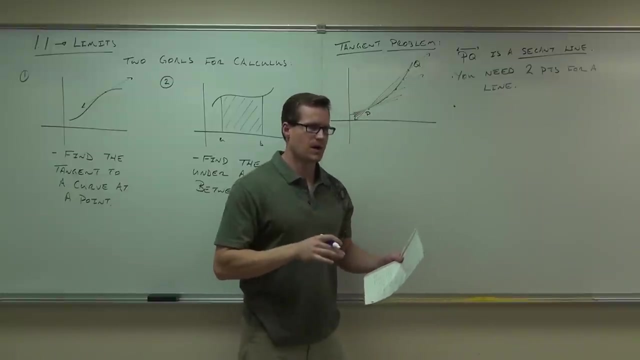 So what we're doing right here? we need two points for a line. Sure, We understand that. Awesome. So we have the points P and Q. Well, the question we're asking is what happens as Q gets closer to P? And the answer is: as Q gets closer to P. 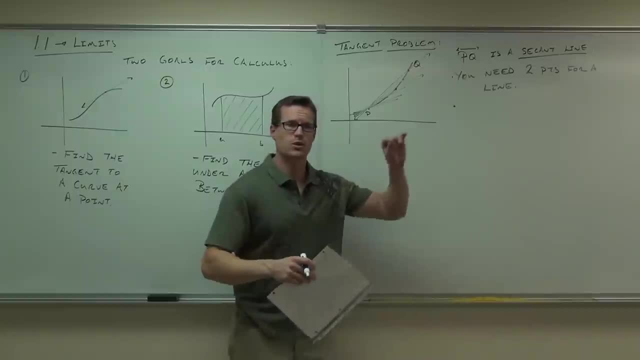 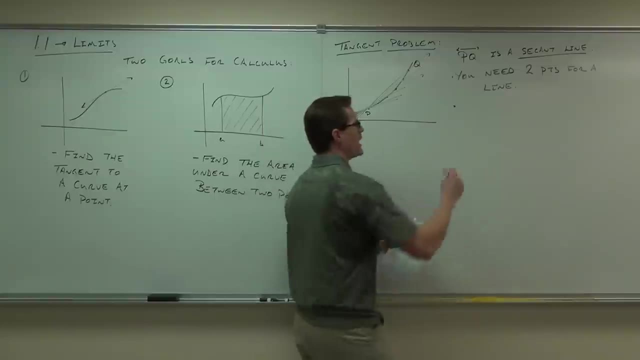 but we just talked about this. we just said this. this is nothing new. As Q gets closer to P, the secant line more closely approximates the tangent line. Not sure if you understood that at the first time. So as Q approaches, I'm going to use that word. 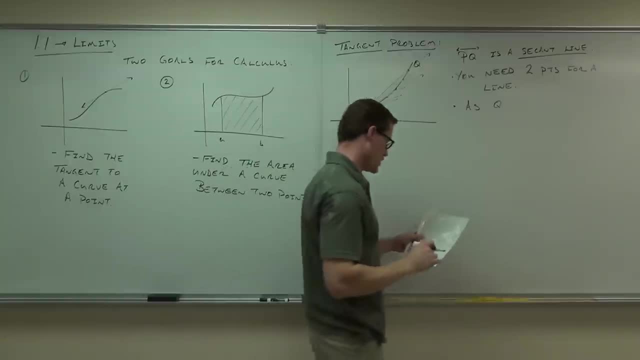 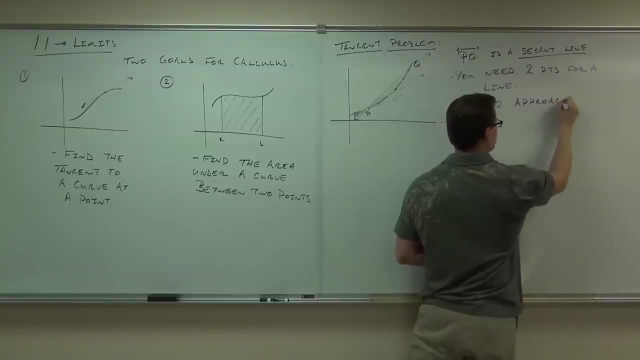 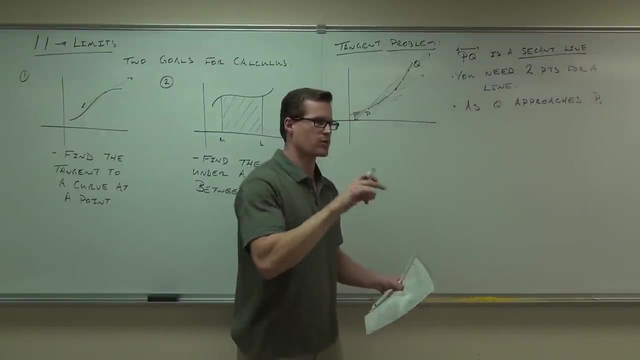 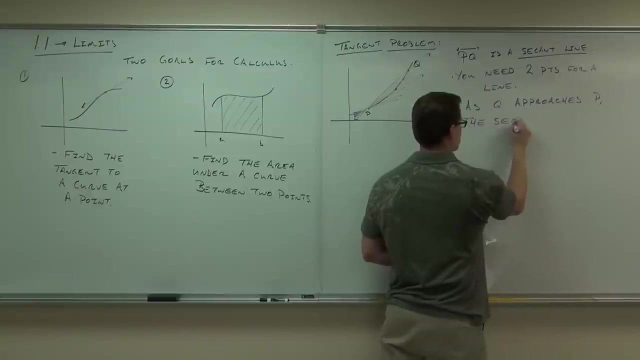 we're going to use that word limits as well. approaches, that means gets closer to As Q approaches P We get closer to a tangent, or in other words, the secant more closely approximates the tangent. Okay, Well, that's great. 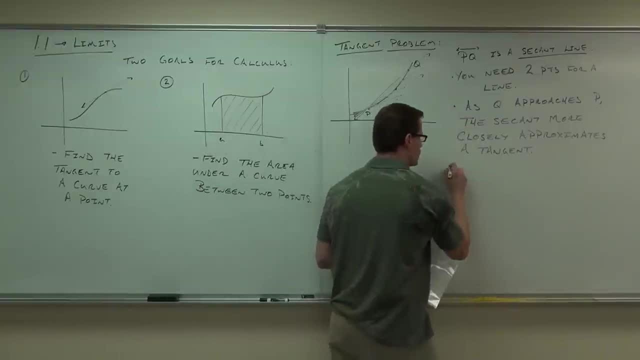 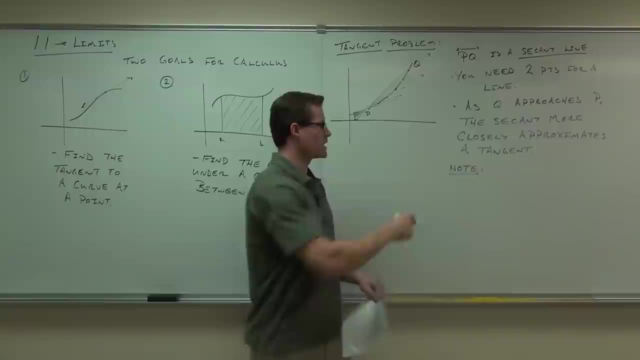 That's great. Oh, one more little note. Why was it that we can't just let Q equal P? What was the reason? Why can't we just say, oh, it's moved to P, Because there wouldn't be a difference. 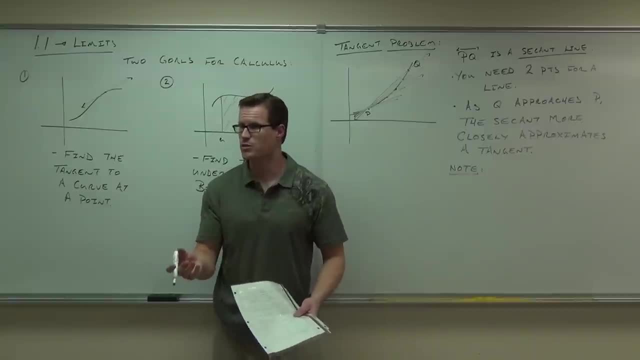 Okay, There wouldn't be two actual points for the same point twice, and that's a problem. You couldn't make an equation of a line with that. So one little note: we can't just let Q equal P, because we need two points to make a line. 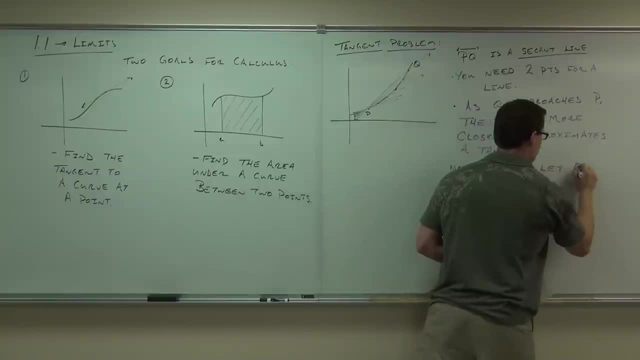 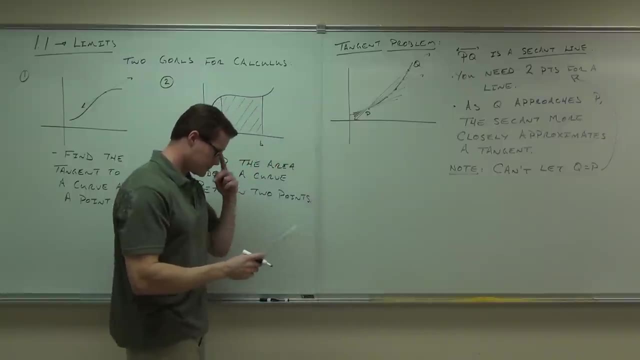 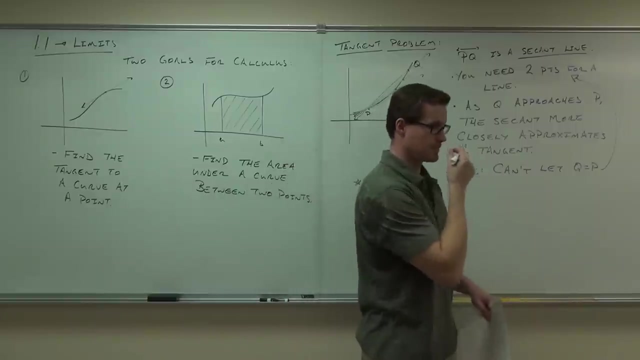 Okay, You need two points. That would be a problem. Here's the idea of a limit. all right, This is a big big idea. Here's the big big idea for limits. okay, The idea is: how close can you get one point to another? 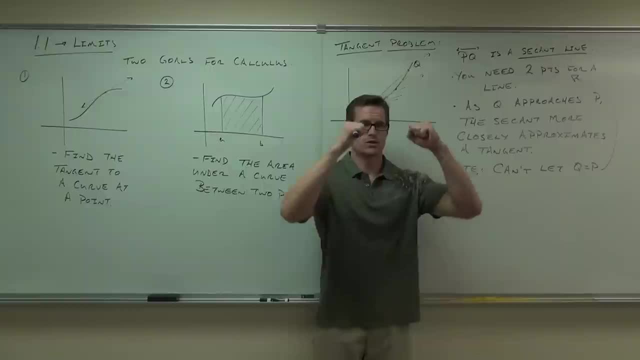 without them being the same point. So let's say I have two points like this. Can you find some space between it? Let's say I move it over to the midpoint. Can you find some space between it? Let's say I move it over to the midpoint. 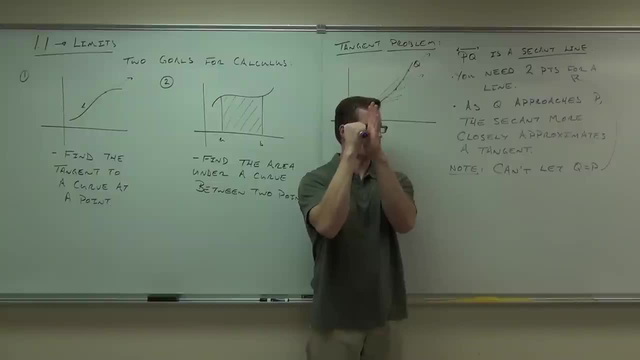 Can you find some space between it? Can you keep doing that for eternity? Between any two points there's a gap. In that gap, you can fill it in with another point, because points have no breadth. That means that even though we draw them on the board like this: 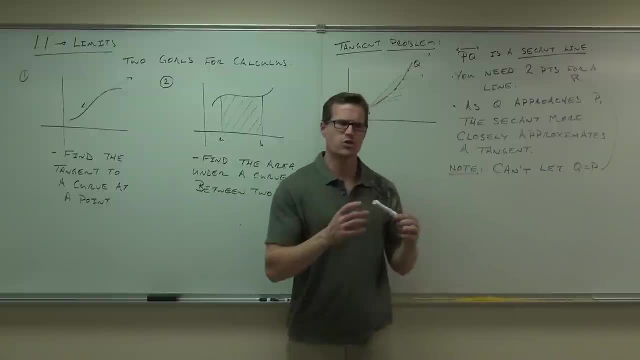 they really don't have any distance between them. So two points can get, would you agree, infinite distance between them. Intestinally close to each other, That means so so close that you can't put anything between them. but there's still so little distance. 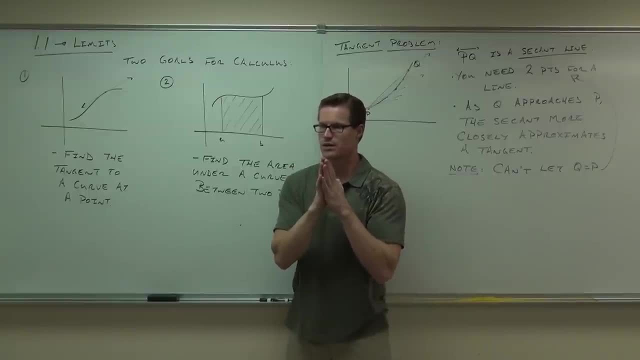 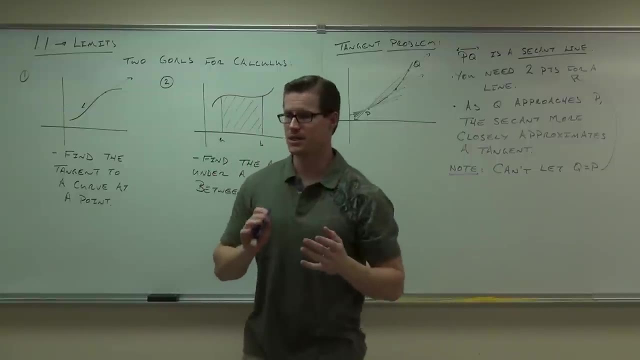 and then you can get even closer to that, and closer to that, and closer to that. Would you agree to that? So here's the idea behind calculus. It says we can get Q so close to P that there's literally no difference between the secant and the tangent. 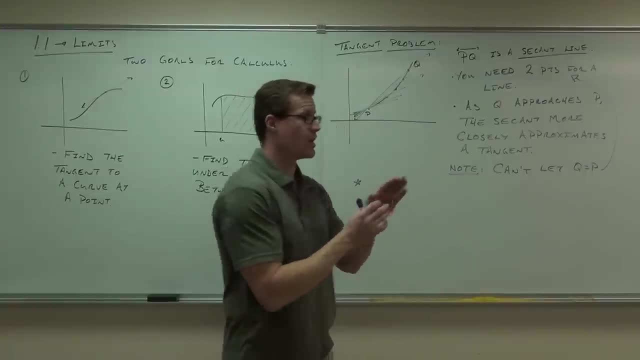 We can get it so close- We can't let it equal, but we can get it so close that the secant line is the same as the tangent line. That's the thing. That's the idea of a limit. Isn't that kind of an interesting idea? 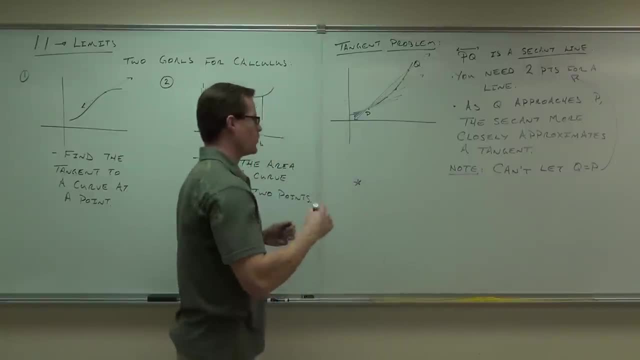 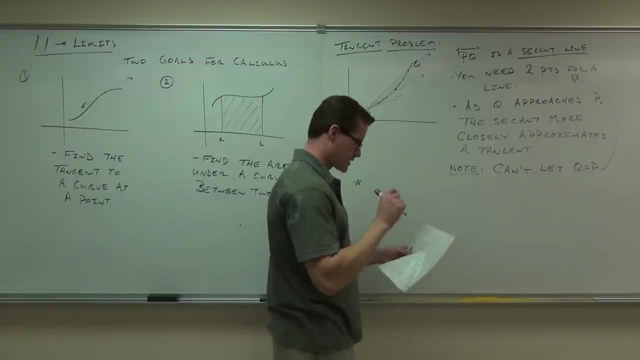 Yes, there are different points, but they're so close it doesn't matter. That's the whole idea. So the big picture for our limits is: if we let Q get really, really, really close to P, the secant will be identical to a tangent. 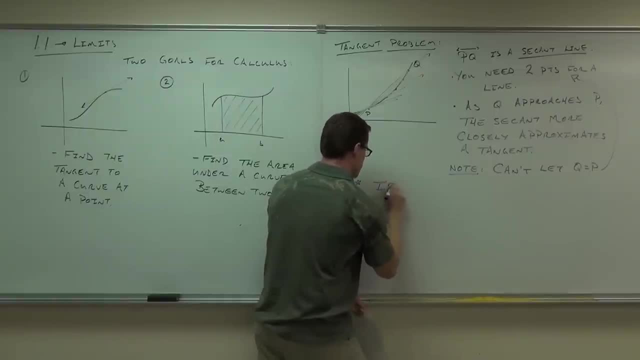 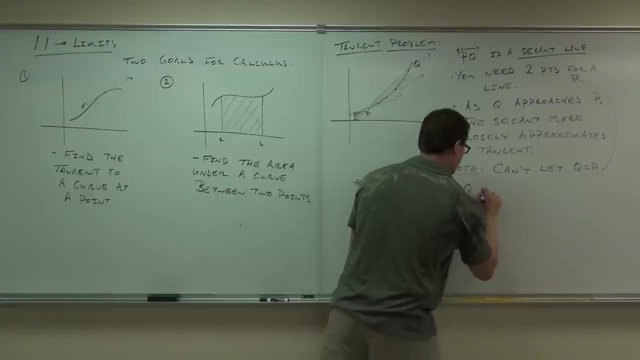 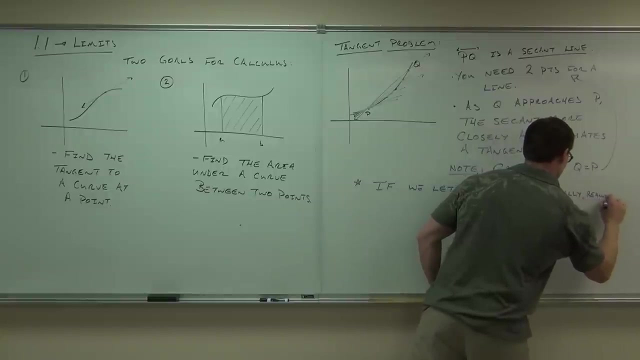 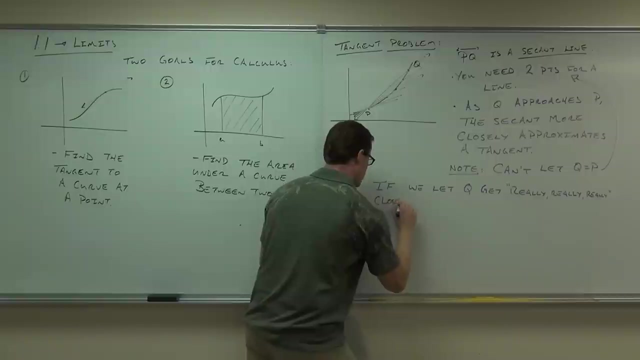 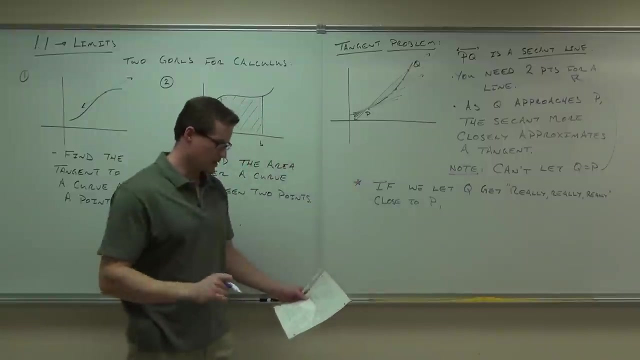 Let's see again, Or approximate it so close that it doesn't matter If we let Q get really, really, really close to P. I'll use a better word to express it. I'll use a more napkin word for that in just a minute. Really, really close to P, the secant will be identical to a tangent. So if we let Q get really, really, really close to P, the secant will be identical to a tangent. Let's see again: If we let Q get really, really, really close to P, the secant will be identical to a tangent. 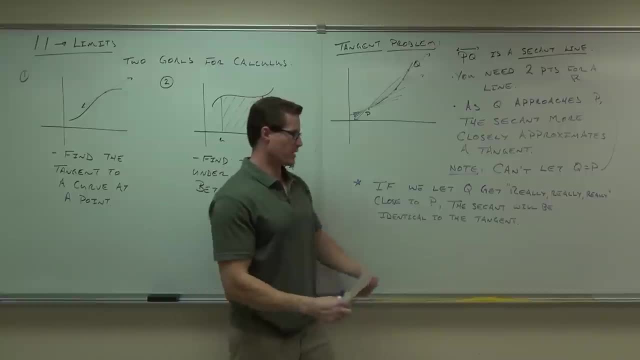 Here's the idea, right, Here's the idea. Now I'm going to replace this really, really, really, with a key phrase for you: The idea of Really, really, really, The idea of moving P or Q really, really, really close to P is called a limit. 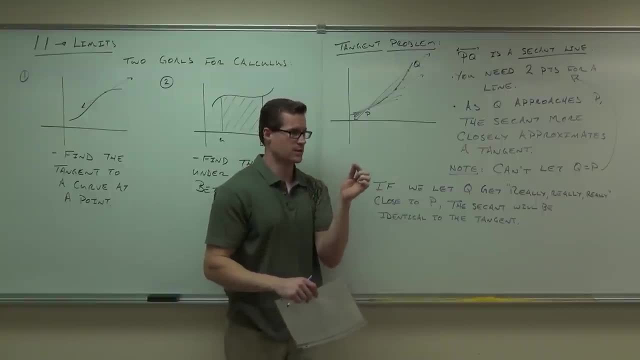 Moving something really really close without actually getting there. That's the idea of a limit. Do you kind of understand the idea of a limit? We would say that Q would be in a limiting position. That means we've got it all the way really as close as we can to P, but it never touches P. 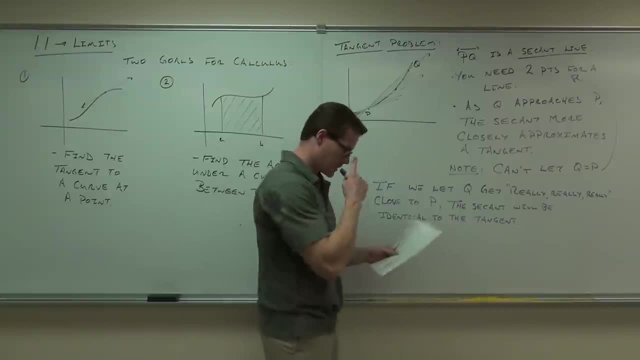 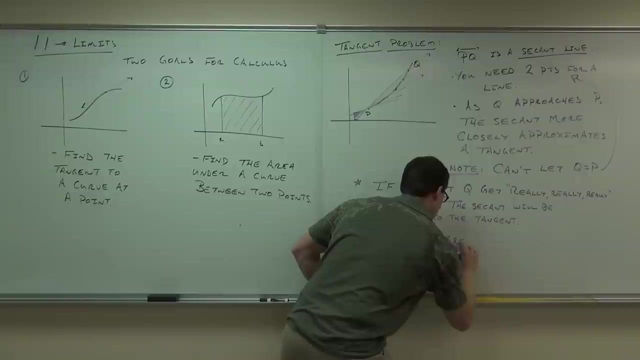 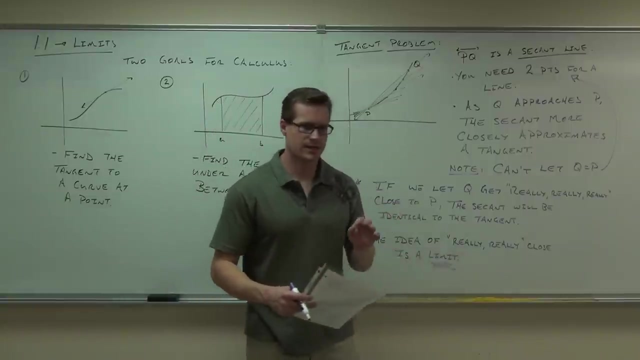 That's the idea of a limit. It gets really, really close. So the idea of really really close is a limit. All right. In the most simple terms, This is it, All right. Would you like to see an example? 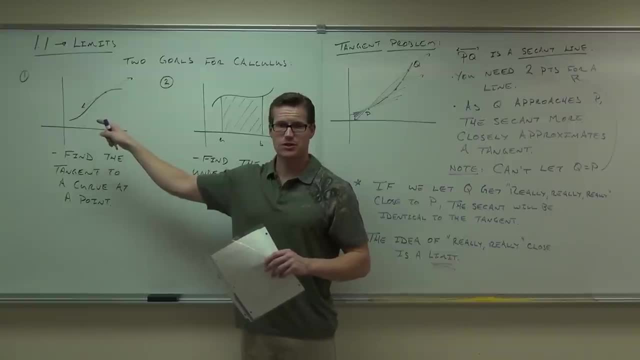 How, How, How, How, How to actually do this? Would that be interesting to you? How to find the slope of a curve at a point. You wanna see that. It's kind of fun. Okay, we're gonna work through this. 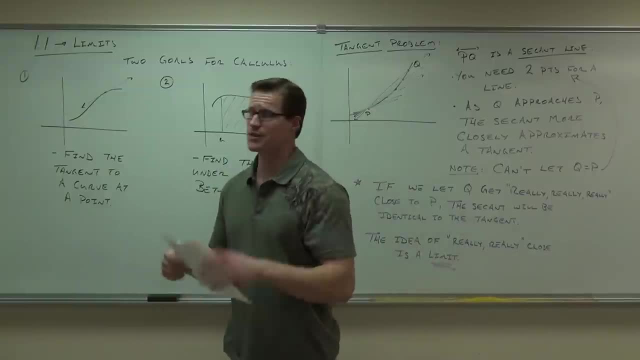 I'm simply doing this to give you an understanding of how limits work and the jump that you can make. okay, We're not going to be doing a whole lot of math like this. I'm just giving you an introduction right now so that you see it's possible with some real math stuff. 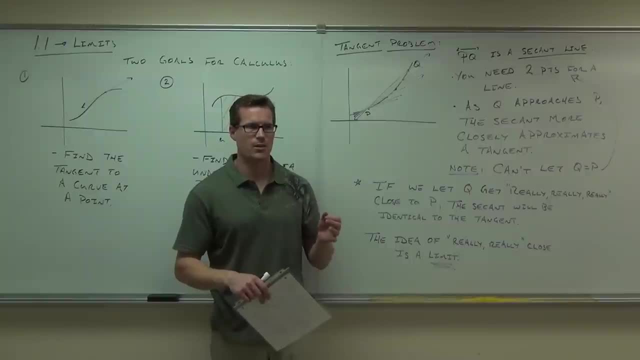 that you've had before, without actually teaching you limits and calculus. I'm gonna make one limit jump in this problem. I'll show you what it is, But this is stuff that you could actually do. We're just gonna use calculus to do it better. 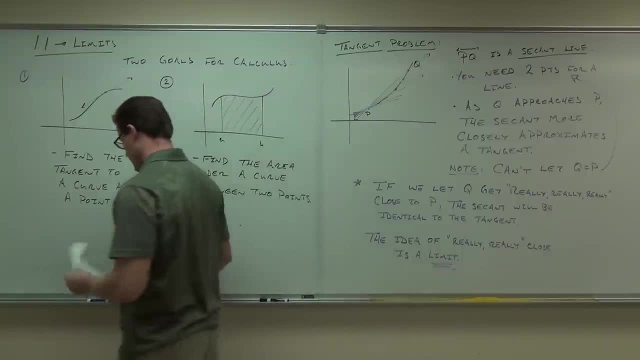 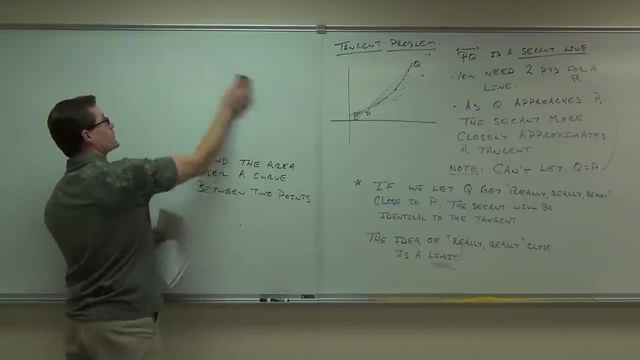 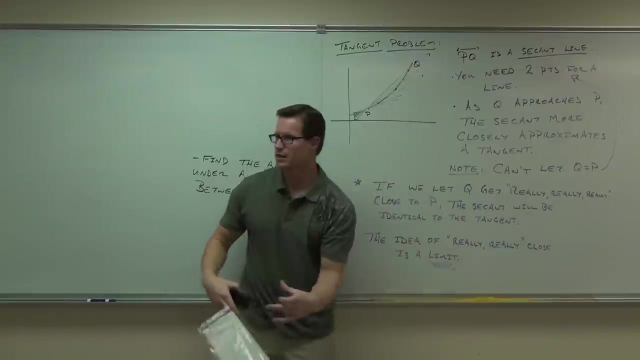 You ready for it? Do it more mathematically Before I go any further. did you guys understand the tangent problem? Nod your head if you're okay with the tangent problem. You understand the idea of a limit, Moving a point really close to. 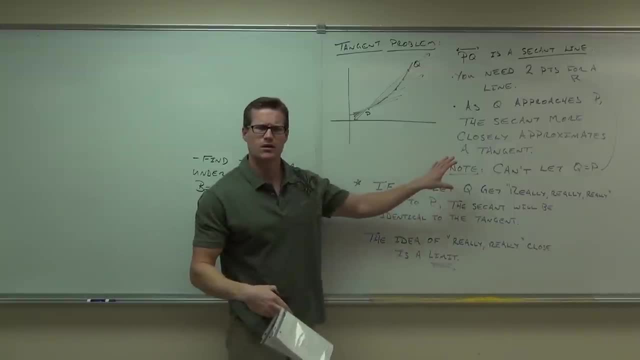 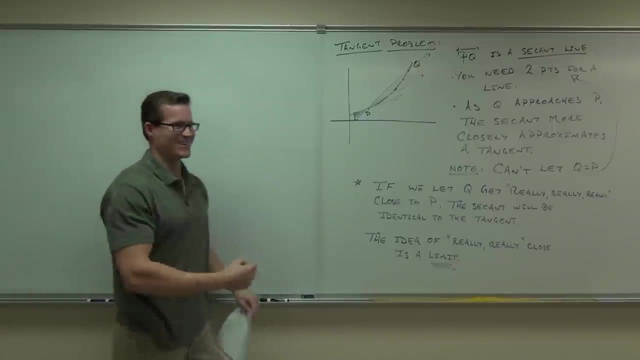 but never actually getting there. Again, why can't we get there? You need two points. yeah, they'll be fine. Okay, cool, now we're ready. now I'm excited. First little step off into calculus land. Do you trust me? 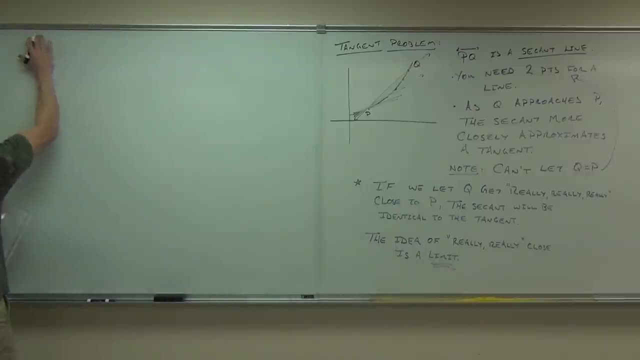 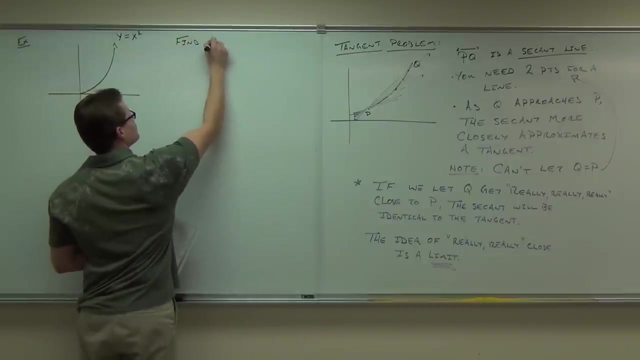 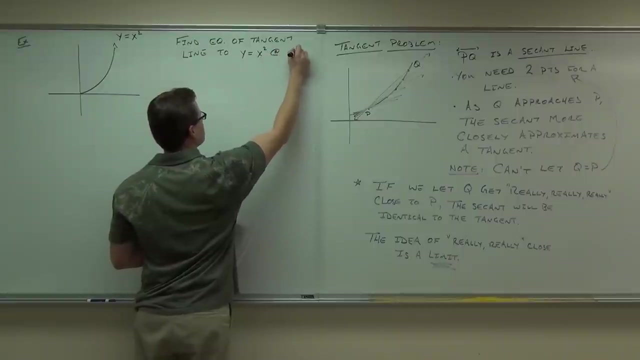 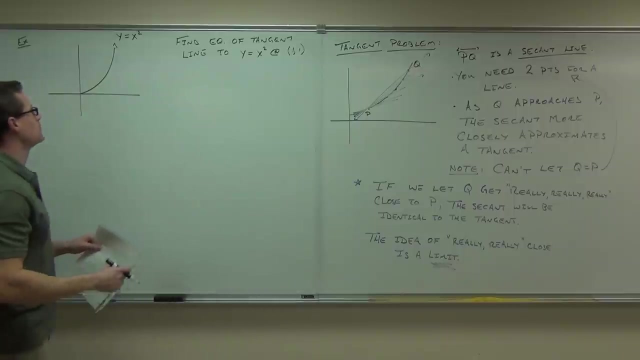 You shouldn't. Here's the goal to this problem. I want us to find the equation of the tangent line to this curve at a certain point, Specifically that one, One one. Well, let's go over to one one. 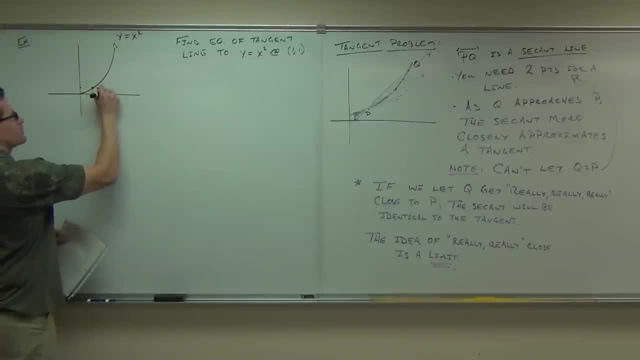 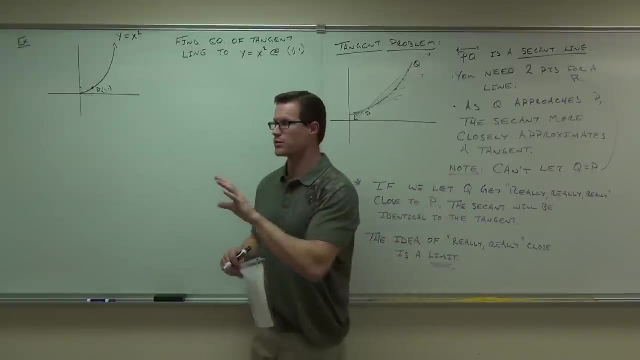 and let's put a point there. So P is the point one, one I'm gonna walk you through how we're gonna do this right now. okay, I'm gonna walk you through how we're gonna make up a tangent line using this idea. 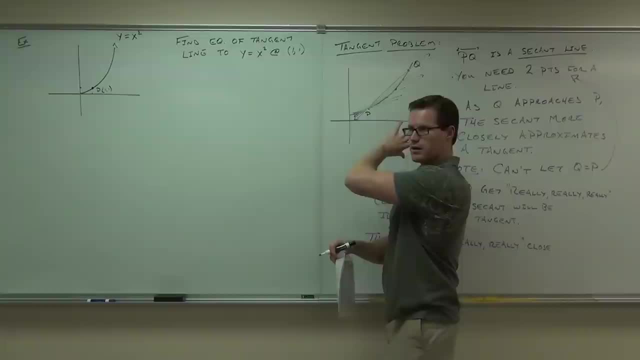 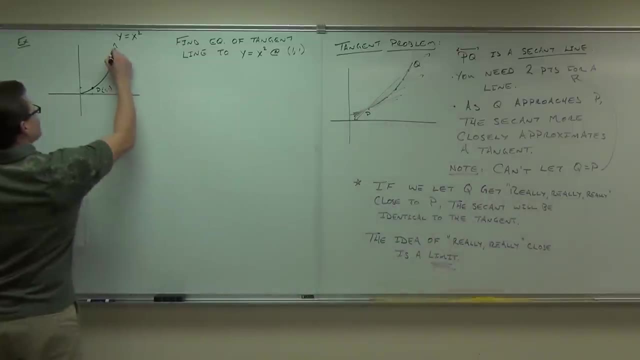 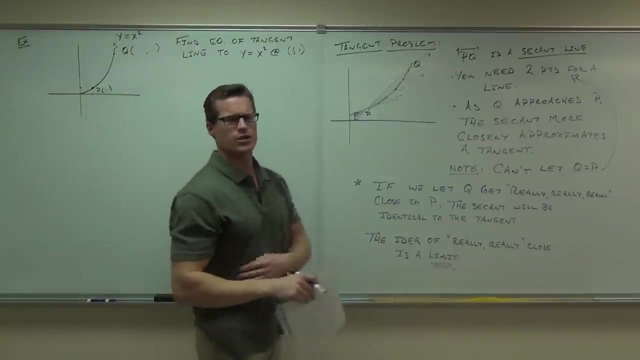 Are you ready for it Over here? on this idea, we had two points right: P's set in stone. you're not gonna move P. What other point do we have? We're gonna make a point Q- Q. What's the coordinates for point Q? 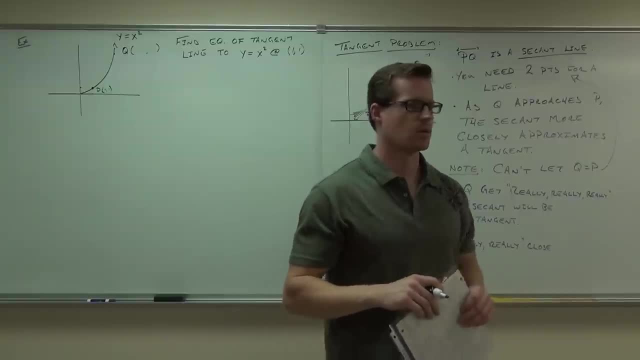 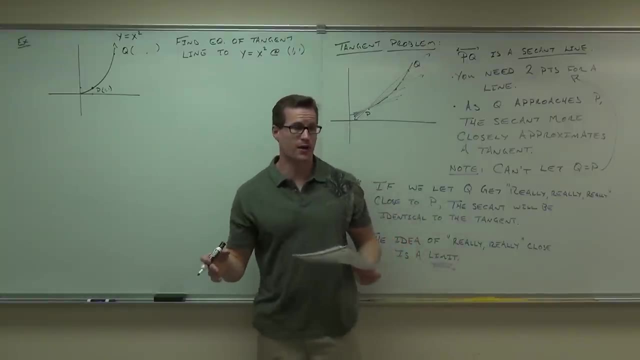 Why don't you tell me What's the coordinates for point Q Two, We can't use actual numbers, right, That wouldn't be very good. so I know two, four would be on there and three, nine would be on there. 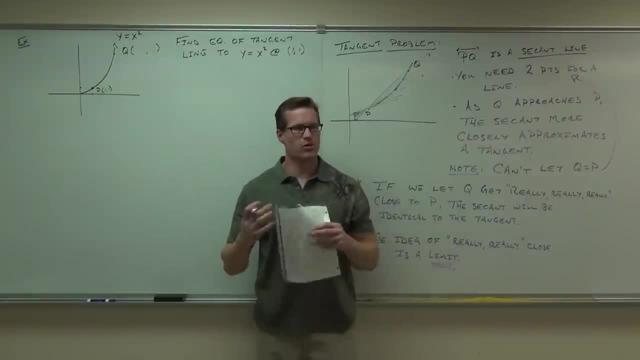 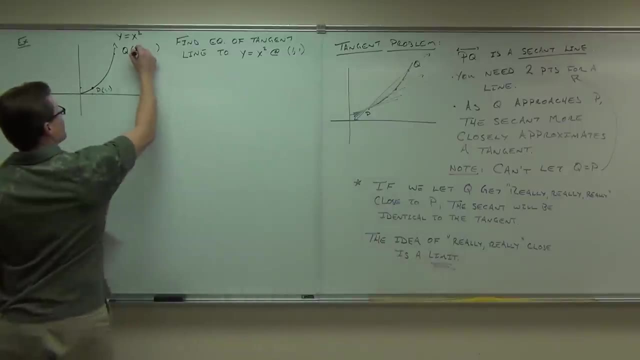 four, 16, and so on. But I want you to use actual points In general. what are the points for? what are the coordinates for any point? X, Y, X, Y, Very good, Okay, Very good, Okay, xy. So now write down xy and have your eraser handy. Have your eraser. 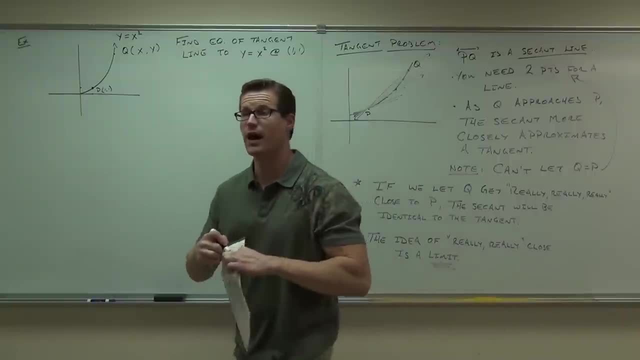 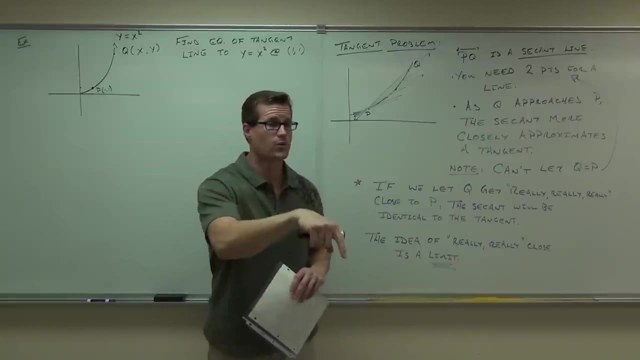 handy, because I'm not going to have xy. I want to keep this in terms of one variable. Now, using your knowledge of what the function is, what's the function? y equals what. Say it again: y equals what y equals. 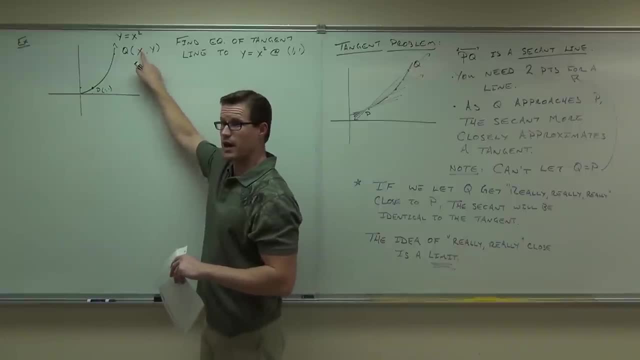 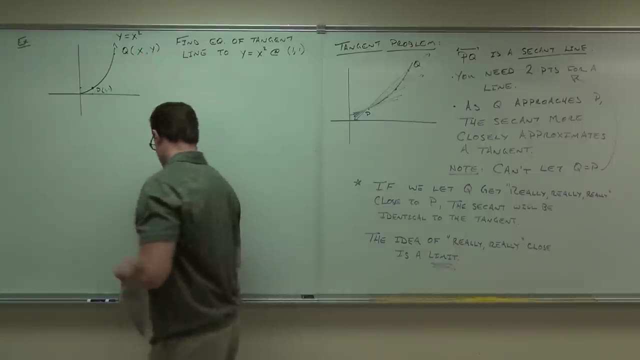 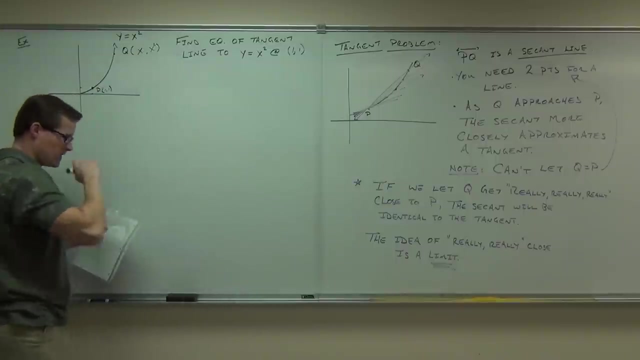 So, instead of having x comma y, would it be okay with you if I had x comma x squared? Yes, no, Because y is x squared, right, So that won't matter. So erase that, and I want you to put x squared. Cool, All right. 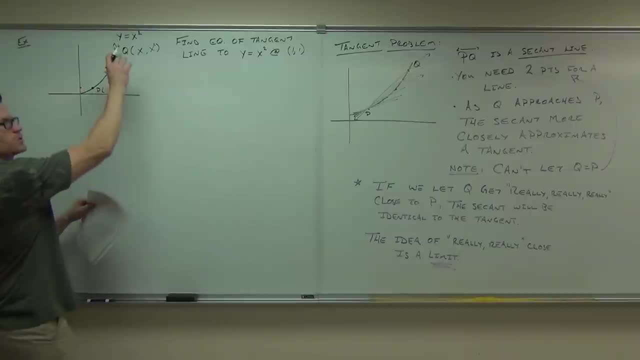 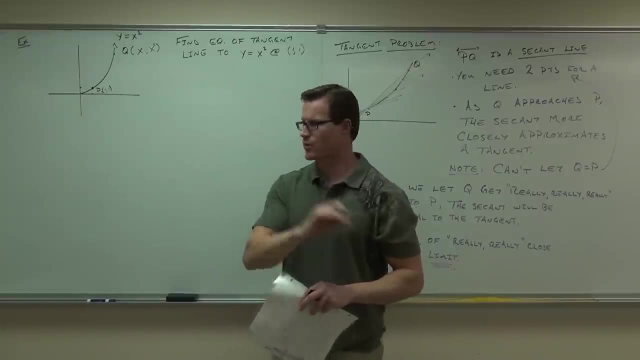 Now we have this secant line going from p to q. p is a fixed point, 1, 1.. q is a movable point: x, comma x squared. Would you agree that any point on this line will have the coordinates x, comma x squared, No matter what I plug in, right, So that movable point that's. 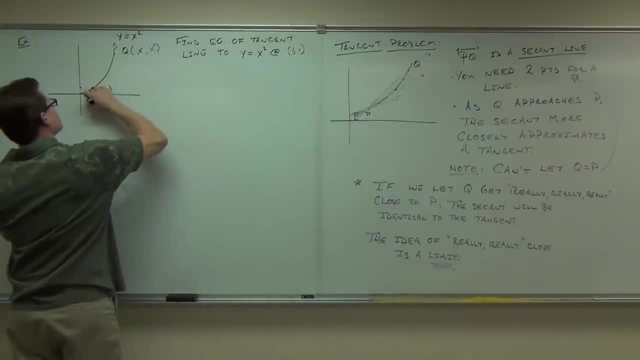 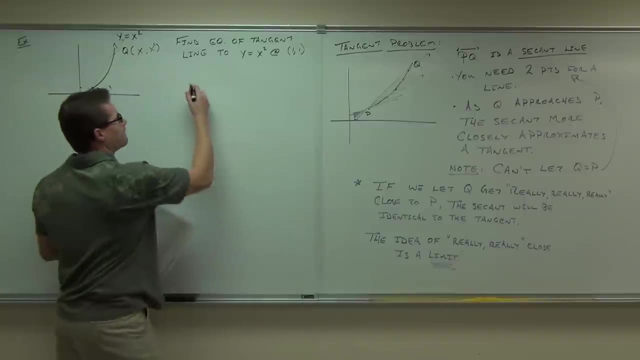 going to have the same coordinates all the way down. Okay, Now we have this secant line. Here's what we want to know. We know that the equation for a line is: y minus y1 equals m x minus x1, true? What we're trying to find is the. 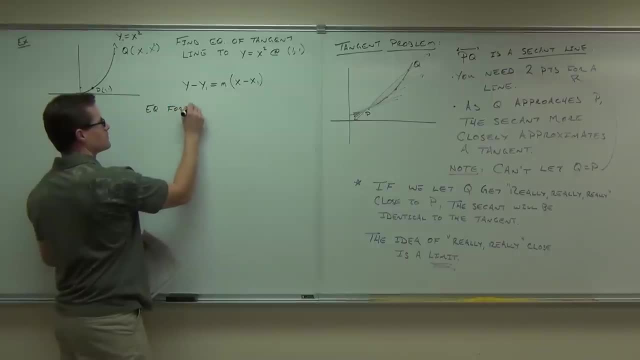 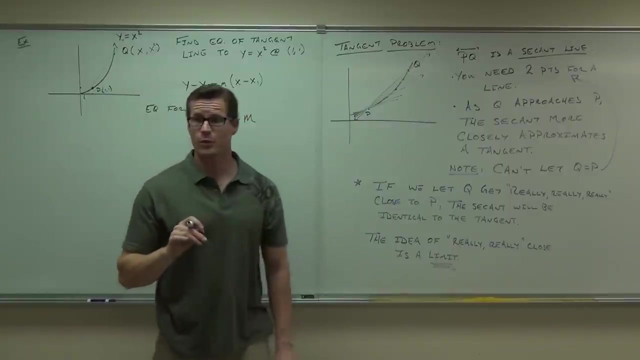 equation for a tangent line. Here's what the equation for a tangent line would be. Pay close attention. It would be y minus y1, that's the same. equals the slope, but a specific slope. It would be the slope of the tangent line. true, Whatever the tangent line slope happens to be, So the slope of. 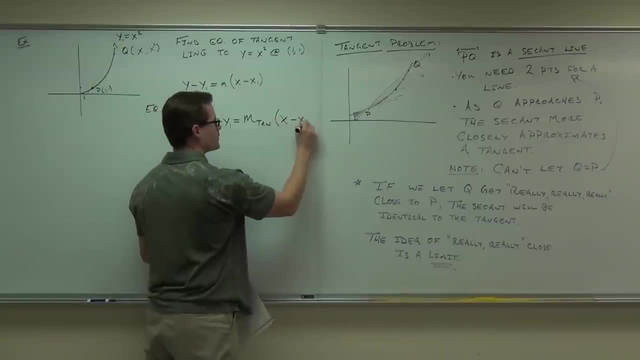 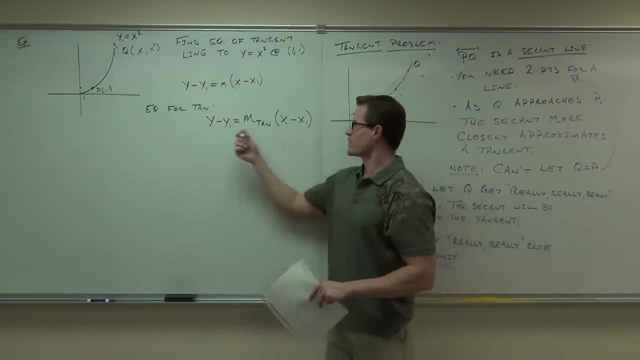 the tangent line and then x minus x1.. Now the cool part about this. I'll recap this in just a bit. The cool part about this is we already have a point. What's my fixed point? that I have 1, 1.. 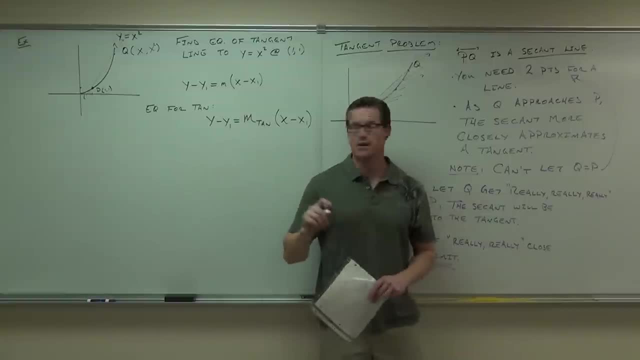 I already have 1, 1.. So really, what this comes down to is: can you find a fixed point? Can you find the slope of the tangent? That's why I said: find the slope of a curve at a point is the big deal for calculus. You already have the point, That's the easy part. The slope: 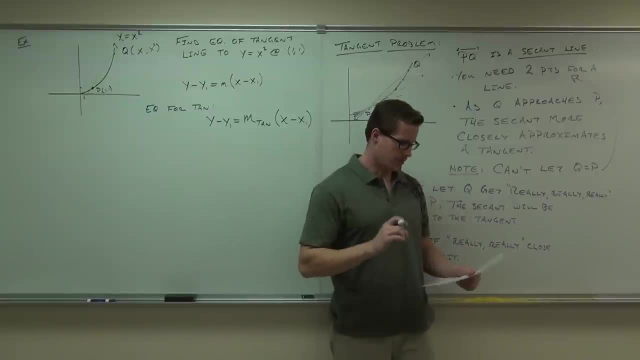 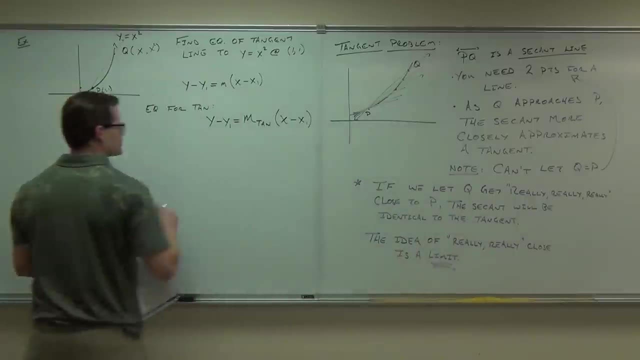 is the hard part. So we're going to try to find right now the slope of the tangent. Are you ready for it? Mm-hmm, Yeah, Are you sure? We're going to use the idea of slope of a secant, So we're going to take. 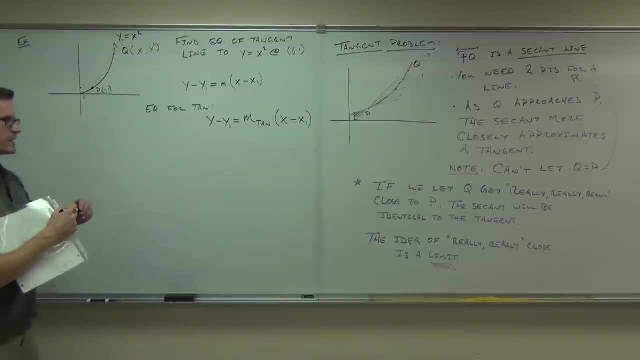 a break right now. We're going to come back to this. in case you're just a little bit lost, Here's what we've done so far. This is why, squared, I gave it to you. We fixed one point according to my problem. That's 1 minus x1.. That's 1 minus x1. That's 1 minus x1.. That's. 1 minus x2.. That's 1 minus x1.. That's 1 minus x2.. That's 1 minus x3.. That's 1 minus x4.. That's 1 minus x5.. That's 1 minus x6.. So we've fixed one point, according to my problem. 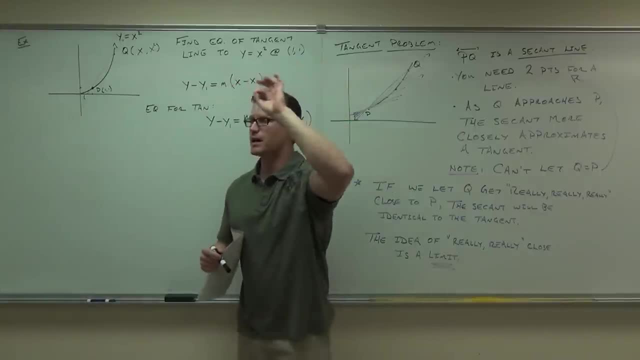 That's 1, 1.. We've made up another point, a movable point, q. q is at x comma, x squared. Where did the x squared come from? Y? That's because it's y. All right, Great, We now know that the equation of a line is: 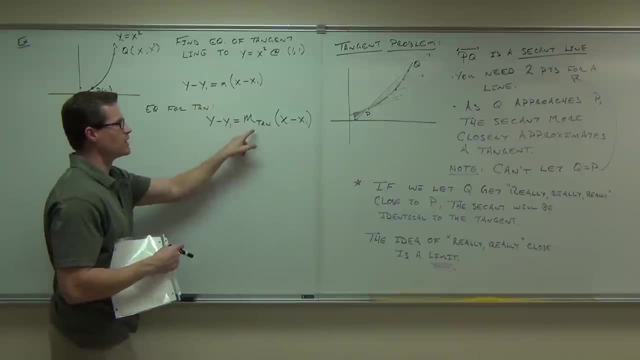 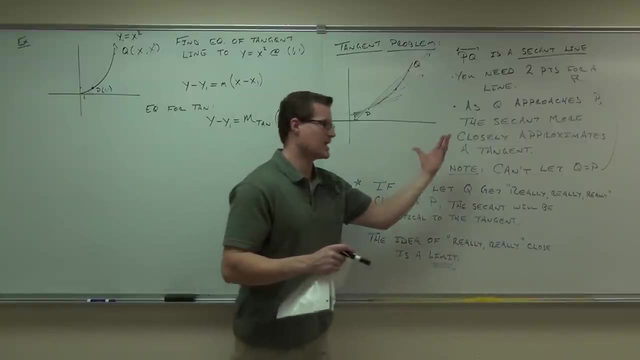 this. So therefore the equation of a tangent line would be the same exact equation, It's just we have the slope of the tangent line. The problem is, it's very hard to find the slope of the tangent line without doing the limiting idea. You can't do it because there's 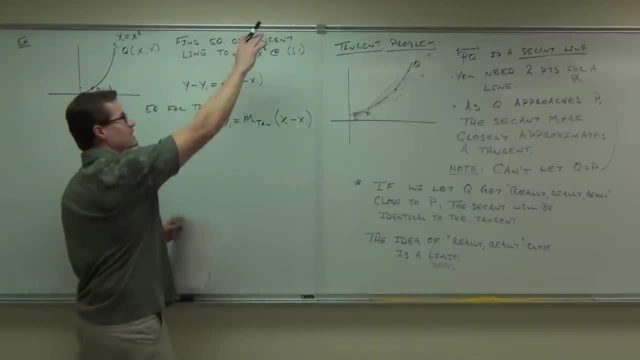 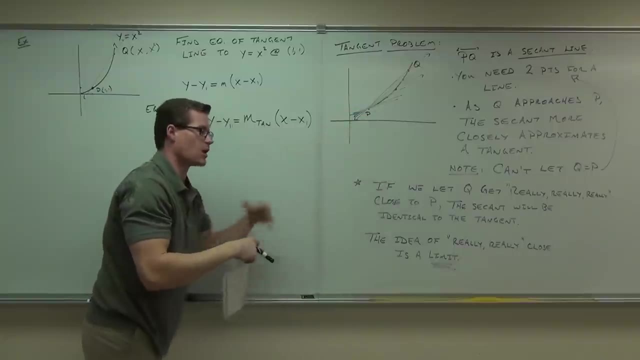 only one point there. So we're going to have to use the idea of a secant and make it into a tangent line by moving Q really close to P. Do you get the idea Basically doing that with this problem? So let's take a look at the slope of a secant, Our specific secant. 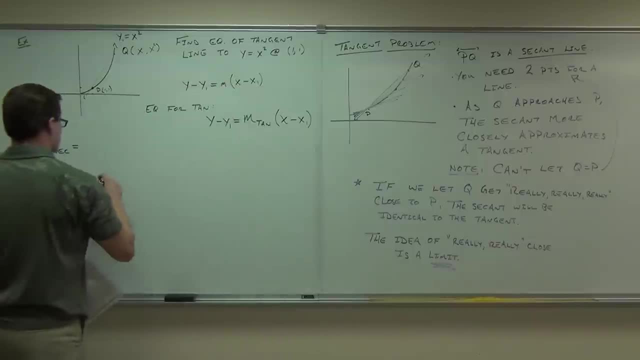 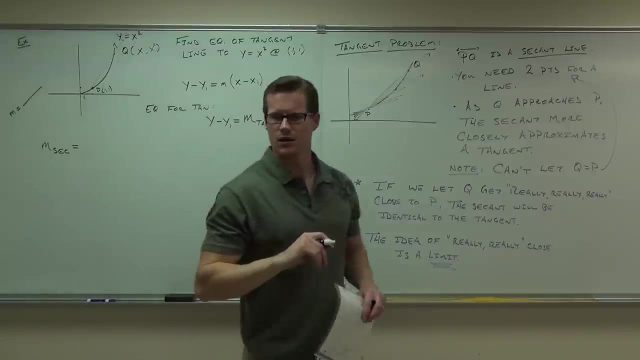 Hey, by the way, do you remember the slope in general, the slope formula? Slope is what over what? Right, Okay, great, In terms of our coordinates, slope is Delta Y over delta Y. Specifically, in terms of our coordinates, what is our slope? That's what I'm looking. 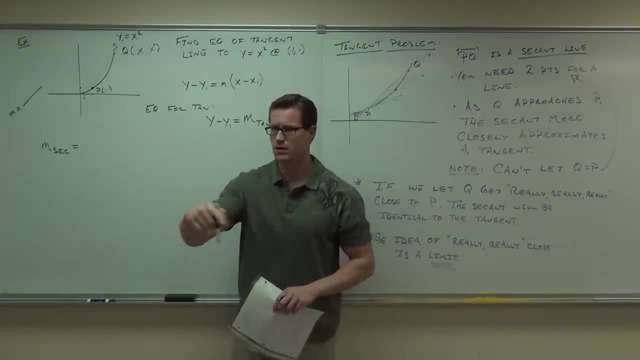 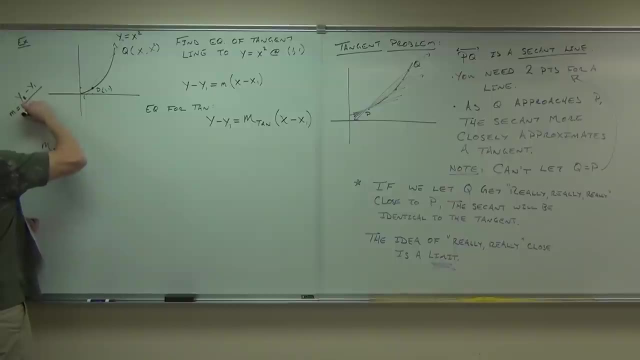 for Y2 minus Y1,, yeah, Over X2 minus X1, otherwise you get the negative of that slope. So Y2 minus Y1, X2 minus X1. Do you follow? How many of you feel okay with this so far? 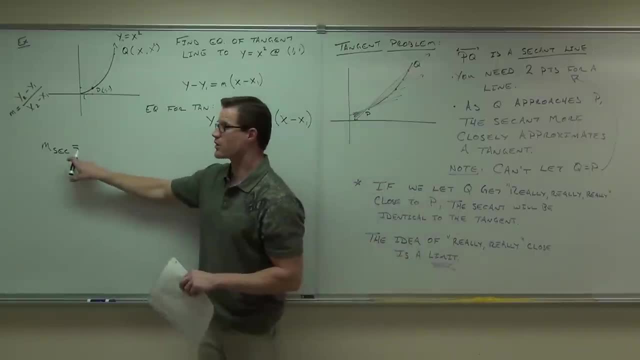 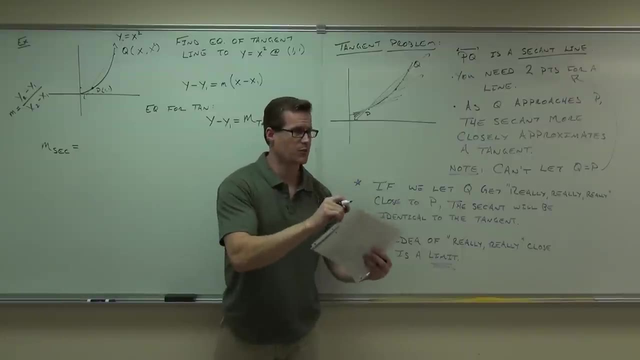 Just slope formula What we're going to do. we're now going to find the slope of our secant. We've got the secant on the board right. The secant will go down. We're going to find the slope. The secant will be. the slope of the secant will be the slope from points P. 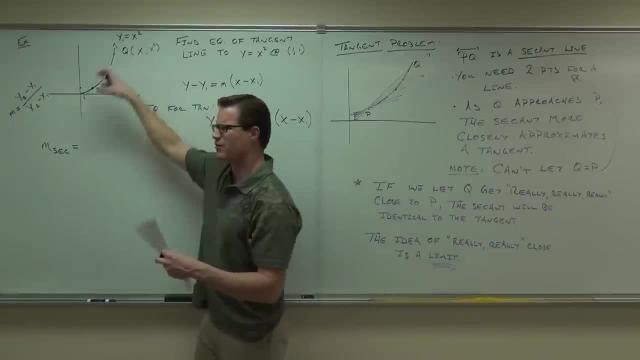 to Q. Agreed, Let's plug in these coordinates. We don't even have them on the board. Plug in these coordinates into that formula. In our case, our Y2 is what Our Y2 will be, X squared. What's our Y1? X, Not X. It would be 1.. What's our X2? X1.. What's our X1? X2.. 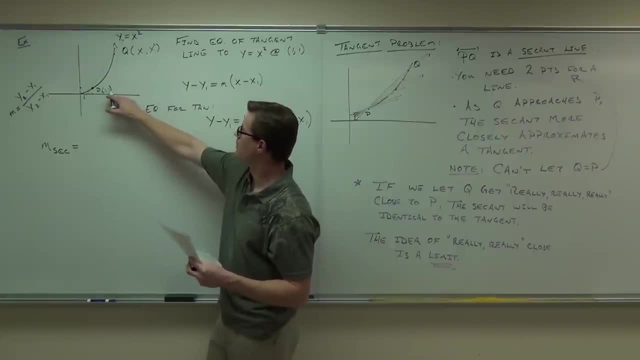 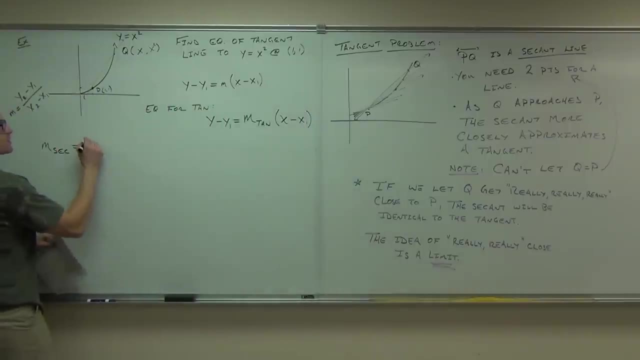 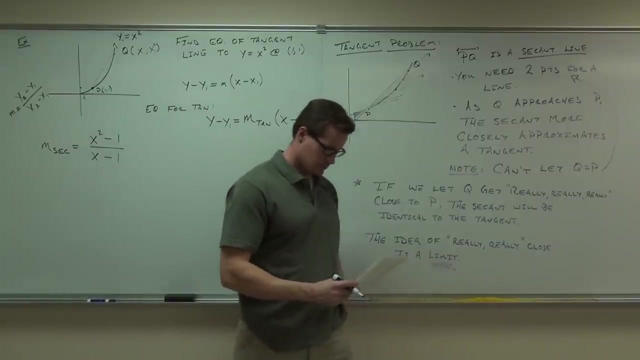 Okay, y2 minus y1 over x2 minus x1, not sure if you're okay with that. So what we have for the silver bar secant is y2 minus y1 over x2 minus x1.. Are you okay with this so far? 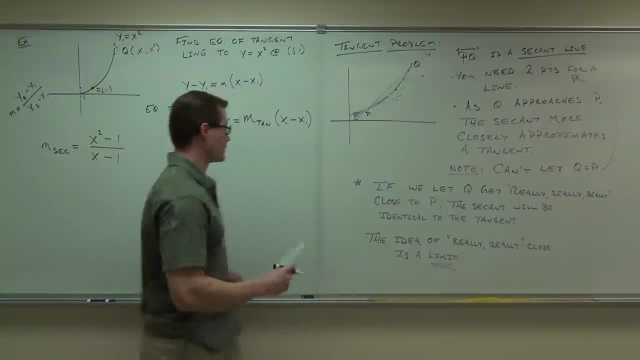 Find out where the slope comes from. There's a couple notes I want to make at this point. First, I'm reiterating a lot of stuff here. I know that I am. I'm doing it on purpose, because these are the key points of calculus. all right, 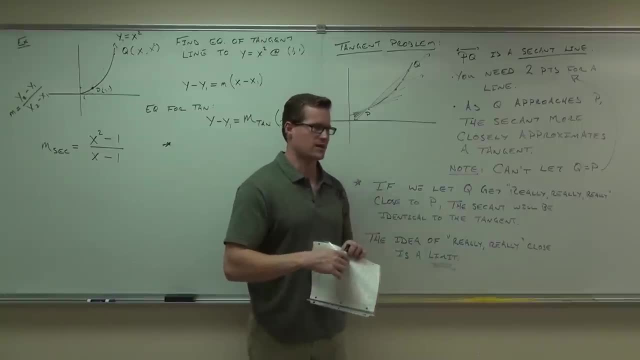 You need to understand what we're doing. I would hate for you to get through this class right and, at the end of it, know how to take derivatives and integrals and have no idea what you're doing. You can be successful on just doing derivatives and integrals in this classroom. 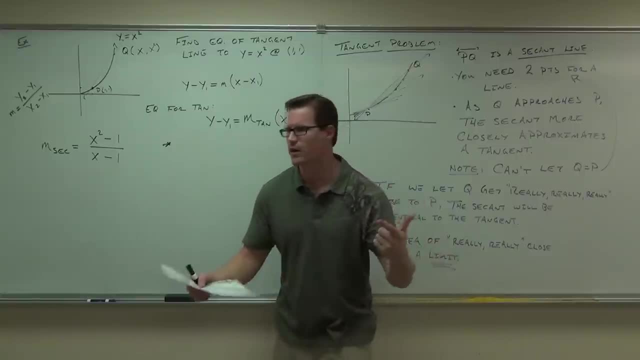 but if you don't understand what it is you're actually doing with those things, you don't even know what they are right now. But if you don't understand what you're doing, it's irrelevant. You're now just doing it. Formulas. it sucks. 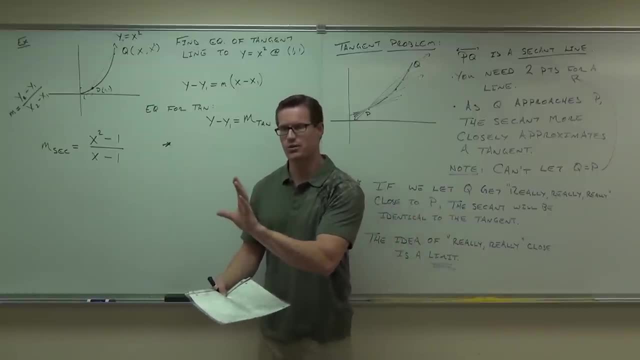 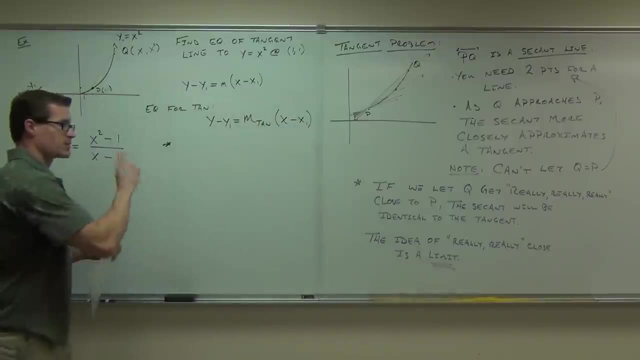 If you know what it comes from, what you're actually doing. I'm going to make sure you know. by the way, it's a little bit more interesting and you can apply it to more things. Do you get the picture So right here what we're doing? step number one is if we move q close to p, 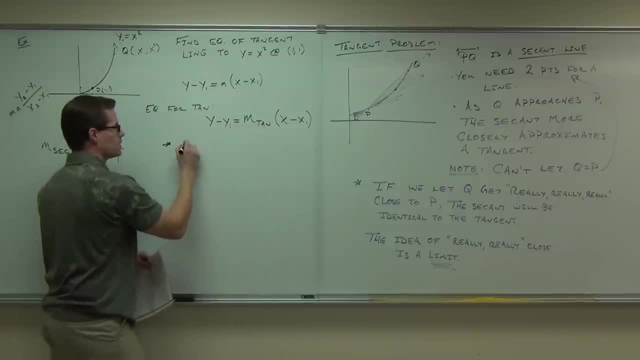 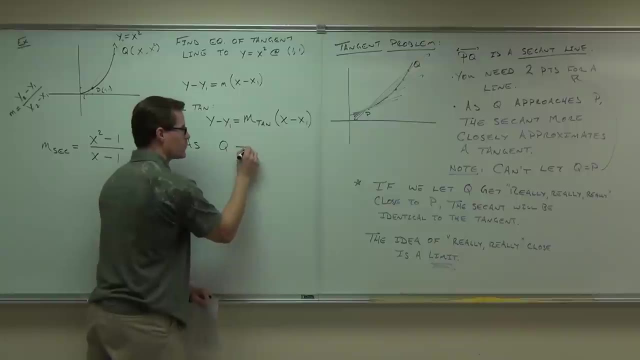 this is going to become this. Do you agree? As p- I'm sorry, as q, I'm going to use a new symbol here- approaches p, That's it. That's it. That means as q gets really close to p without touching. 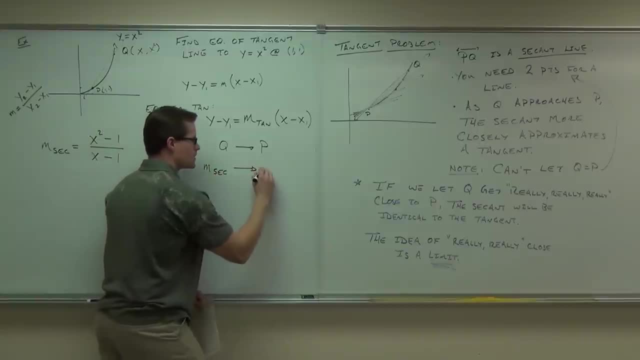 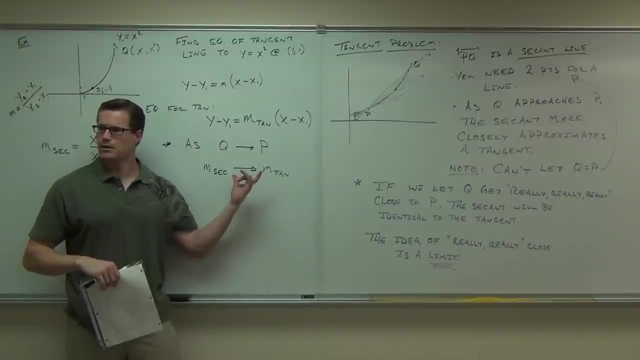 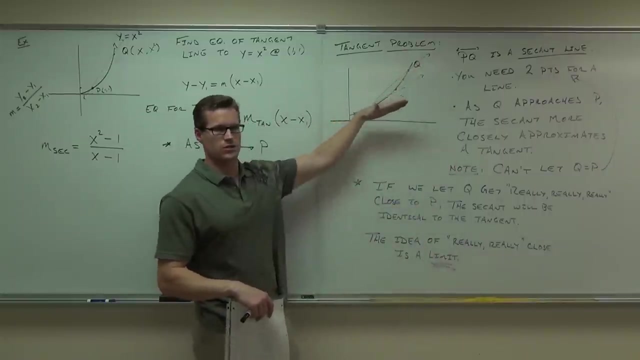 the slope of the secant line approaches the slope of the tangent line. Would you agree with that statement? That's over here right now. You agreed with it already. Ha-ha, I tricked you. As q gets close to p, the secant gets close to the tangent. 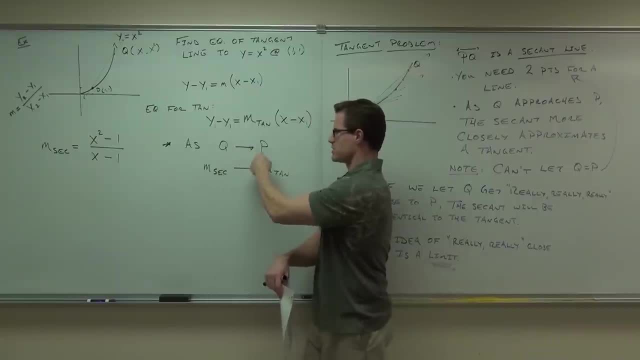 True, That's what this says right now. okay, As q gets close to p, the secant gets close to the tangent. How close, It depends on how close we get these things. Okay, If we get them so close, it doesn't matter. then these become so close, it doesn't matter. 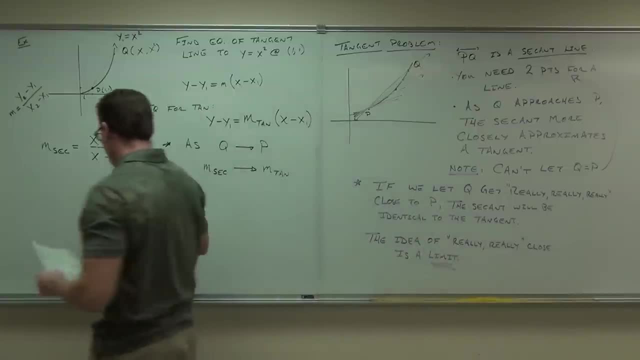 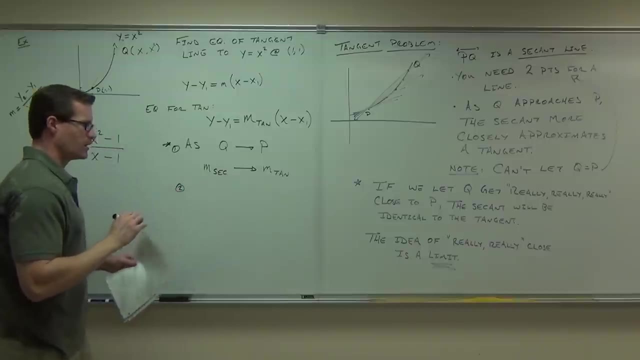 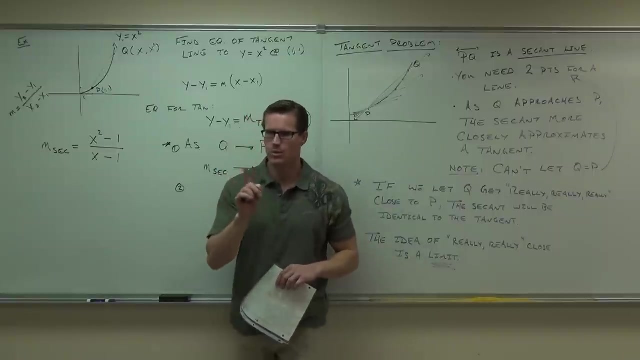 Agreed. It's kind of neat, right, It's a cool idea. Now the problem is: here's note number one. Here's note number two. This is interesting, right? Where are we trying to find the slope? What point. 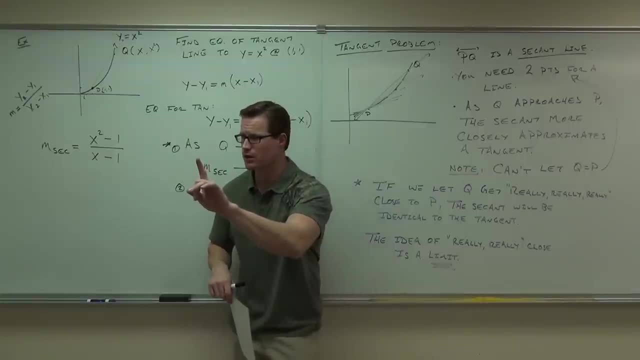 1, 1.. 1, 1.. And what's the x-coordinate of 1, 1? 1, 1.. To find the slope of anywhere you plug in that value. right, This gives you the slope of the secant line, true. 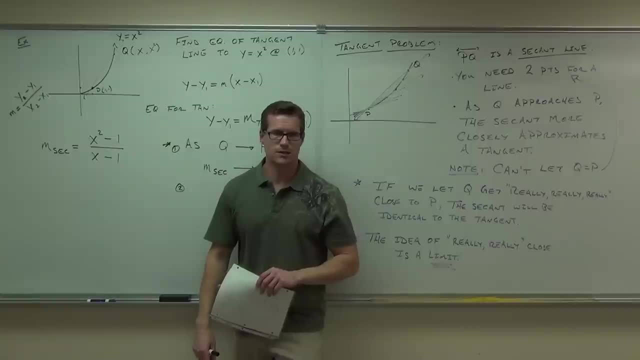 Plug in 1. Plug in 1. What happens? No, you don't get 0. You get 0 over 0 over 0 is not 0. That's a big problem. 0 over 0, 0 over 0 is undefined right. 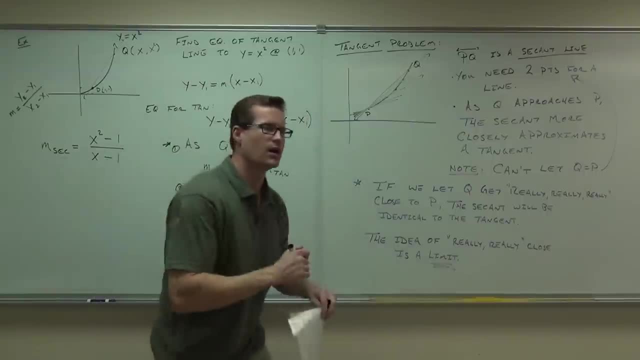 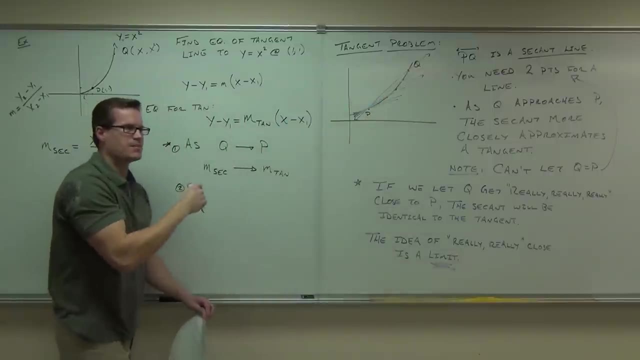 Isn't that an issue? This is why, folks, this is the reason why, why you cannot have have the point getting. listen, you can't get q close to p, because if you plug in 1, it's undefined. That means that you're you. you have the same point. 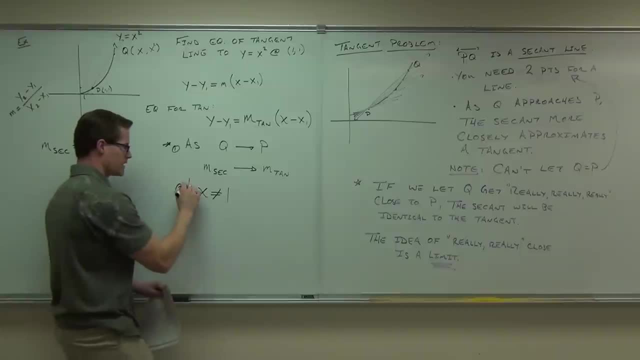 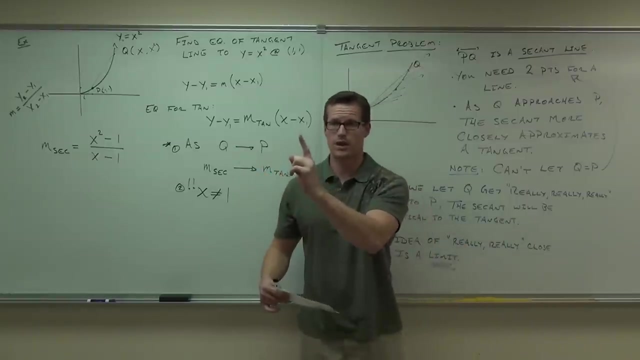 So you can't let x equals 1, that's big time. That means double important. You can't let x equal 1.. This is why we can't let q equal p, because we only have 1 point right. you can't find the slope. 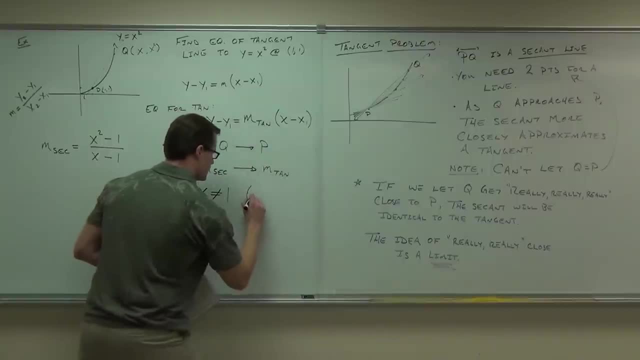 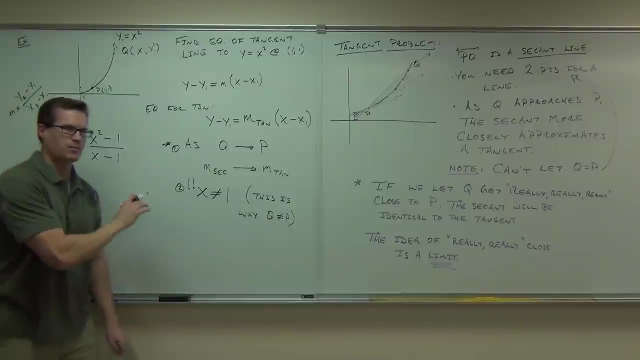 It fails, It's undefined at that point. This is why q can't equal p. If it does, if you try to find the slope of the secant at that point, move q all the way down and then plug in the x coordinate if it's the same thing. 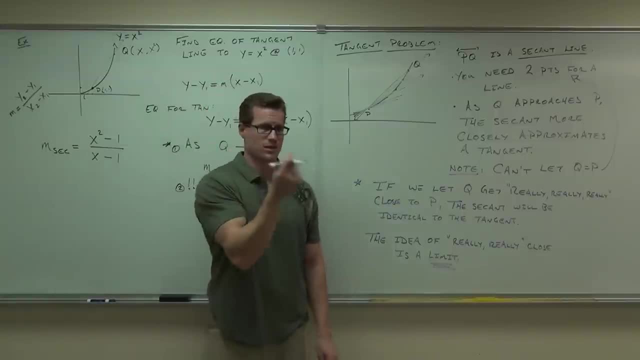 you're going to get something that's undefined, because you're trying to find the difference between points that don't exist, a difference that doesn't exist And that's going to be. you're divided by 0. There's no difference in the x axis. 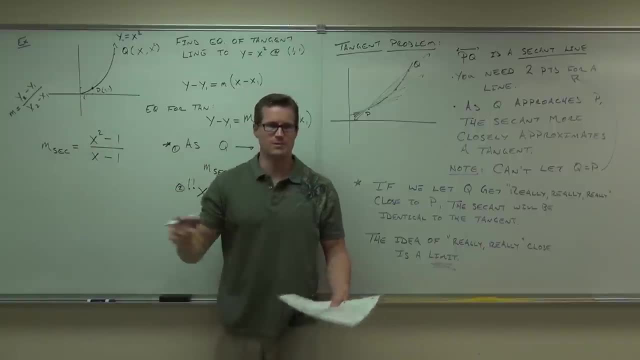 That would mean you're divided by 0.. You get something that's undefined. That would mean you're divided by 0.. You get something that's undefined. You get an undefined slope. That's a bad thing, So we can't let q get all the way to p True. 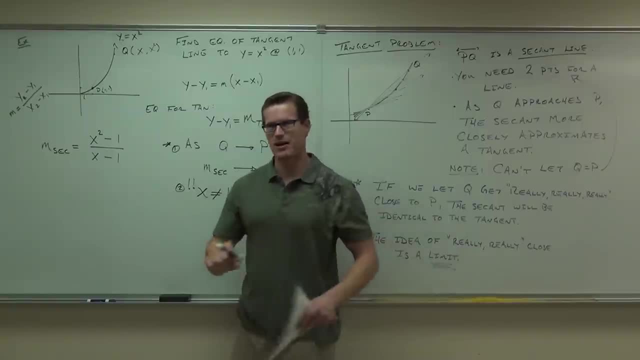 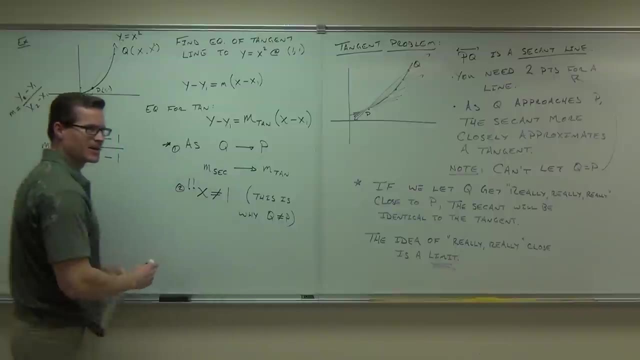 All right, What can we do Now? this is going to blow your mind. You ready to get your minds blown Like a mind grenade You ever seen Yes Man? Watch Yes Man, It's so funny- Had a ripple. You all have ripples. 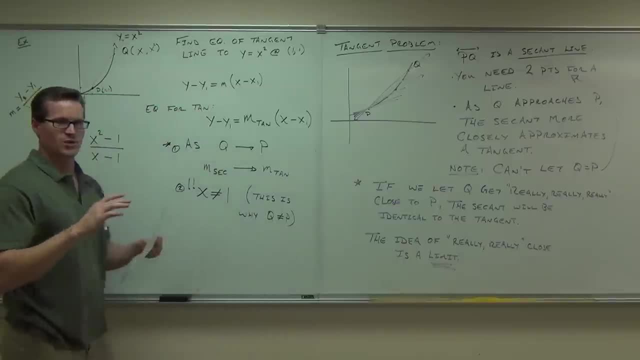 Let's go on a ripple Breath. Have you not seen it? that just sounded really stupid. You watch, Yes Man, It's pretty funny Now. so next part: It's going to blow your mind. Can you factor that? In fact learning what we knew about acid and stuff like that? 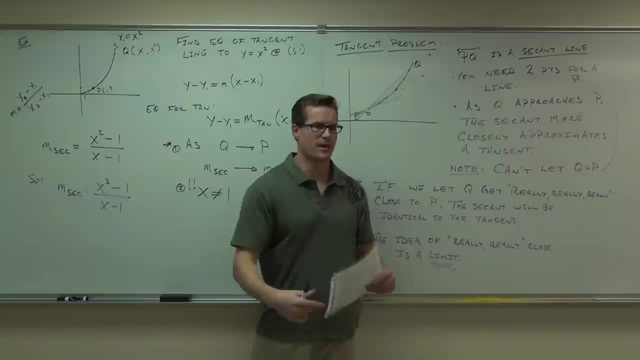 you know that if you have 0 over 0, it's factorable because of some stuff in mathematics that I haven't bored you with yet. But if you ever have some number that makes 0, it means that that's a factor. 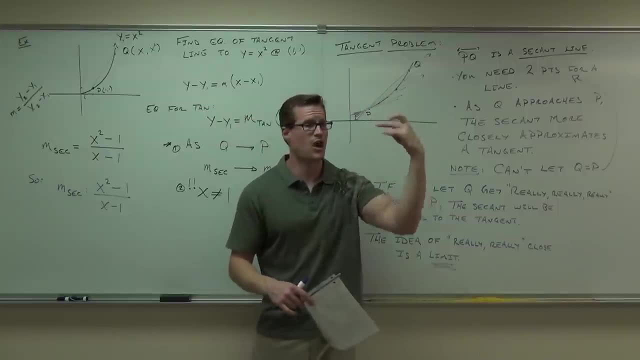 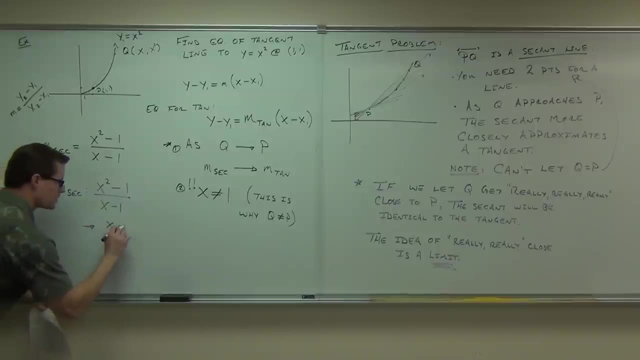 If you have some number, the same number, that makes 2 polynomials 0, it means they have a common factor. We've got a common factor here. In fact, if you were to factor this, this is going to give you x plus 1, x minus 1, over x minus 1.. 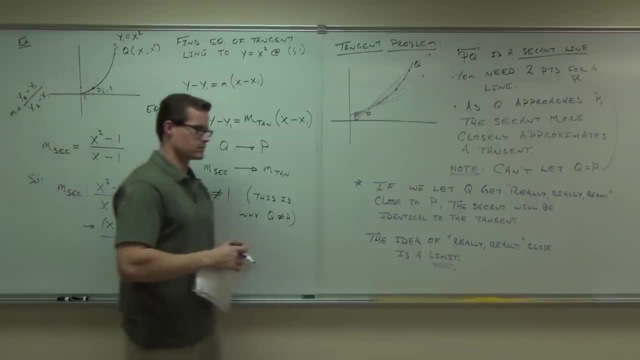 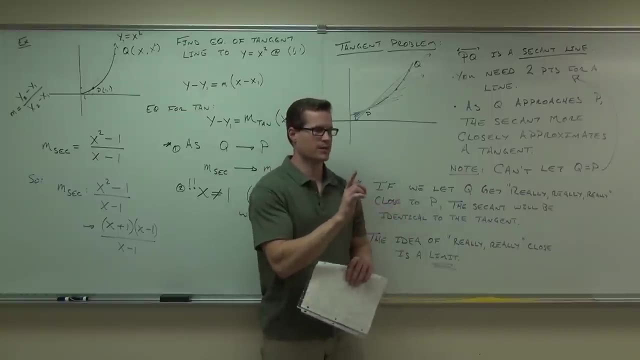 Agreed. Okay, Do you think see anything that simplifies out of that? Aha, Now this is cool. Now this is interesting, very interesting. What we're going to do is we're going to be able to simplify out this thing. 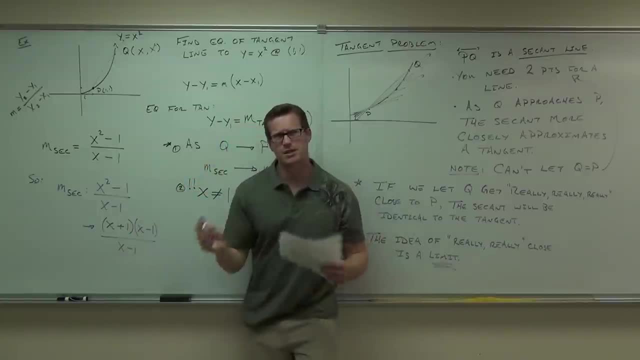 Now I know what you're thinking. Well, wait a second. Can't you not simplify out a domain issue? Isn't that a problem for you? And the answer is yes and no, It wouldn't be a problem normally. However, watch carefully. 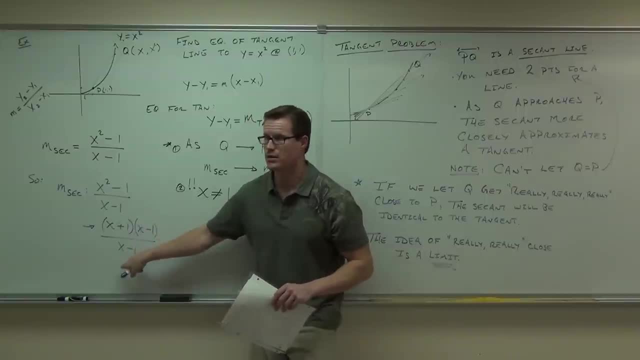 Are we actually letting x equal 1?? Is q actually getting to the point p? No, So is x actually equaling 1?? No, We're getting really, really close. I'm talking like 1.000000 forever, and then a little bitty 1. 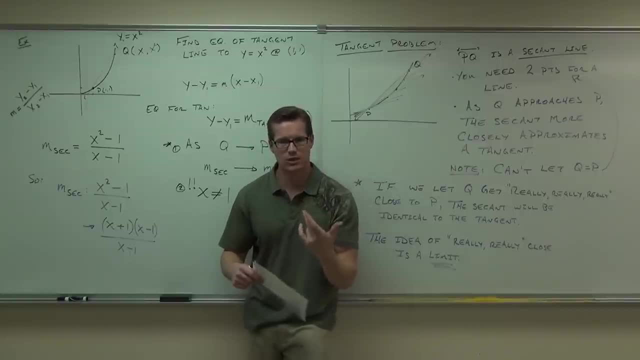 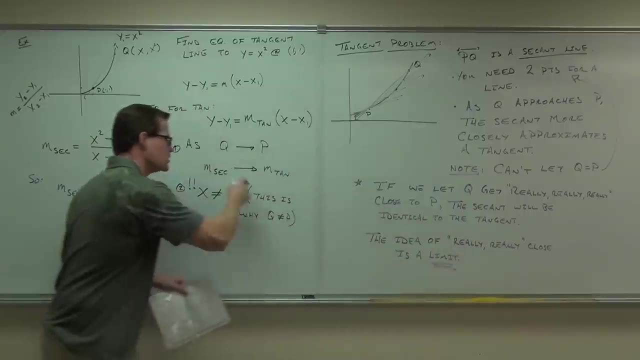 at the very end of it Really close, but it's never actually equaling 1.. So keep in mind, when we do this we're not getting rid of any, we're not really altering the domain whatsoever, because we already knew x wasn't equal to 1.. 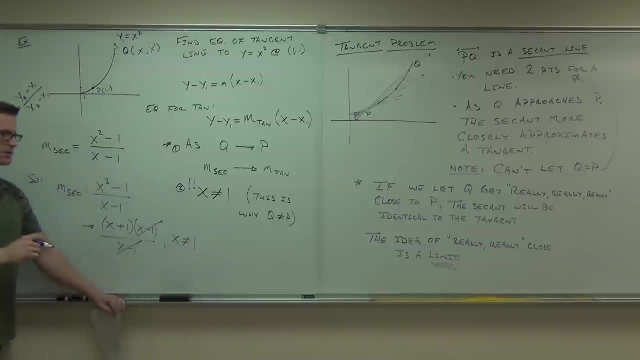 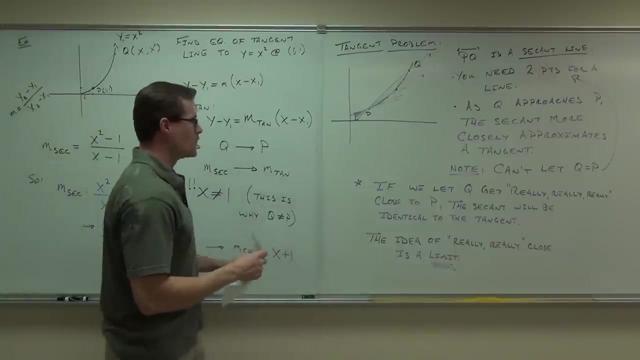 So we have this little restraint. Already, x isn't going to equal 1, so then what we know is okay: the slope of the secant now equals x plus 1.. Were there any questions on this? No, Okay, I'll keep looking at it. 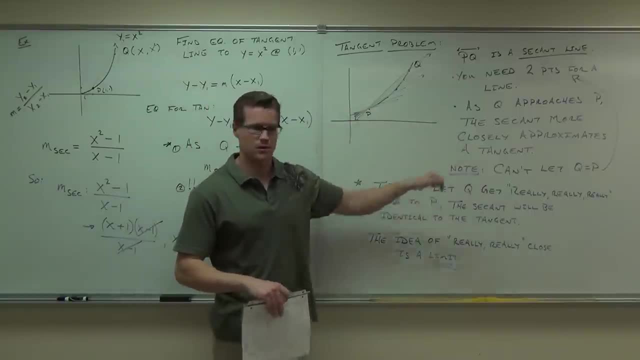 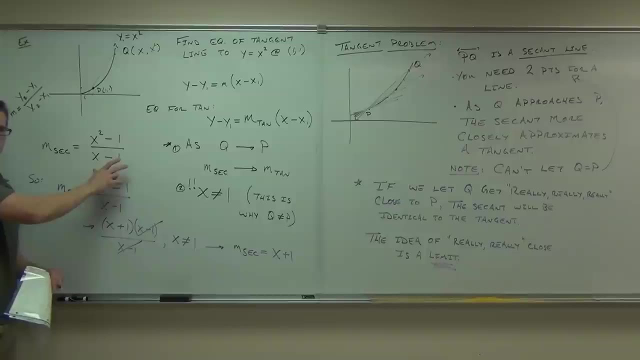 Okay, I'll keep looking at it. questions on this, because I've got to erase it. Do you have anything? Is this making sense to you? Do you see where the slope formula came from? Do you see how we can factor and simplify it? 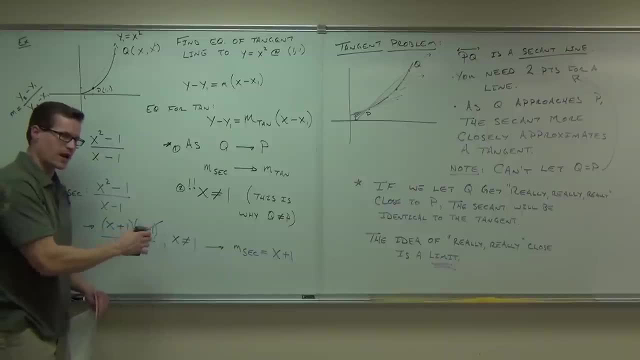 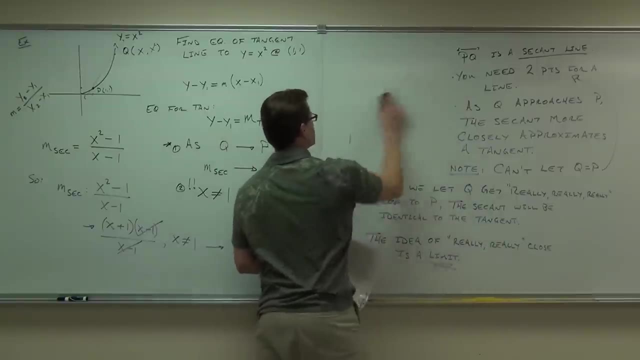 And now we get down to here. We don't have any problems. We're not eliminating a domain issue, because we're actually not letting x get equal to 1. It's just getting really close to it. Here's the jump that we're going to make. 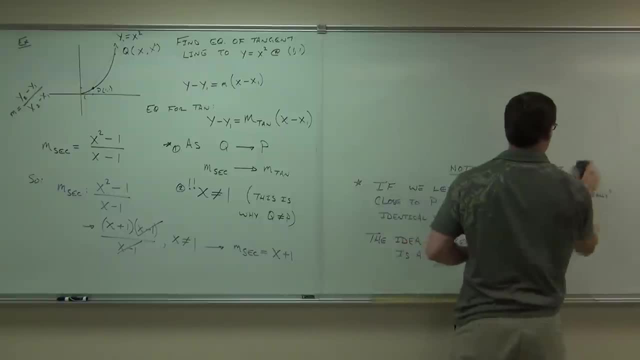 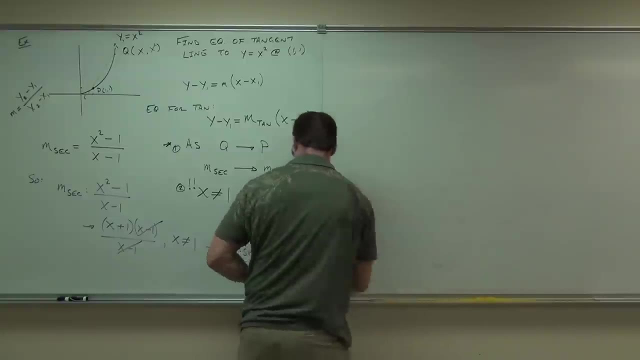 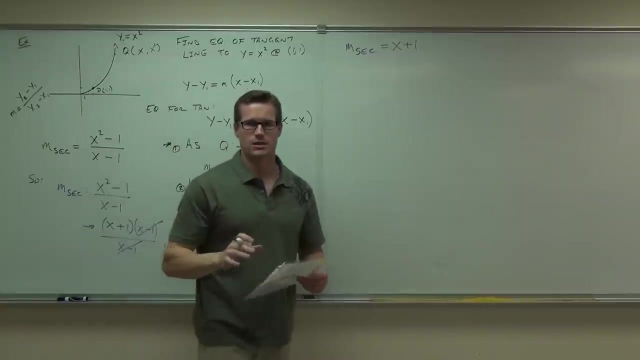 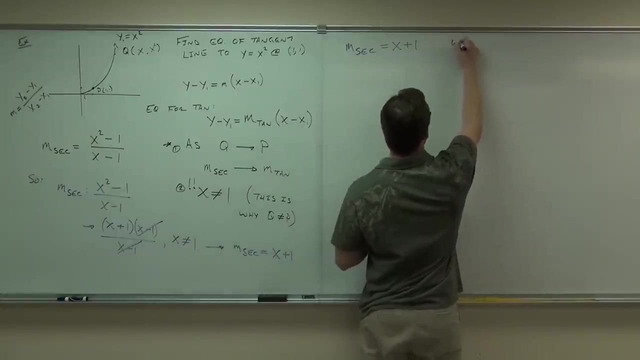 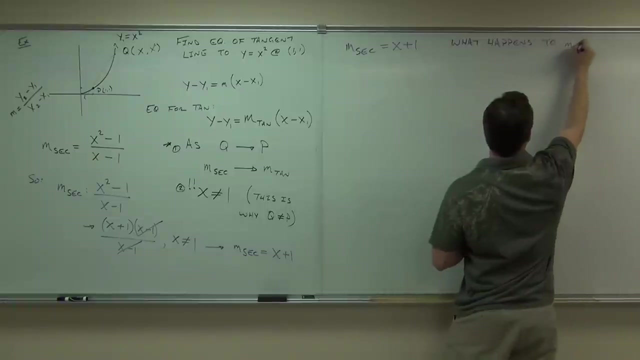 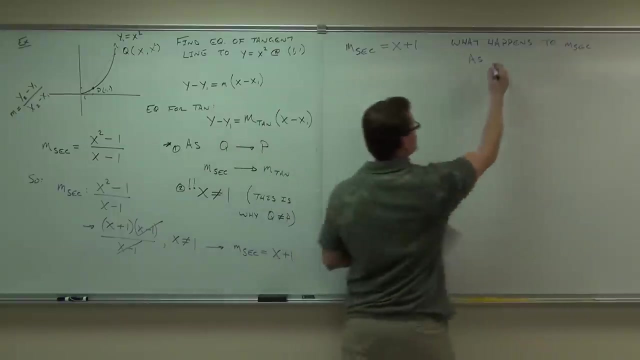 OK, Here's the jump. So that was true. That's what we have down. What I'm asking you is: as q gets closer to p, so basically as x gets closer to 1, what happens? As q gets closer to p, that means the x variable is getting closer to 1.. 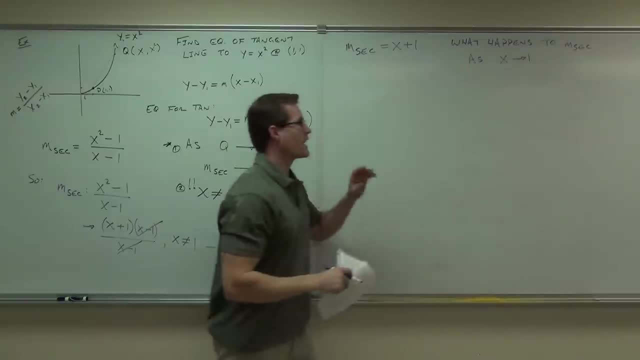 As x gets closer to 1, can you tell me what happens to the value of the secant? Let's try some. OK, Think about this for a second. Just do a little bit of math with me. Let's say we started at the point. 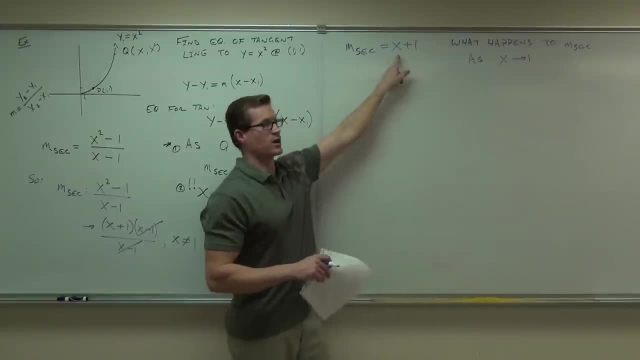 4, 16.. So x would now be 4. Plug in 4 here. How much would you get? 5. OK, Now let's move it down to 3. Plug in 3 here. What would you get? 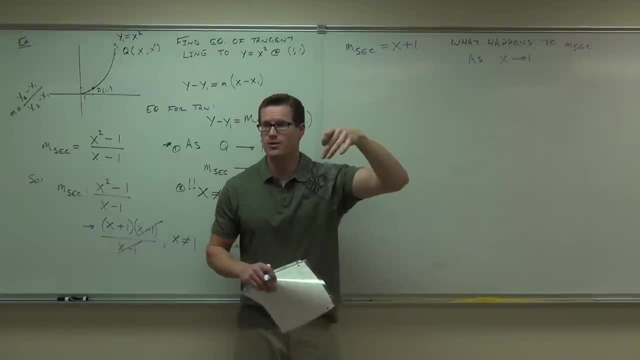 5.. Move it down to 2.. How much would you get? 3.. OK, Move it down to 1.5.. How much would you get? 2.5.. 2.5.. Move it down to 1.3.. 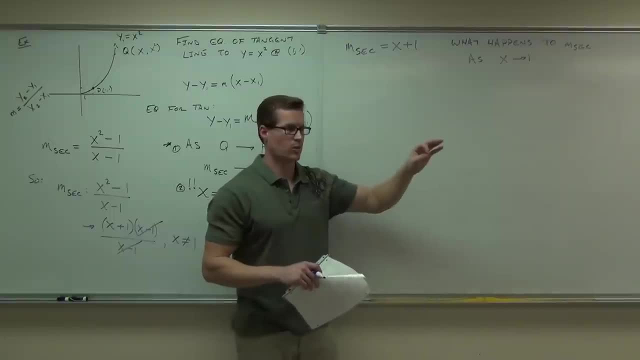 What would you get 2.5.. Move it down to 1.1.. What would you get 2.1.. Move it down to 1.01.. What would you get? 2.01.. 2.01.. 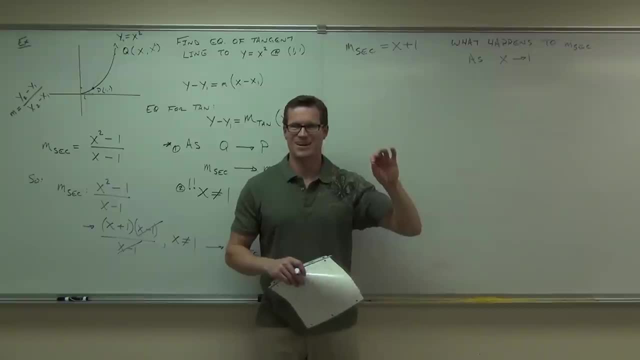 Good, Move it down to 1.00001.. Move it down to 1.000000 forever, and then a little 1 at the end. What would you get? 2.0.. 2.0 forever and a little 1.. 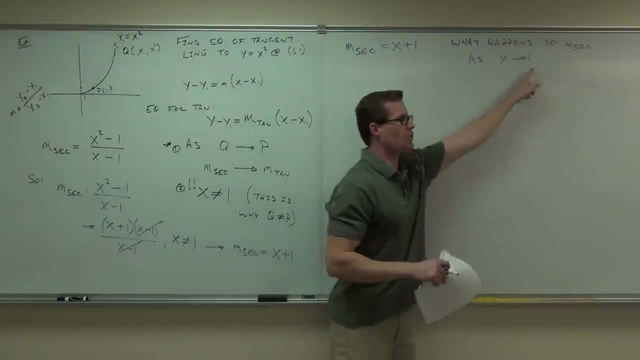 Would you? Would you say that as this thing gets closer to 1, the slope of our secant gets closer to 2?? Would you say that, Because I'm plugging in things really close to 1, I'm going to get out things that are? 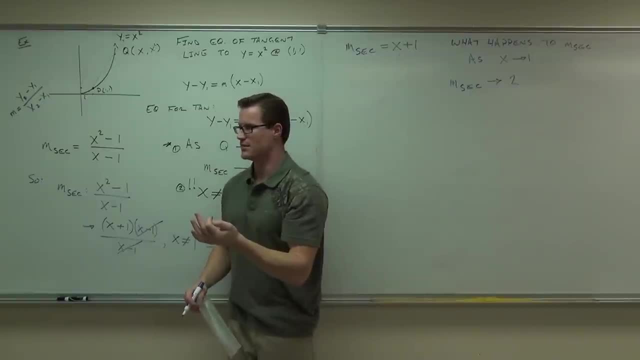 plus 1, really close to 2.. Does that make sense? Makes sense to you? Our secants should be really close to 2.. Here's what that says. This lets us make the jump. This is a limiting position. It says that we know the limit of the slope of the secant line is 2.. 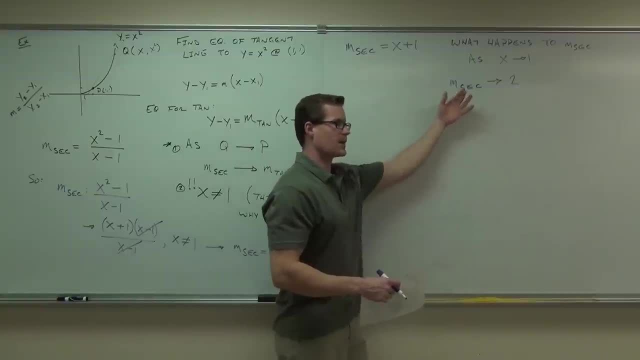 What that means for us is that the slope of the tangent line actually is 2.. That's the jump. It says the secant line at this point, if x gets super, super close, really really close, if x gets really really close to 1, the secant line is 2.. 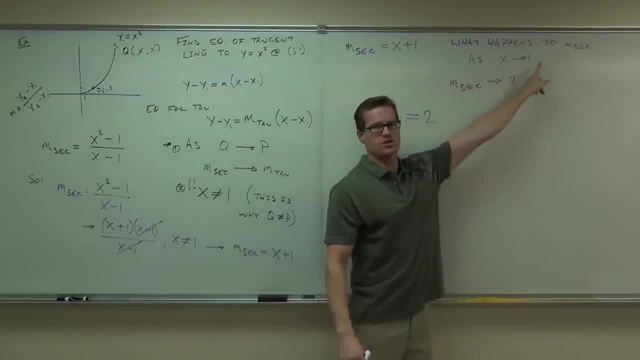 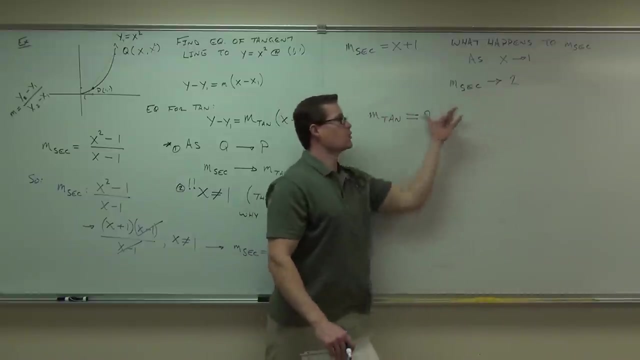 That's the jump. So we got 2.3.. Perfect, Thank you. the secant line gets really really close to 2.. Now I can't let x equal 1, but I can make the jump that if I could let x equal 1, the slope would be 2.. 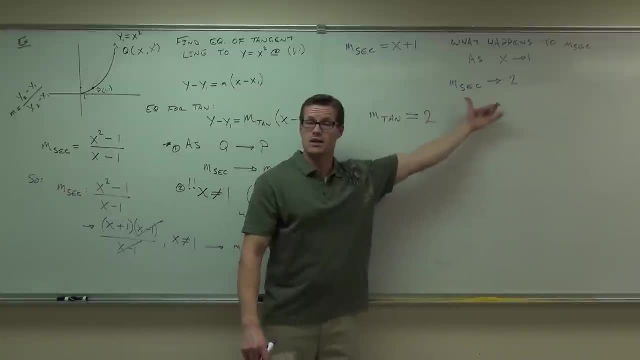 That's the jump there. Do you guys see the jump? This is using limits to make the jump between a secant and a tangent. So because the secant's approaching 2, we say, okay, we got this. That's called a limit. 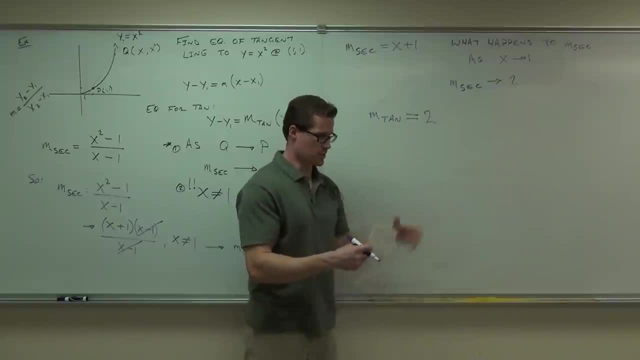 We're gonna talk more about limits later on, But the jump is going from here to here. Now can you fill out this equation using that information? Sure, we know that it would be y minus y1,, which is 1, equals the slope of the tangent. 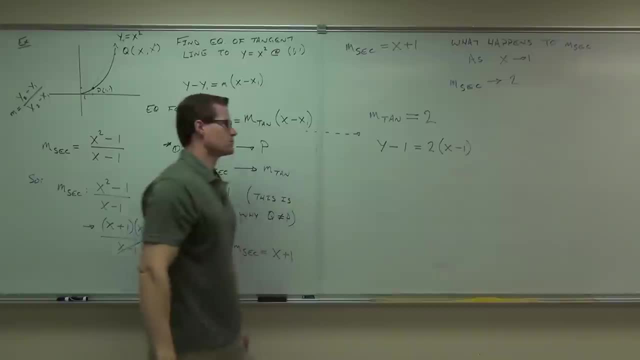 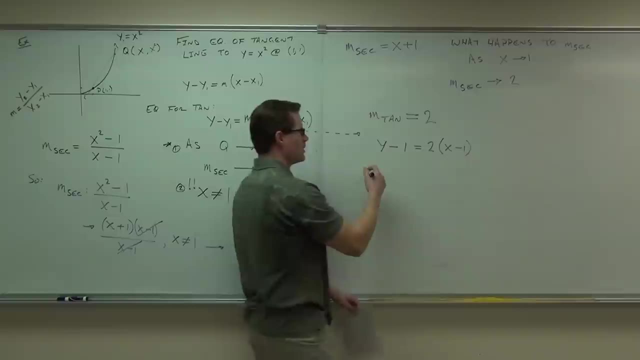 Hey, we know, it's 2x minus 1.. Now, of course, we don't generally leave things in point-slope, we'll solve them. Do you see where the 1,, the 1, and the 2 are coming from, folks? 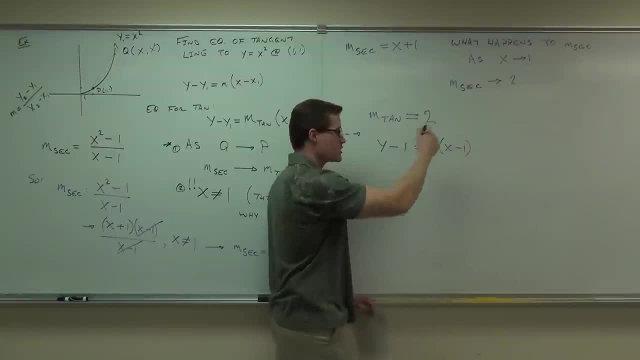 Our point is 1, 1.. Our slope is now 2, that's the slope of the tangent. If we solve it, we get y minus 1 equals 2x minus 1.. Add the 1, y equals 2x minus 1.. 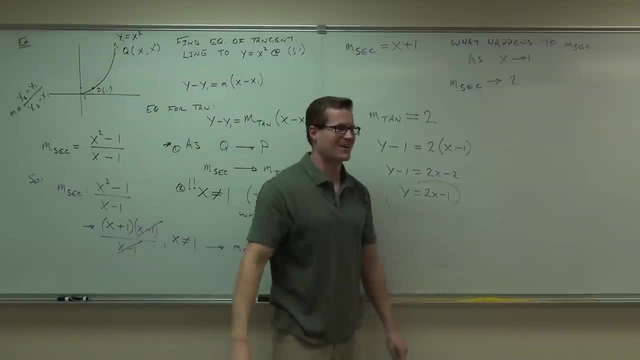 That's the slope of a curve at a freaking point. That's awesome. oh my gosh, isn't that cool. We just found the first tangent line to a curve that you've done. Now, granted, it's not a very hard curve. 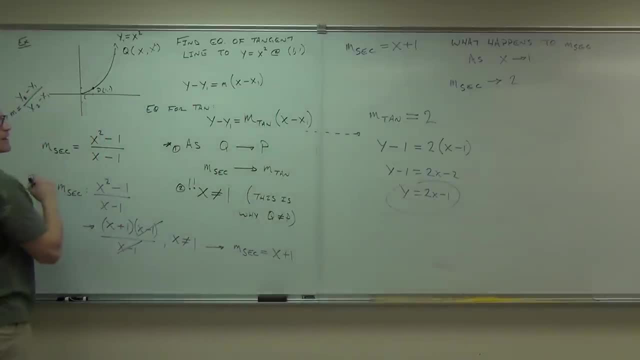 but here's what it is. I'll show it to you. You can actually graph it. Here's minus 1, it crosses there. You go up 2, 1, 2, over 1, oh, that's the point. 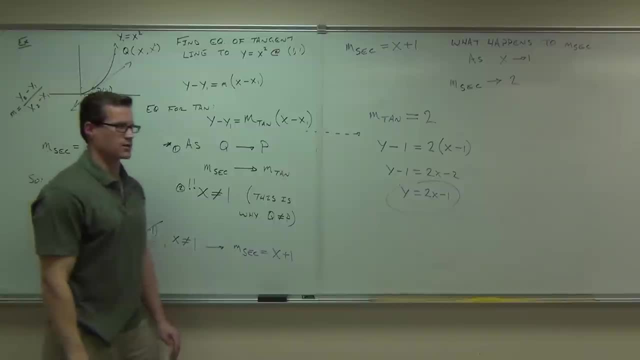 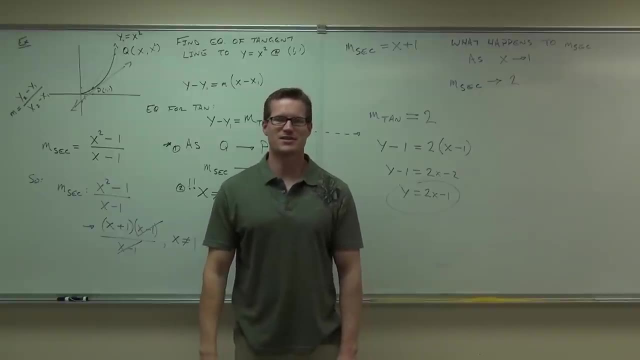 And if I graph it, it intersects at only one spot. That's it. that's a tangent line. Isn't that awesome? Your mind should be blown. Is that why you're looking at me stunned Like? is that your stunned face? 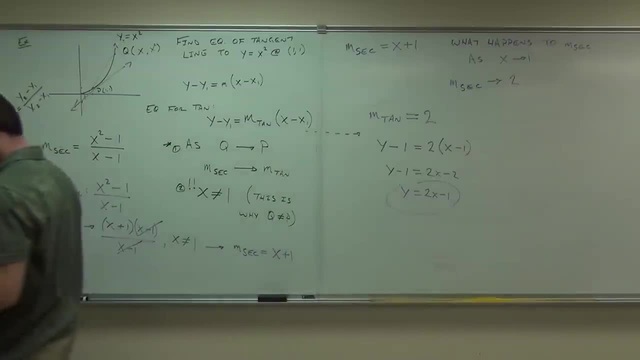 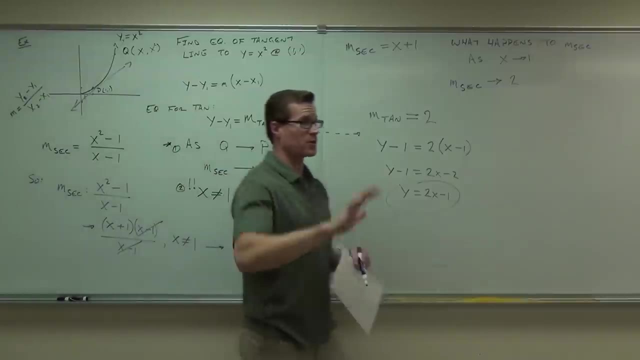 It should be your stunned face. Okay, Now by a show of hands. after 40 minutes of doing one example, how many people in this room have we talked about Good? Do you have down right now the basic idea for calculus? 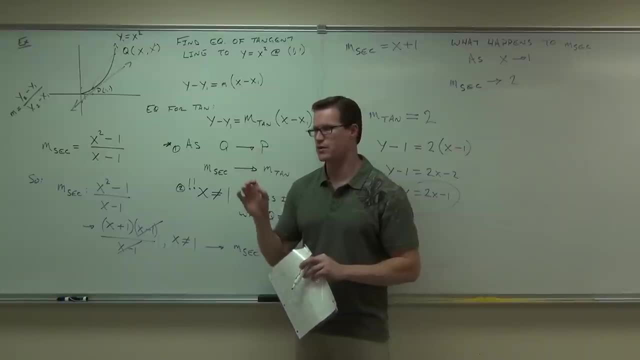 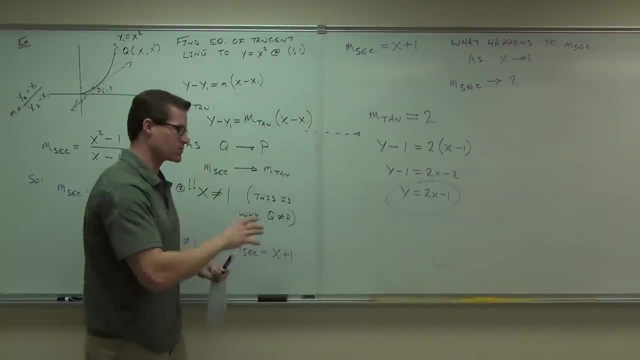 This is the basic idea: Using limits to find this tangent of a curve at a point. Is it gonna get more advanced than this? Yes, of course it is, but that's the basic idea And we're gonna do things differently when we actually get to the calculus. 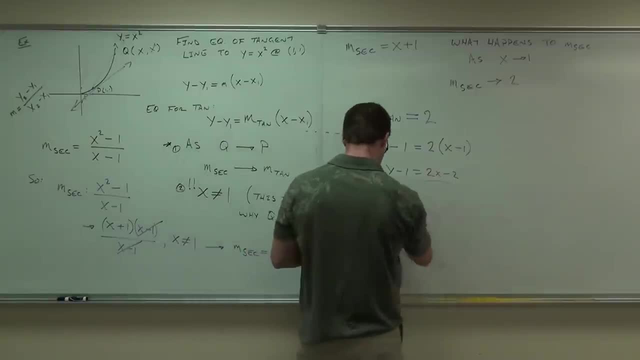 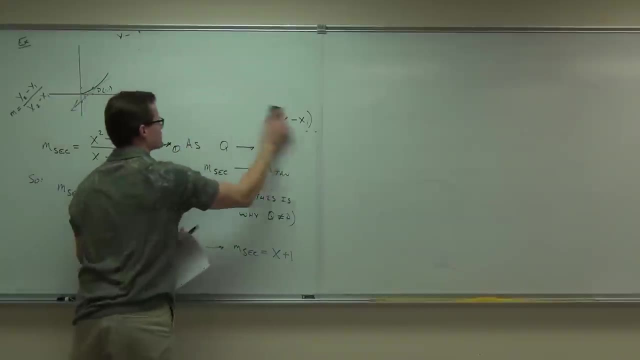 We study limits more first, but we will get there. Now, the next thing we gotta talk about is the different problem. I'm not gonna spend a whole lot of time on it. I'm basically just gonna introduce it to you, because I know for sure you guys are not gonna remember this. 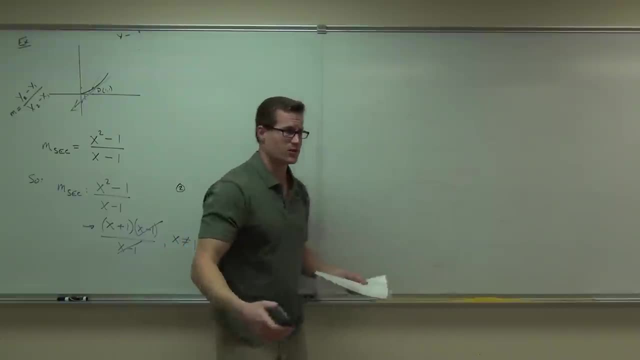 by the time we actually get to area under a curve. so I'm gonna reintroduce it to you again, But for right now I want you to just get the idea about what's gonna happen later on. Okay, so the area problem. 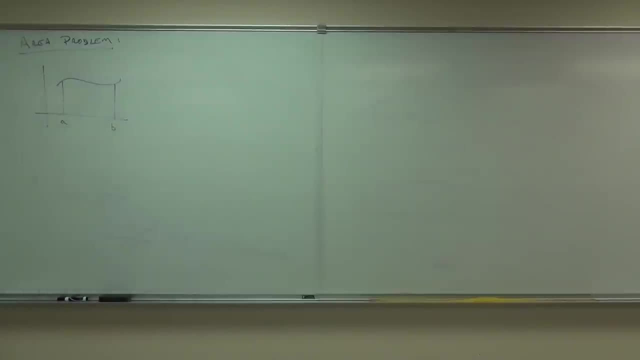 Here's the area problem. The area problem says: can you find the area under a curve between two points? Yes, you can with calculus. Only how are we supposed to do this thing? and let limits work for us. 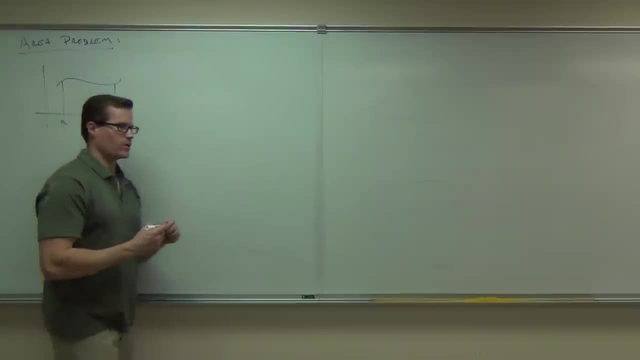 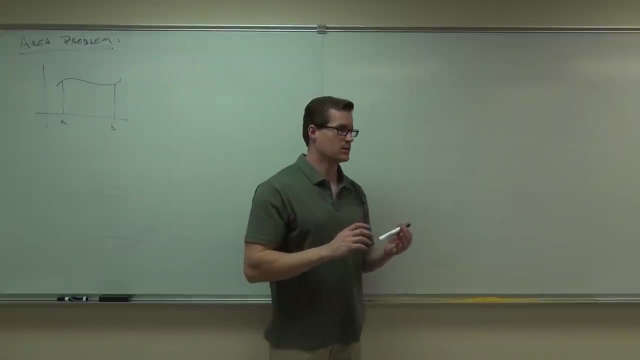 Here's the plan. Firstly, can you find the area the way it is right now? No, it's got a curve to it. You can't find areas with curves in them. So what maybe would be an idea You can approximate, if I'm making it like a rectangle, 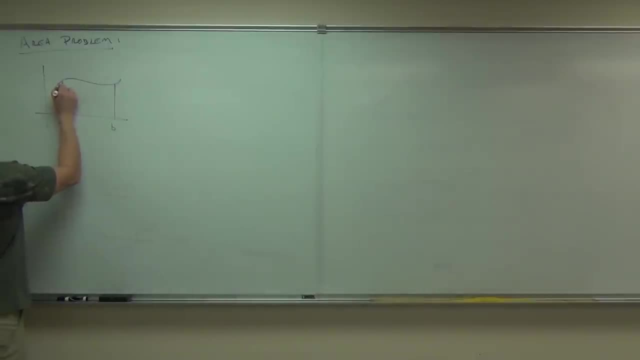 Oh, I could, Yeah, sure, If I did this and said: okay, a rectangle, would that be an approximation? would it be a good approximation? no, not really. however, what if i did: okay, i don't want just one rectangle, maybe i do this. i say: okay, i want a rectangle from 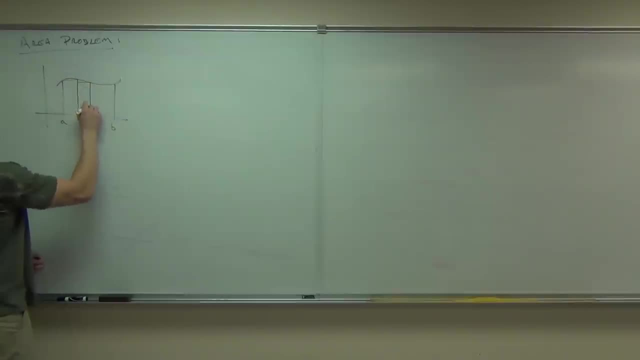 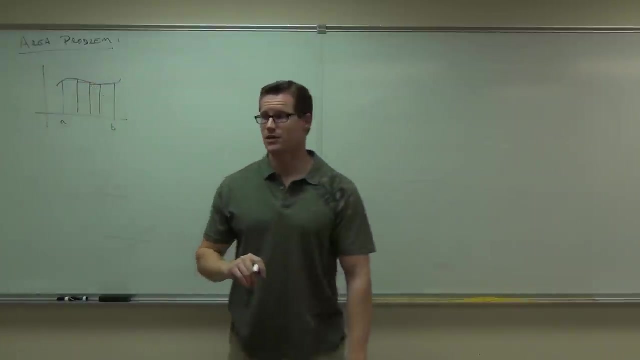 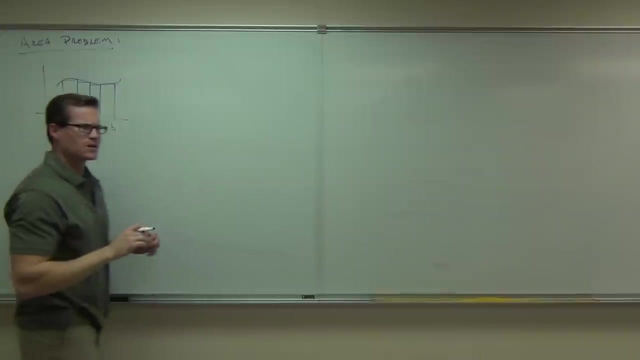 here to here, then a rectangle from here to here, then one from here to here and then one from here to here. is that a better approximation? the missing area is smaller. yes, that's the idea behind the area problem. what we're going to be doing is making rectangles. why rectangles? well, let me. 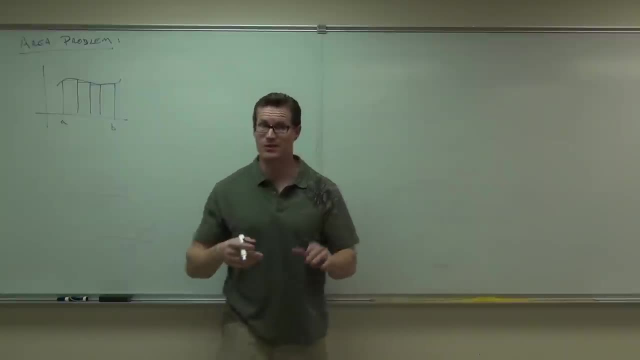 ask you, can you find the area of a rectangle? that's why rectangles and they're easy to draw. so if we make lots and lots and lots of little itty, teeny, bitty, weenie, little rectangles like that, all the same width but go in the entire length of our, our curve, and we add up all those rectangles, 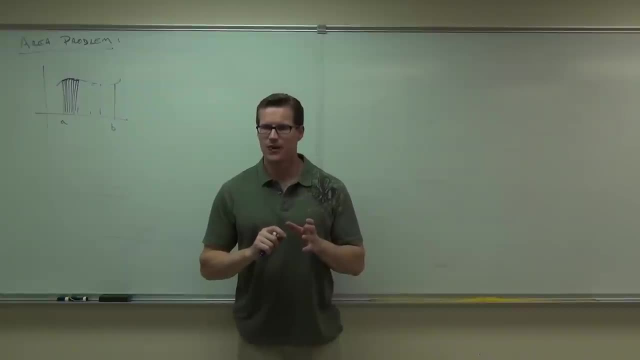 are we going to have a pretty good approximation of the area And, in fact, if we make those rectangles infinitesimally small, so whereas you couldn't even slip a piece of paper between them and then add them up, is that going to be even better? In fact, if we stuck an infinite number of rectangles? 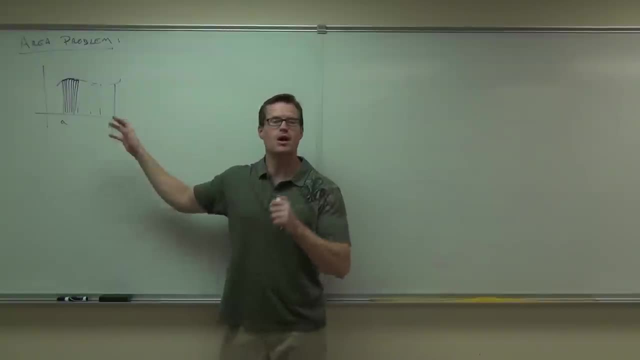 between this point and this point, which you can do with limits, we're going to have a perfect area, and that's the idea for the area problem. You stick an infinite number of rectangles in there and add them up. It's going to involve limits because we're letting 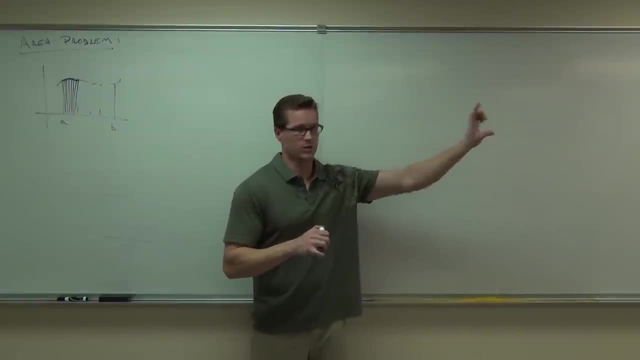 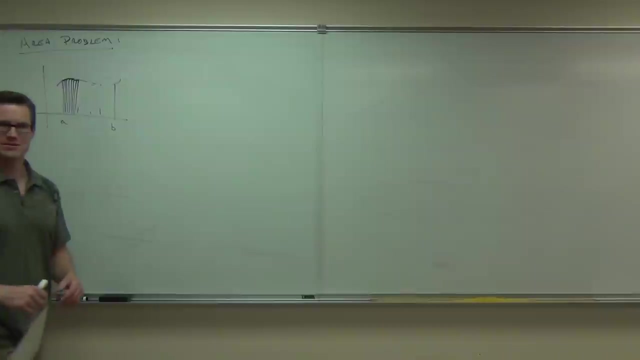 some number go to infinity. You can't ever reach infinity, but a limit will take care of that for you. That's the idea behind the area problem. Does it make sense? Kind of The idea of the rectangles? Trust me, we'll get much more involved later. You have no. 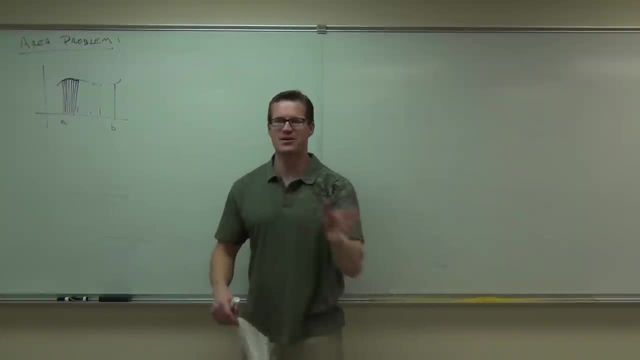 idea how to do this right now. Don't worry about it. okay, We're not even going to do a problem. We'll do that later in chapter four or something like that. So let's define a limit. What a limit says in English is: what does the function do as a variable approaches? 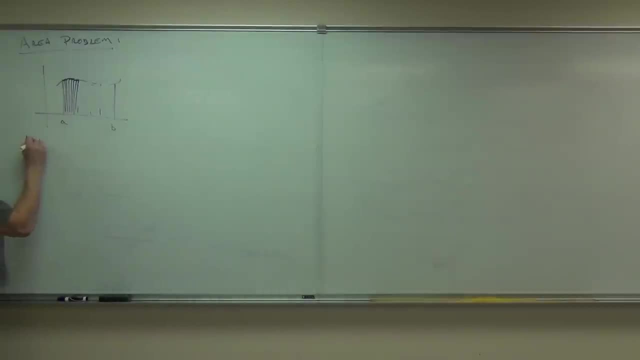 a given value? That's what it says in English. So limits. What does the function do as the variable approaches a given value? Yeah, Okay, Okay, That's the question. Now do we care what happens to the function at that value? 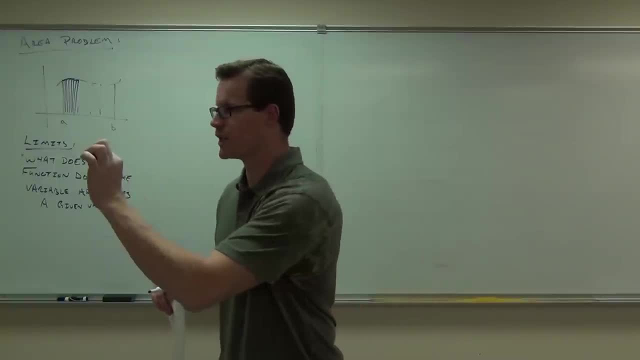 The answer is no. The limit isn't about getting to the actual point, It's about what happens as you're approaching that point, getting really, really close. You see the difference there. In the previous example, we couldn't actually get to 1.. 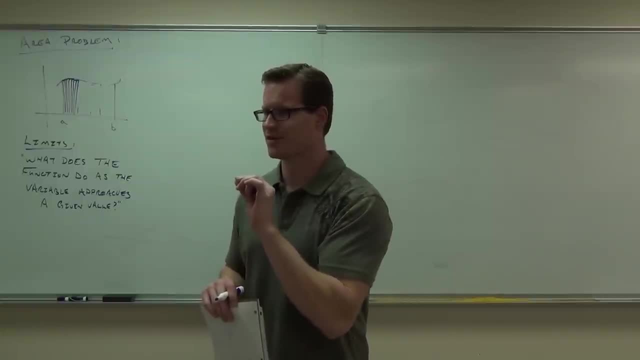 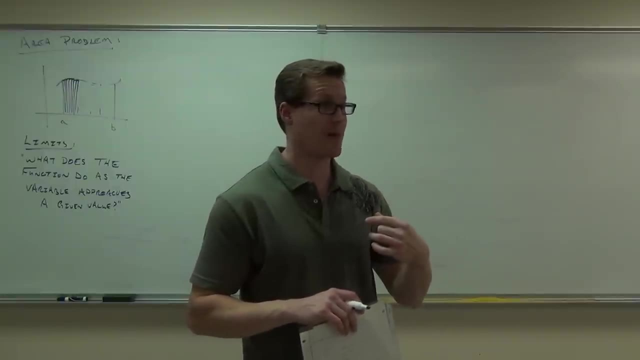 Do you remember why Some of you were zoning? You're zoning out. You can't have one point on the line. We'd also make an undefined point, right, If you undefined that, it would be that. But we saw what happens when we get really close. 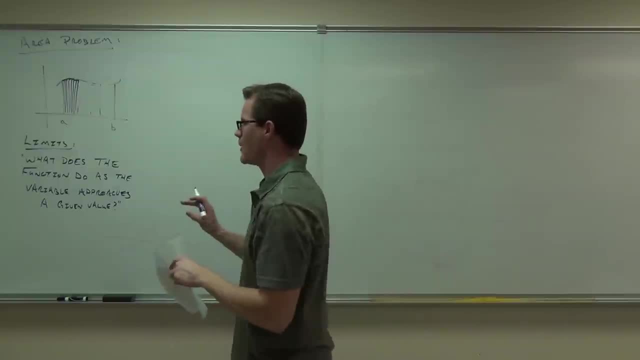 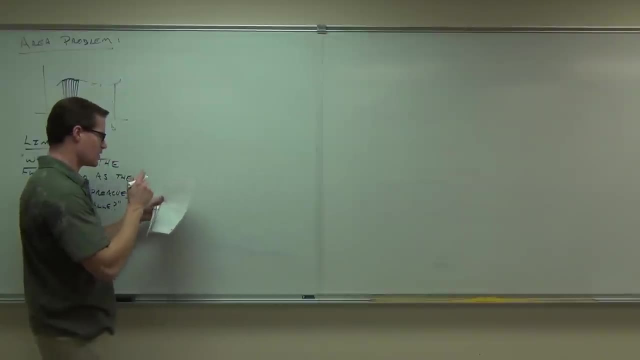 The function got really close to something else. That's the idea of a limit. So we don't care what happens as you get to the value, What happens as you approach the value. For us, this is exactly what we did actually kind of in our heads. 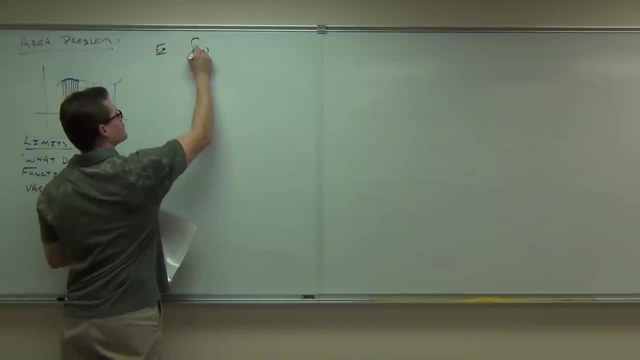 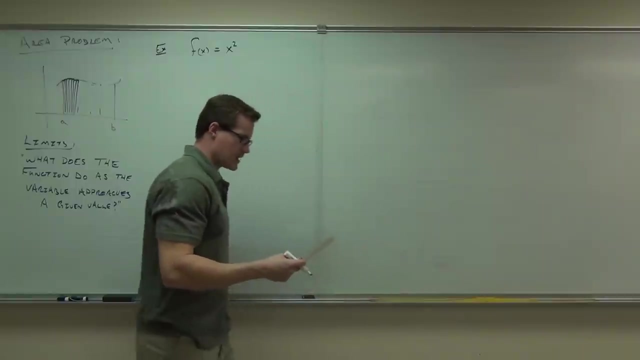 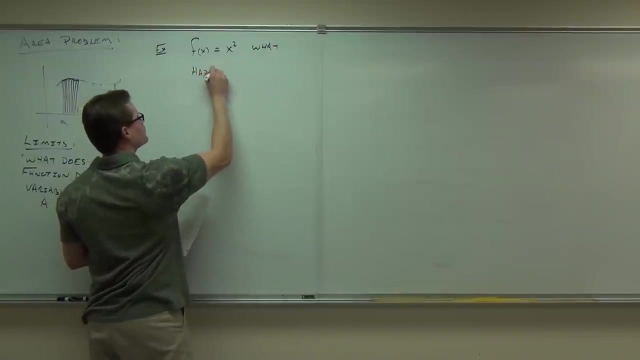 What happens? What happens to x squared? As x approaches, let's do 2.. That's x approaches 2.. I could have written it in English, but that's just as valid. What happens as x approaches 2?? Now, do we care what happens if you plug in 2?? 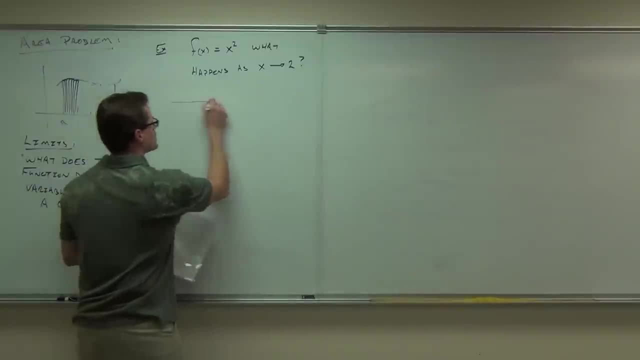 No, we don't care. What I care about is x approaches 2.. What I care about is what's going to happen if I draw this table right here with x and f of x And I say I'm trying to get to 2.. 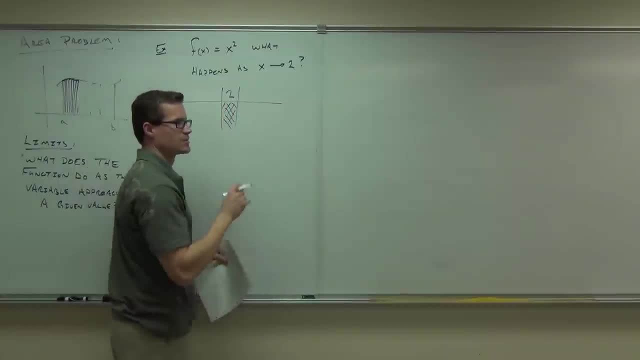 I don't care what that value is. What I'm trying to see is what the function is doing, as I'm getting close to that thing. So what's happening as we approach it from the right? What's happening as we approach it from the left? 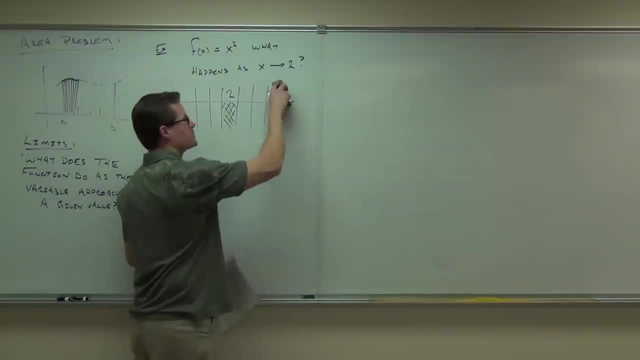 Give me some. oh, I already ruined it. Give me some numbers. Give me some numbers to the right of 2.. Some numbers to the right, 3., 3., 3.. Give me something smaller than 3., Like 2.5.. 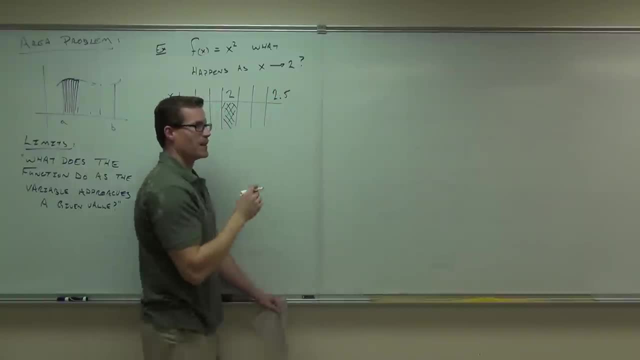 2.5 is good. I like that. That's what I was about to write. That's why I was ruining it. Give me something a little bit closer to 2.. 2.3.. Closer than that, maybe? 2.1.. 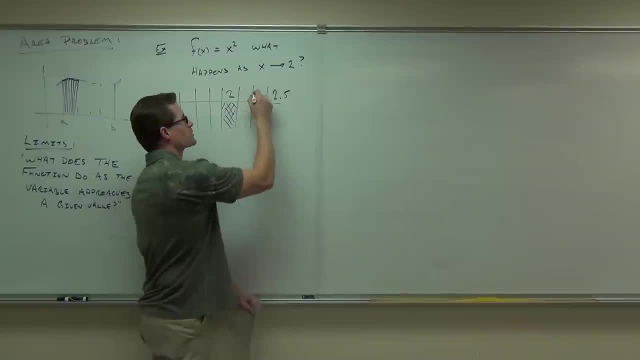 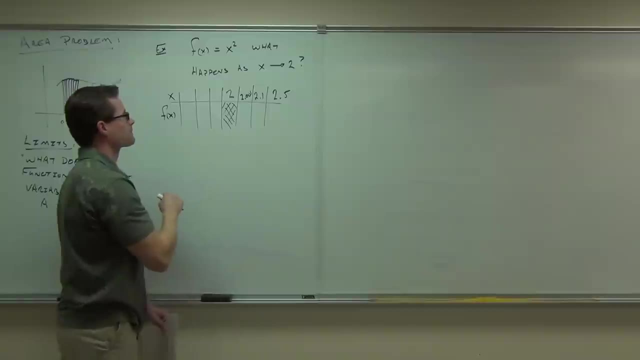 2.1, yeah, or 2.01.. We want really close, right? So 2.1 and maybe 2.001.. That's pretty close. Take your calculator out, by the way. Now let's go the other way. 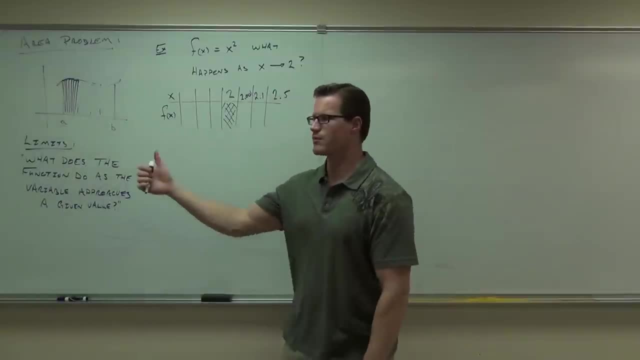 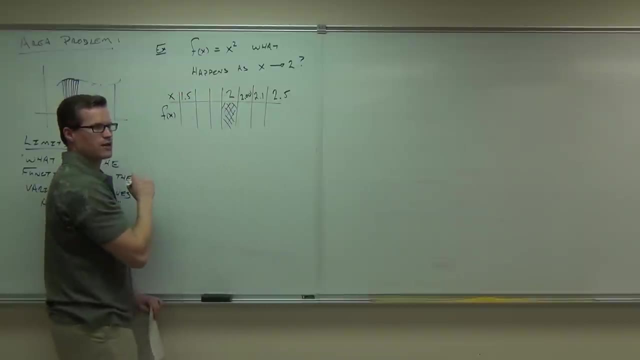 Give me a number that's smaller than 2 that we want to work our way up from this way: 1.99.. Okay, Sure, how about we keep it kind of symmetrical: 1.5, I like that one. 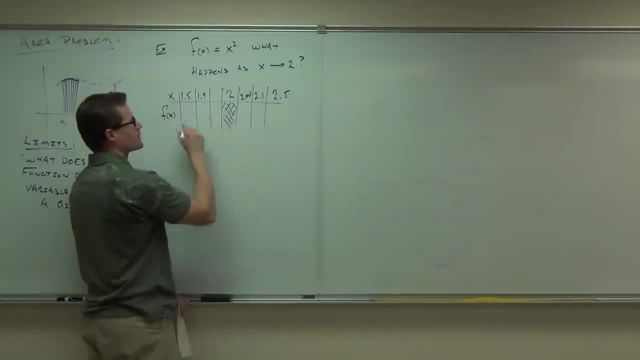 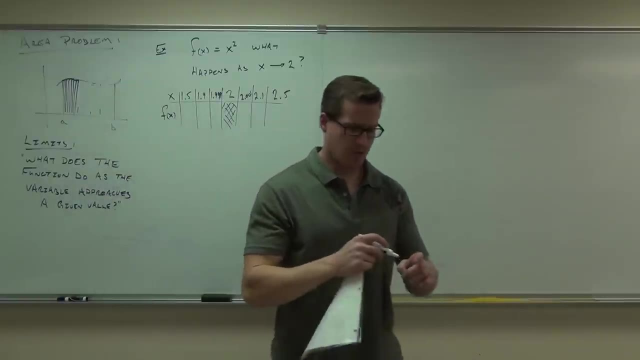 We'll do 1.9,, all right, and 1.999.. How about that? Does that work for you? Take those numbers, our function's x squared. Let's look what happens to the function as we plug those things in. 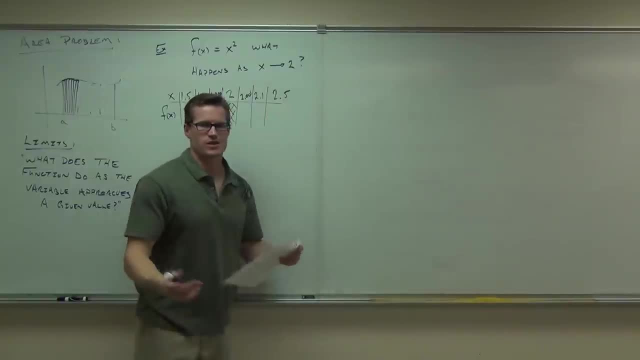 If you plug in 2.5, what do you get when you plug in? is it 6.25 or something like that? Plug in 2.5, do you get 6.25?? Yeah, Okay, So we'd start with 6.25.. 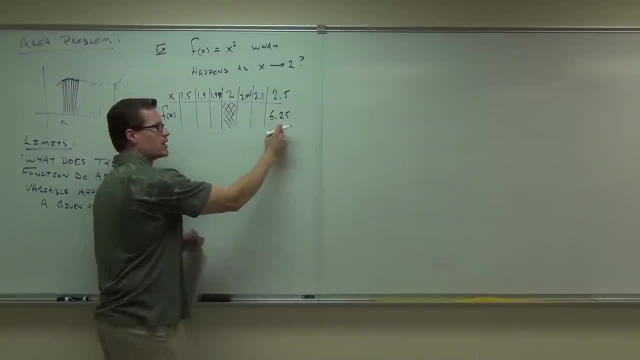 What we care about is: does this side look at the board? If we go this way and we go this way, do they meet up at the same point? That's what we're talking about for limits. Now, this is a very easy example. 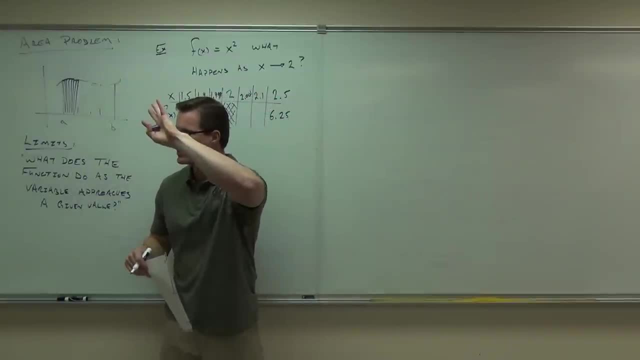 We just we're working with x squared. We know the answer's going to be 4, right, Or at least it should be 4.. We're going to see if that actually happens when we, when we evaluate our limits, Plug in 2.1, someone out there? 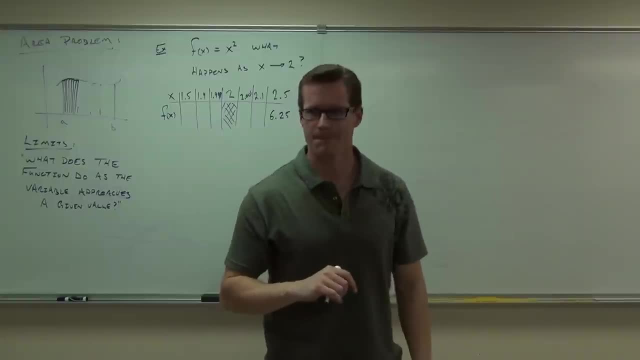 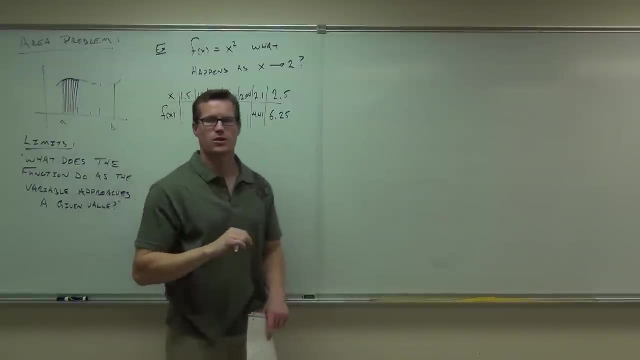 Tell me what you get when you plug in 2.1,. would you 4.41.. 4.41? Okay, that's closer to 4.. Tell me what you get when you plug in 2.001.. 2.004.. 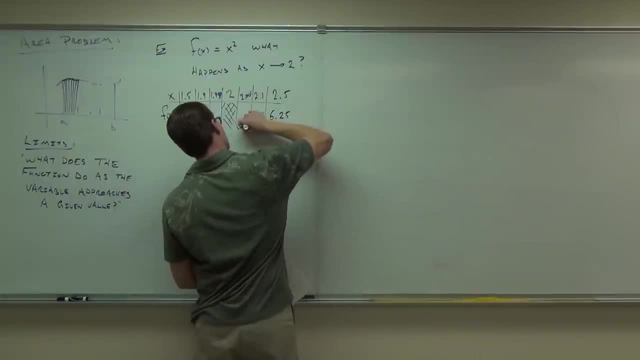 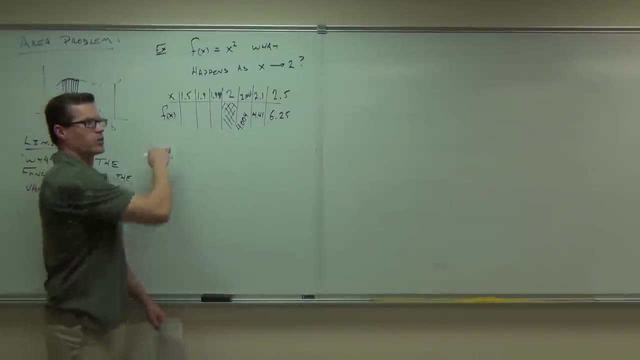 What was it? 4.004,001.. How about that, Like that? How about 1.5?? Oh, that's 2.25.. Isn't it? How about 1.9?? Plug in 1.9.. 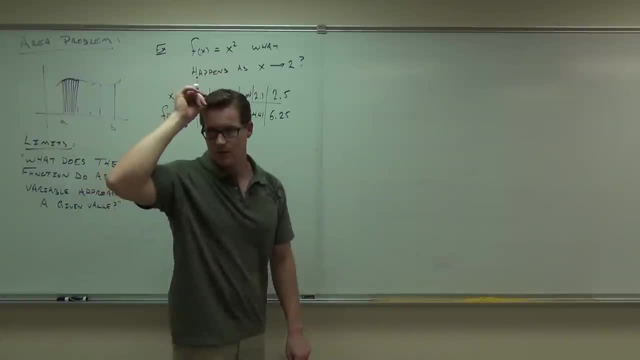 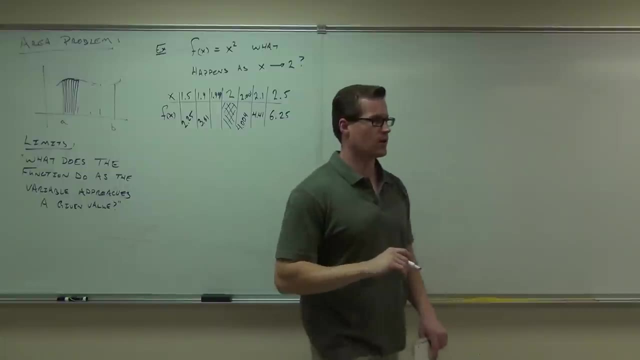 What do you get when you do that? x squared, 3.6. 3. 6. Okay, And now do 1.999.. 1.999.. What do you get? 2.9.. How much. 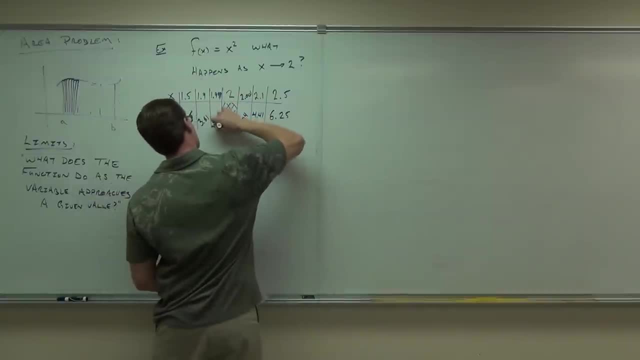 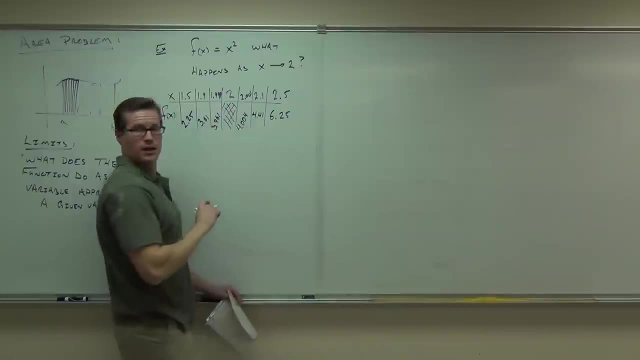 3.960.. 3.960?. 1. Emma, Yeah, Yeah, Okay, cool, What's going on here? Let's see, With a limit, we really don't care about what happens at 2. Because a lot of times, what you're going to find out is that we deal with limits where 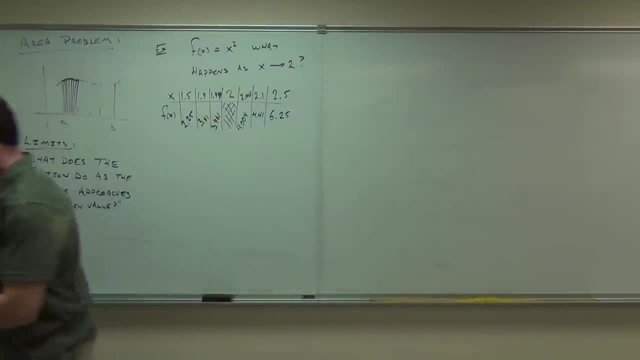 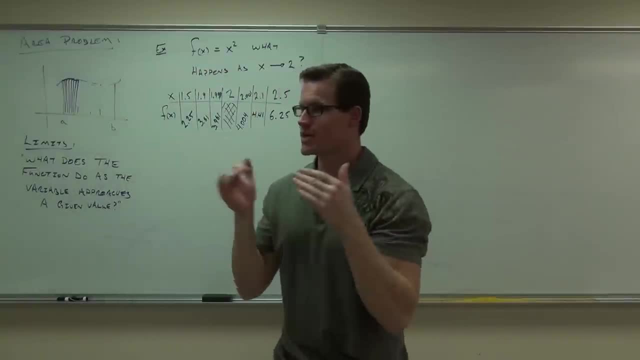 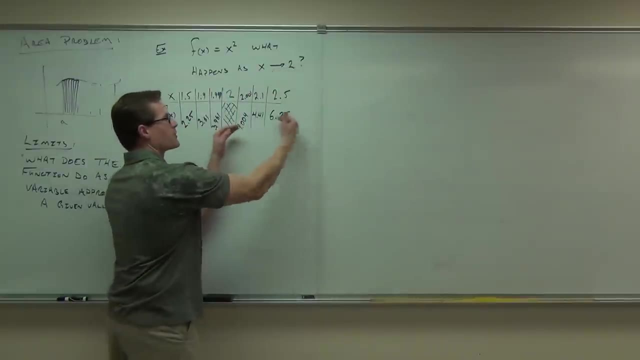 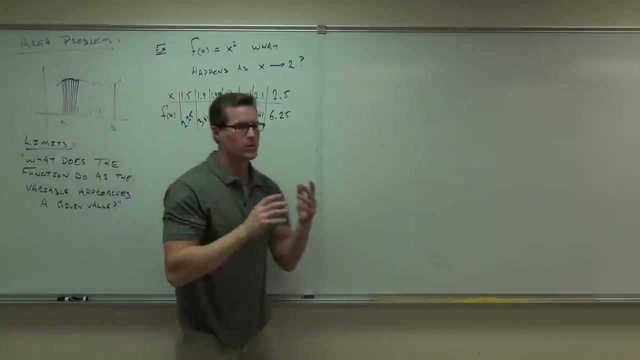 to 4,, down to 4, down to 4, down to 3, down to 3,, down to 4,, down to 4, 4, and where's this heading Towards the lower right? Where's this heading? 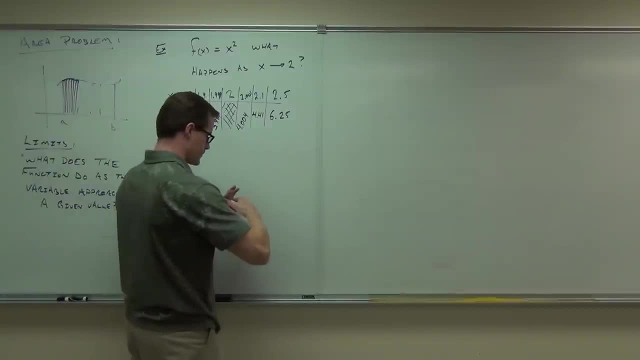 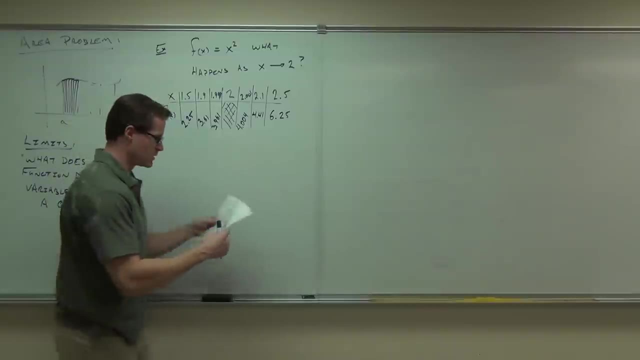 hacia 4. A couple notes about this. the function must approach the same value from both the left and the right. So this is from the right, this is from the left. The function must approach the same value from the left and the right for the limit. 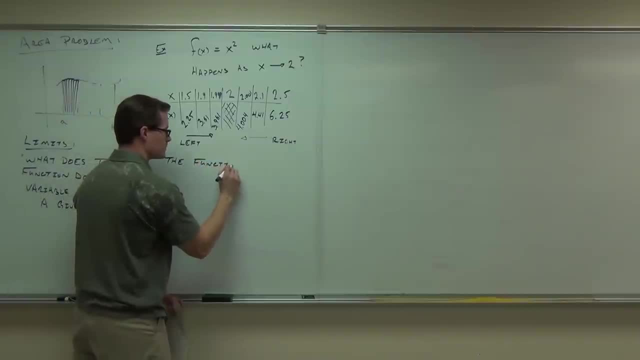 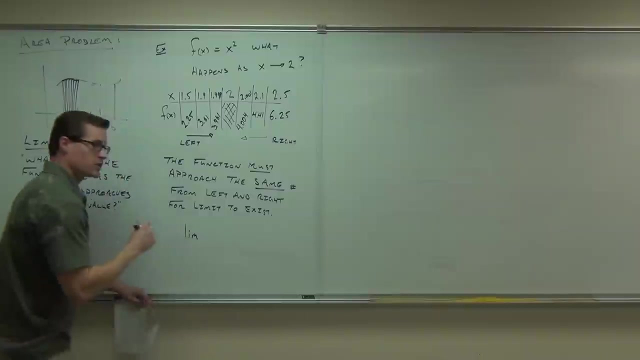 to exist. If it does. here's how you write the limit. What you do is you put a little limb under case, which kills me because I can only write in capitals. So you put the limit, you put the variable you're working with, you put that little arrow. 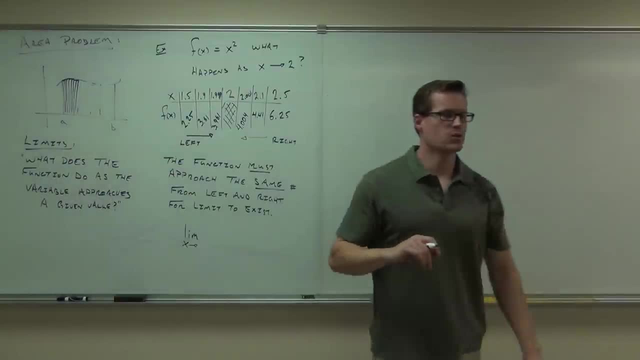 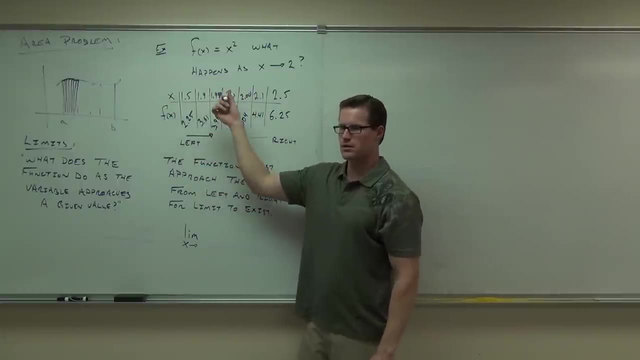 which I already told you is approaching, and you put the value to which x is approaching. X is this one. Where are we trying to get to on our x 2.. We're trying to find out what happens around the point. x equals 2.. 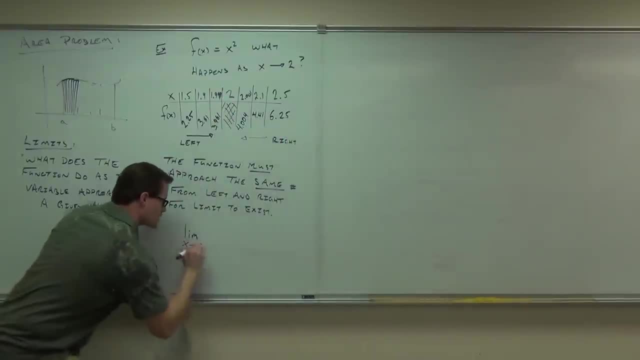 Does that make sense to you? So you say the limit as x approaches 2 of your function. what was our function? Say it again: X squared, X squared. The limit as x approaches 2 of our function is equal to what did the function approach? 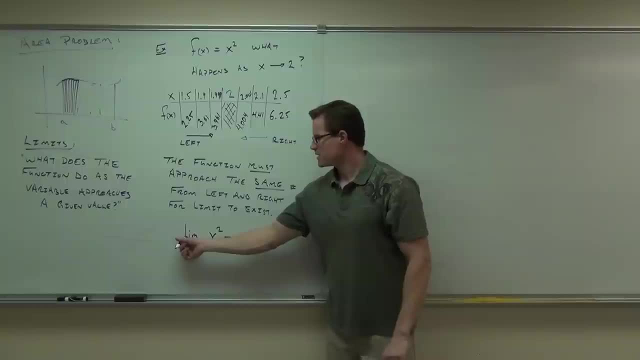 Here's what this says in English. okay, Look at the board. What does the function approach as the value x approaches 2?? What's the function approach as x approaches 2?? What's it going to do? That's the limit. 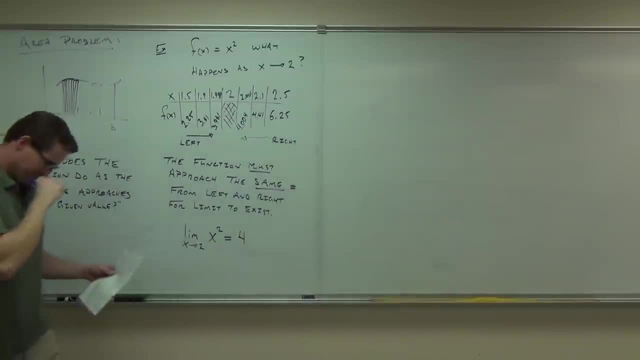 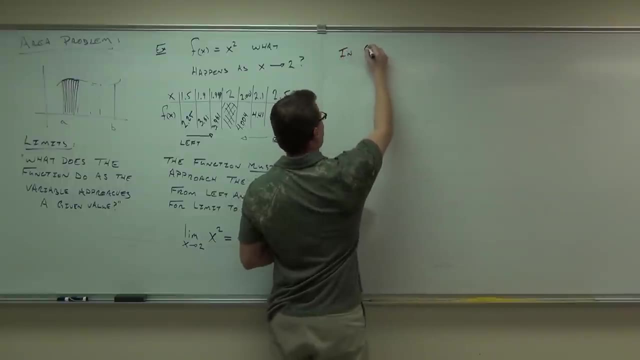 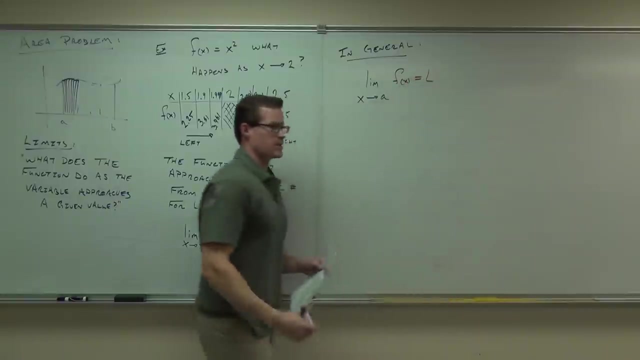 In general, we have this. This will be the last bit We've got. a limit of a function is equal to some number. That's what capital L is. That would stand for the limit. That would stand for the limit of this function as x approaches a. 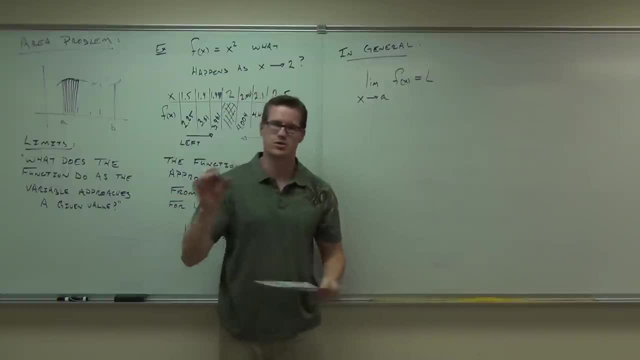 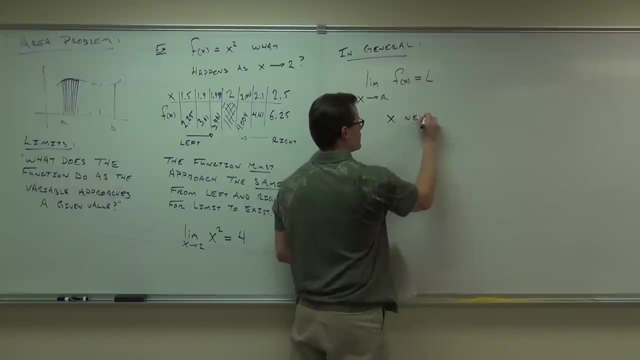 It's what the function is tending to do from both sides as x approaches one single value. The only thing that we need to know is the limit really doesn't depend on getting to a. X is never going to equal a. X never gets to a. 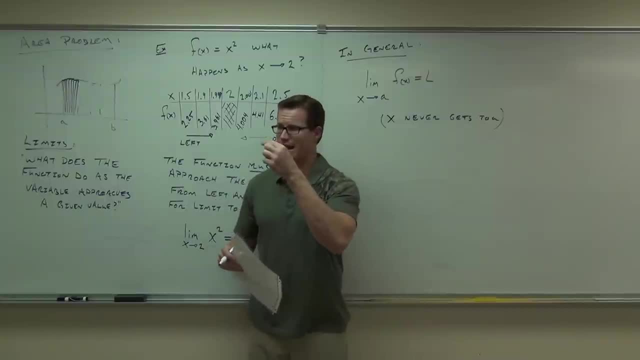 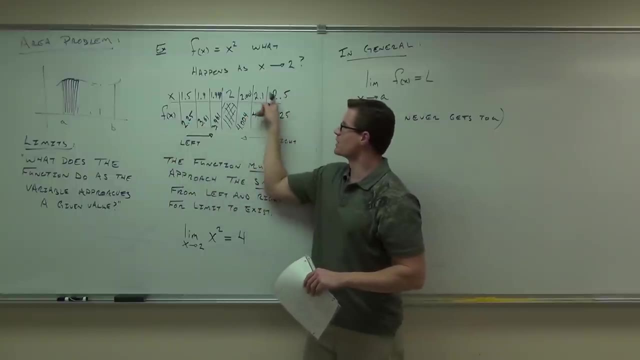 We just care about what's happening to the value of the function. We just care about what's happening to the value of the function, as x is getting really close to a from both sides Up here on the board. what's happening to the function, as x is getting really really close to a from both sides. 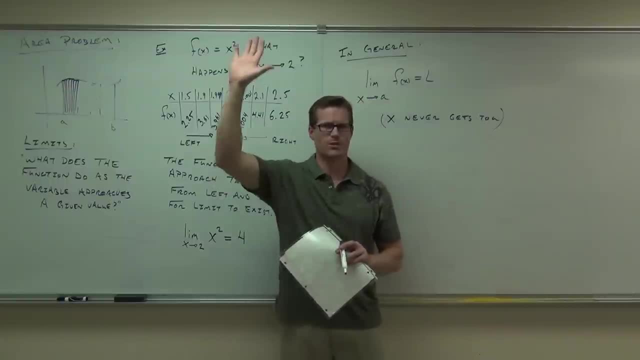 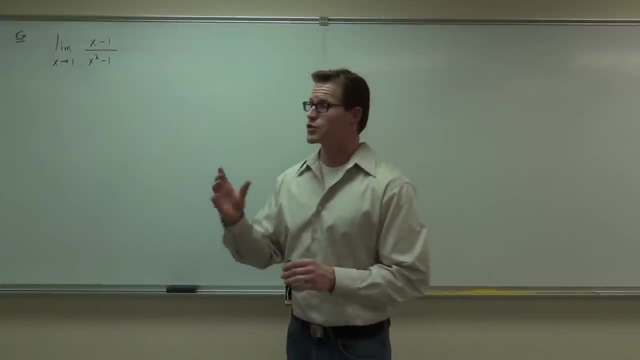 It's getting really, really close to 4.. That's the limit. How many of you understand the idea of a limit? Cool, Next time we'll work on how to find some limits, All right. So if you remember from last time, we're talking about limits. 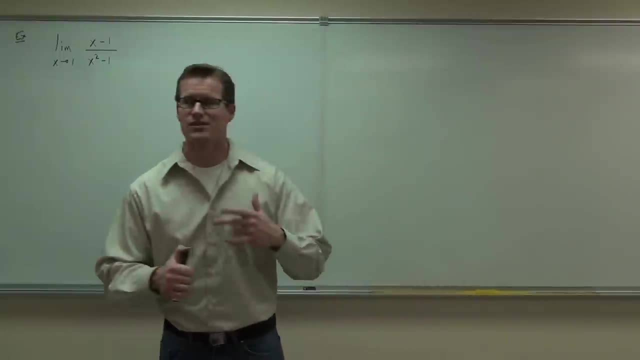 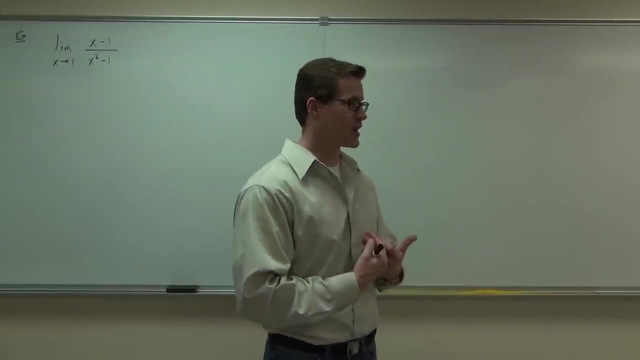 And what we're realizing is that a limit basically says, or asks the question: what is the function doing? What's the value of the function doing? What's the value of the function doing as x approaches a certain number? Now, do we ever care what happens when x gets to that number? as far as a limit is concerned, 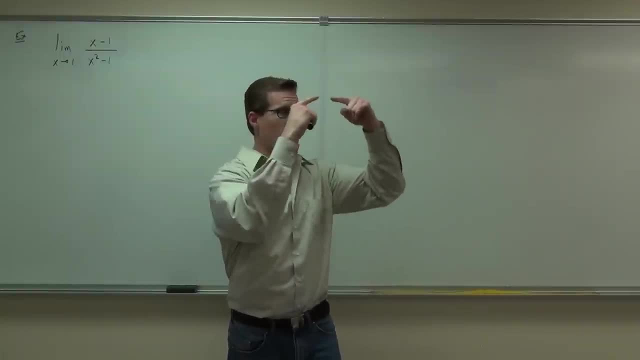 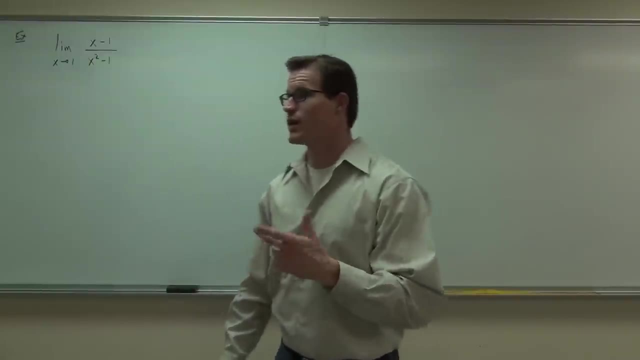 No, No, not really. Just what's the function doing? Where's it getting close to? as we're getting close to that x value, And that's the idea here. So when we're talking about the limit of x minus 1 over x squared minus 1, that's our function. 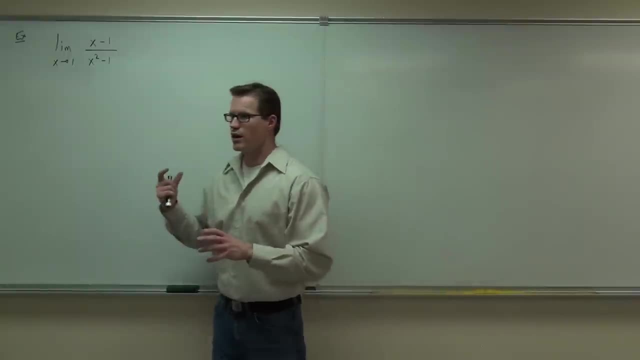 we want to find out what happens as x approaches 1.. Now why can't I figure out what happens when x equals 1? Tell me that That would be undefined, right. As a matter of fact, it makes both the numerator and denominator 0.. 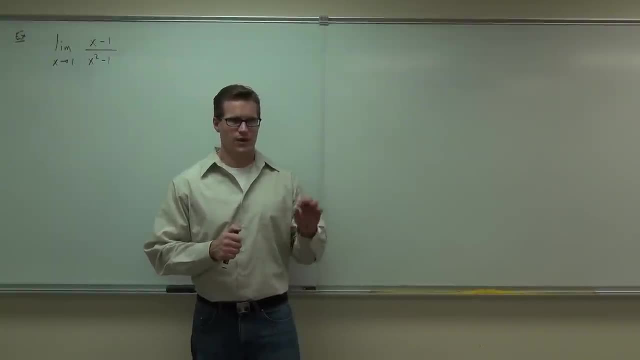 And that would still be undefined. We found out that that's. is that a whole or an asymptote? Do you remember? That's a whole, That's going to be a whole. Ultimately, this function has a whole. So what we want to find out, though, is what's the function doing as we approach that certain value? 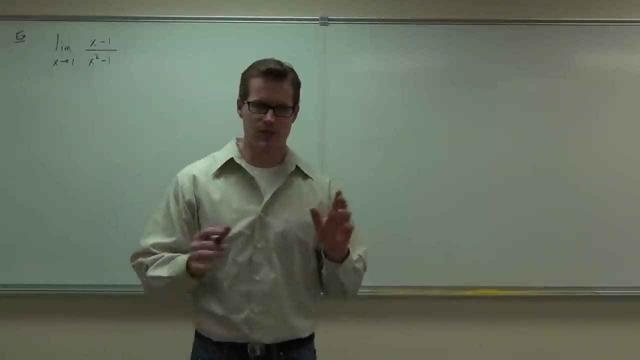 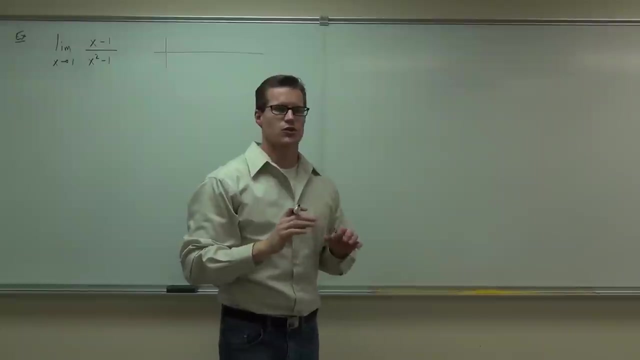 Now, one way we figured out- the only way we figured out- these limits is to make up a table, And this is kind of the elementary way that you discover limits, right when you first learn. Now, towards the end of the day, I'll teach you some better ways on how to do this. 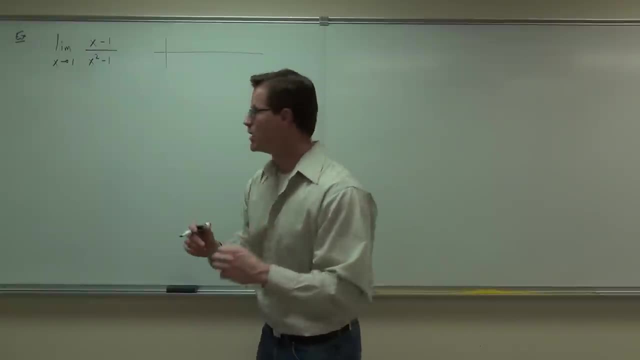 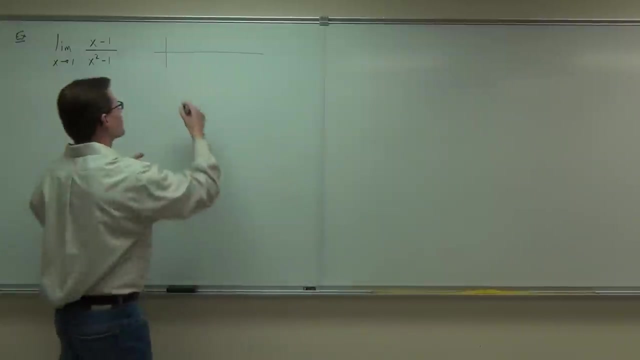 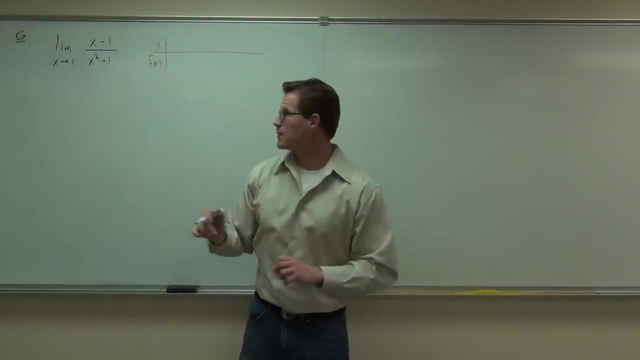 But right now, though, I want you to see what happens with the function, with the limit. So when you are finding these- and your homework's going to ask you for that, find the limit of this function by making a table of. When you do that, you have your x values on the top, you have your f of x values on the bottom. 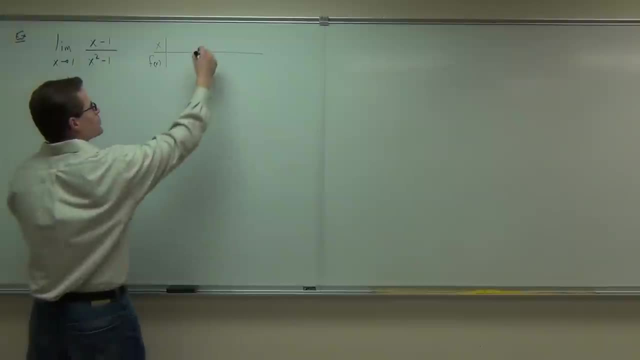 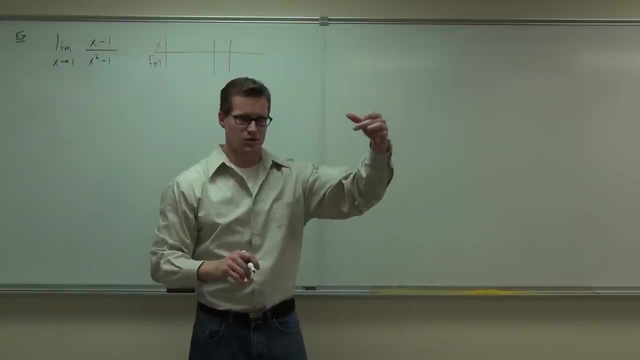 in this case x minus 1 over x squared minus 1.. And you start with the number. you want to find the limit of the number, that you want to find the limit of the function where x is approaching that certain value. Put that in the middle. 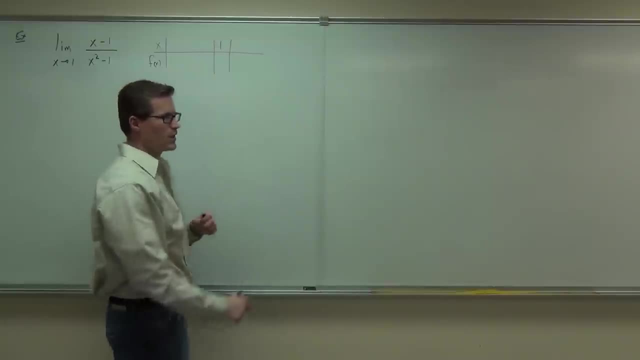 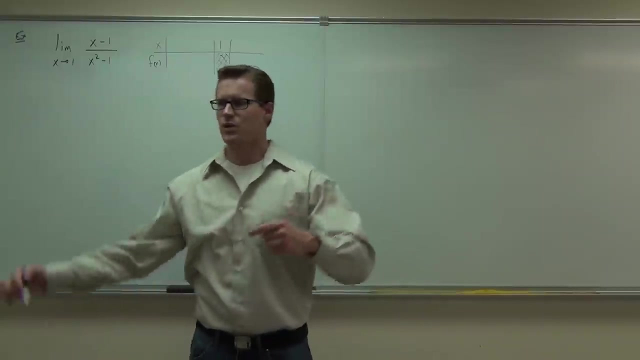 So, for instance, you're going to put 1 right there And really I don't want to know what that is, because you can't plug it in anyway. What we want to find out is what's happening from both sides. Is it going to the same value? 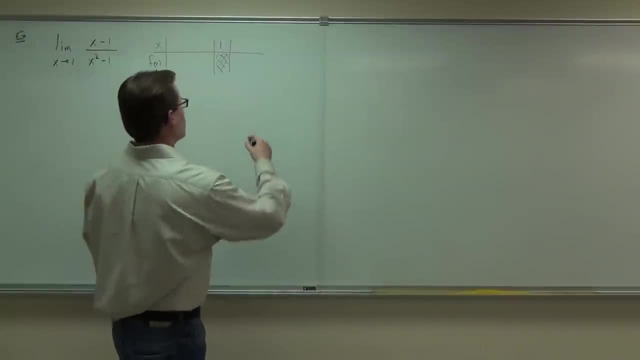 You follow me on this. So what you need to do now: put these numbers in order, because it is a number line You don't want to have like I see a lot of mistakes on this. I see a lot of people do this. 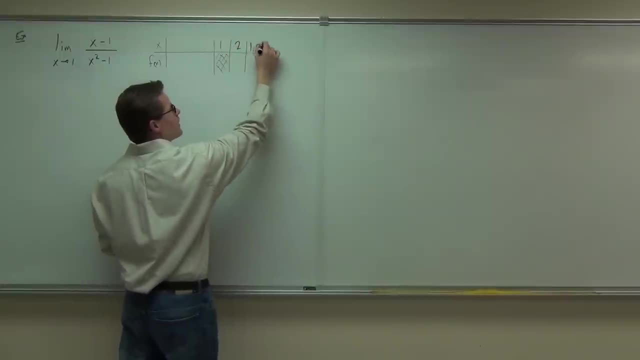 Okay, well, I'm going to start at 2,, and then I'm going to go to 1.5,, and then I'm going to go to 1.1,, then I'm going to go to 1.0001.. 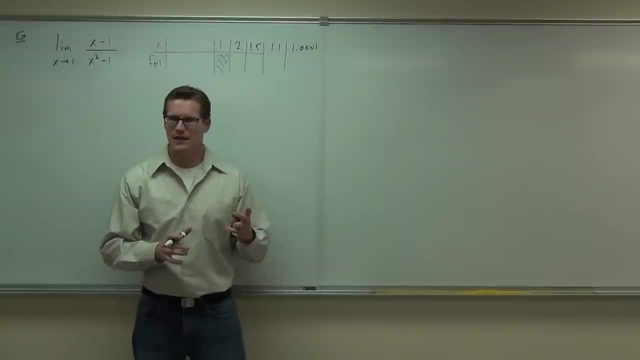 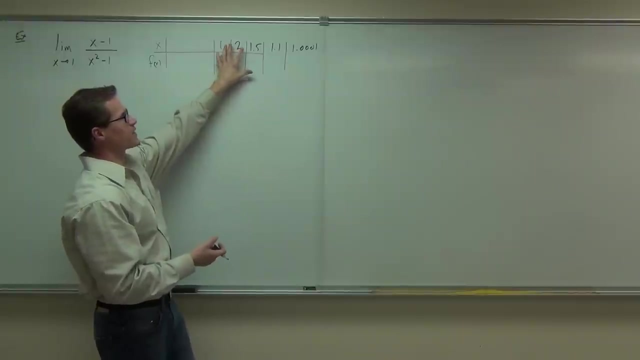 Do you see how that's the wrong way to do it? That's going to show you one direction, but it's the wrong direction. You need to have these numbers reversed so that this is just a little bit past 1.. We're coming from the right-hand side. 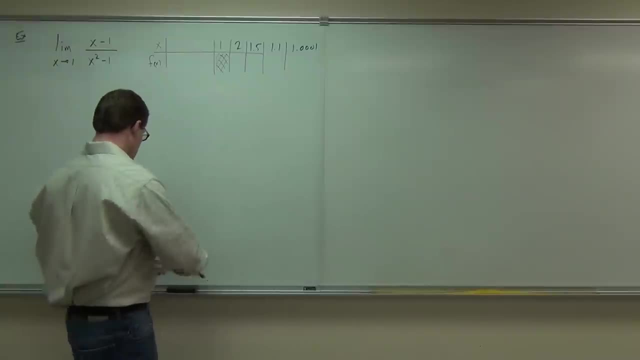 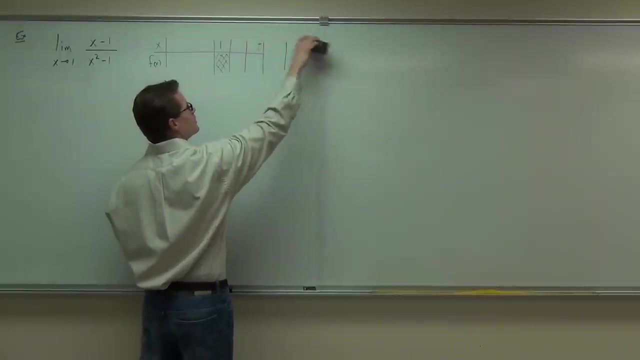 So if you want to find out where it's coming from, don't have 2 right here. Have 2 over there somewhere if you're going to do that. So these numbers that we have next to 1, they should actually be the numbers that are close to 1,. 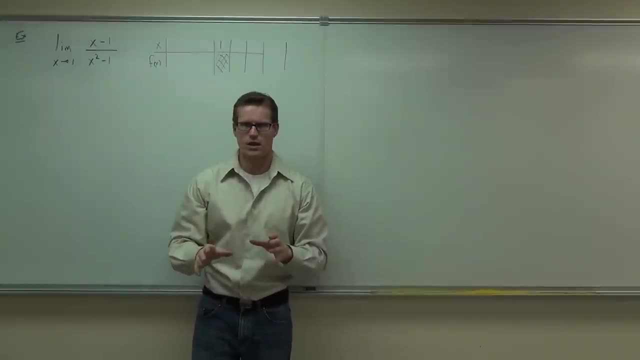 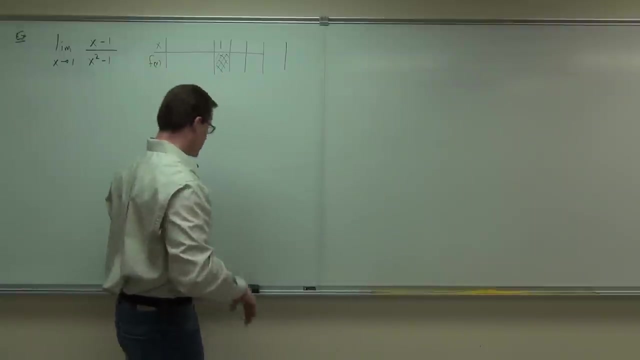 not the other way around? Are you following that? I'm not sure if you're okay with that. So we don't want to have the smallest numbers over here, the ones that are closest to 1 over there. We want this just like a number line in the book. 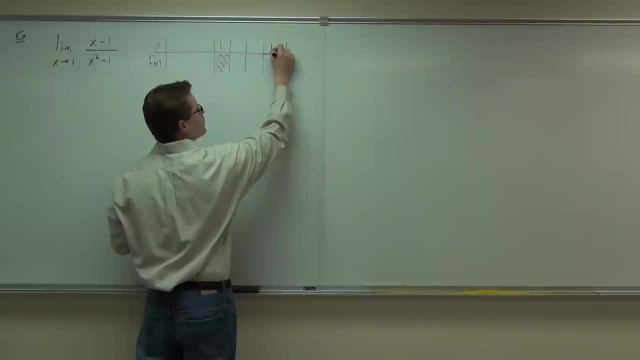 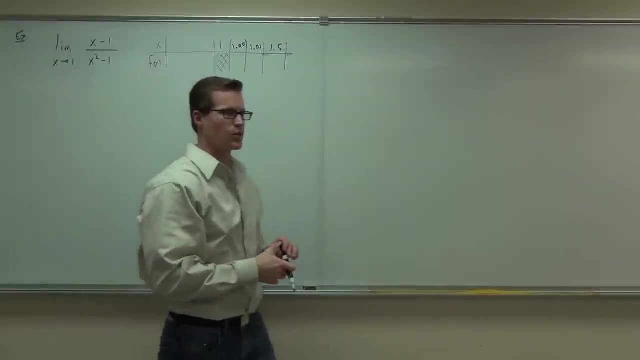 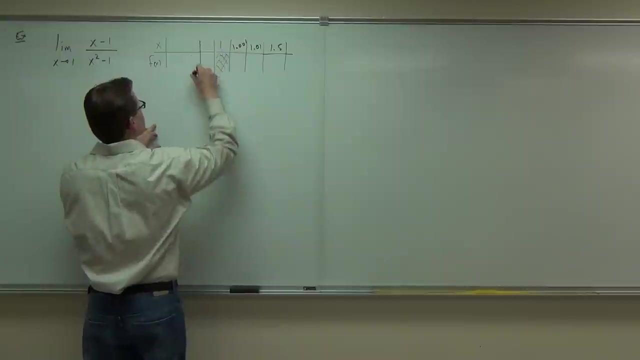 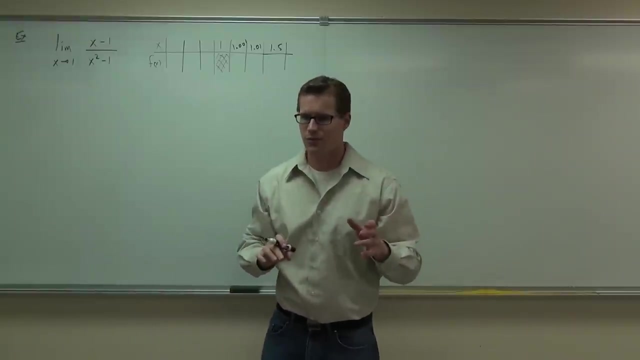 So here maybe we do start with 1.5, 1.01, 1.001.. Make it really close to 1.. Now the other way, I'll probably want to start with 0.5.. I want to make it symmetrical at least a little bit. 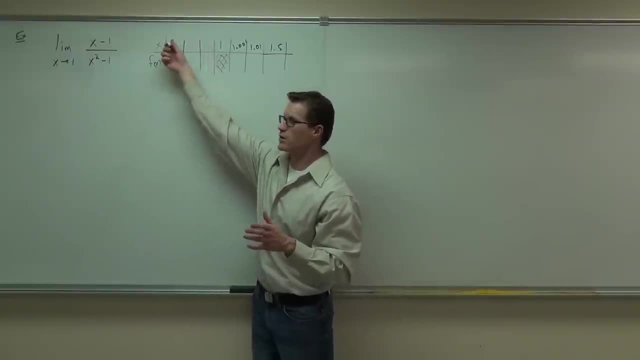 So where's 0.5 going to go? Is it going to go by the 1 or over? here on the left-hand side, Left-hand side, I want the numbers that are really closest to 1.. Well, the closest to 1.. 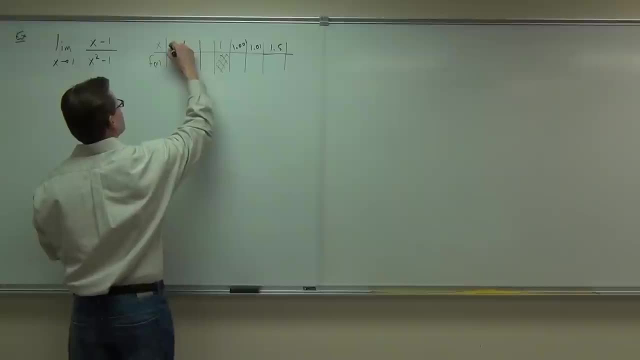 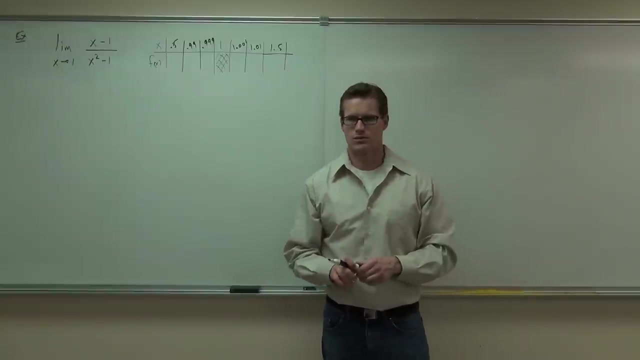 That's going to show me the trend. So 0.5 may be 0.99 and 0.999.. What I'd like you to do right now, on your own, take out your calculator, find those numbers. How about this? 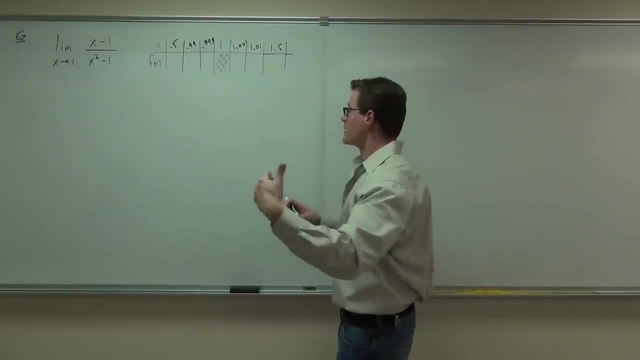 The people to the left side of the camera do these ones. okay, People to the right side of the camera do those numbers. Can you do that for me? So plug them into the function. Tell me what you're getting out. 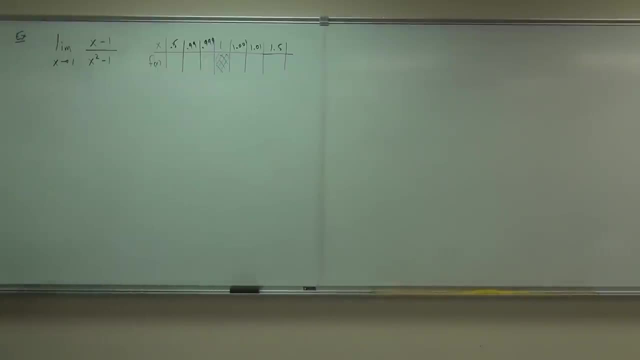 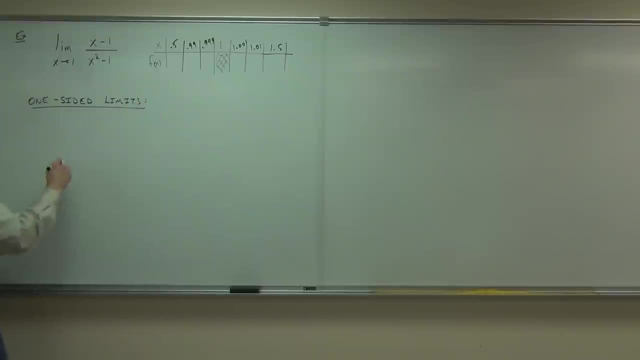 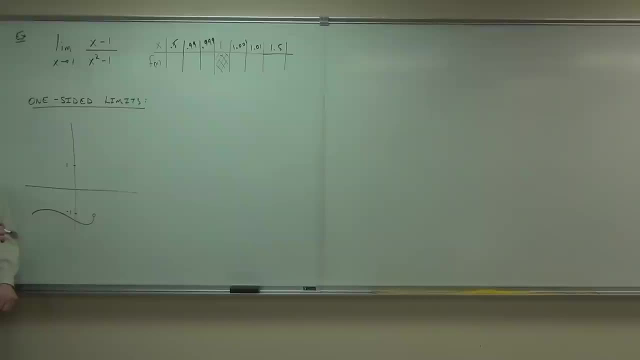 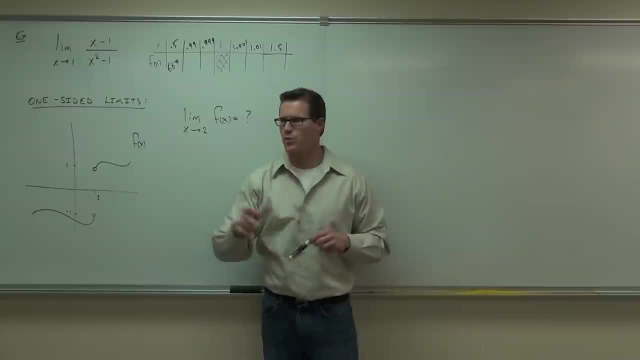 So six point six, seven. How about the point nine, nine. Did anyone find that one Point nine nine? Five point zero. five, two, five. Can I get a double check on that Five point, How much? Point five zero three. Point five zero three. 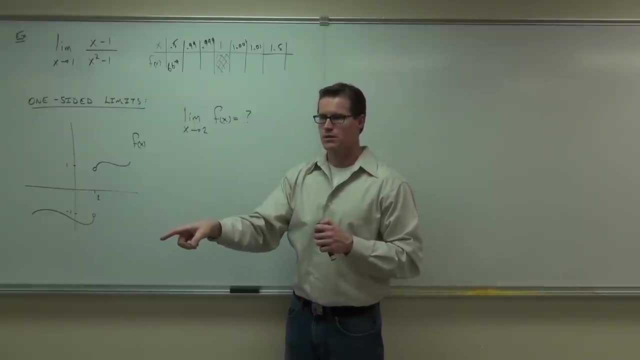 How about for this one? That's the one, That one. Let's double check that. one Point nine, nine minus one. That should be pretty small, You know, negative something. One more double check. What did you say it was? 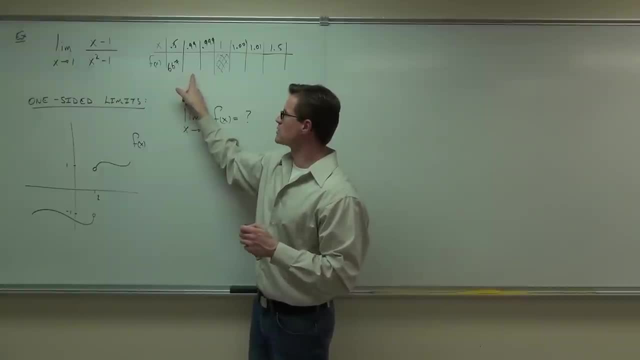 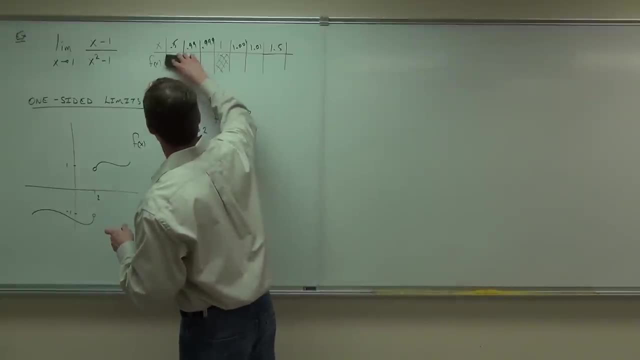 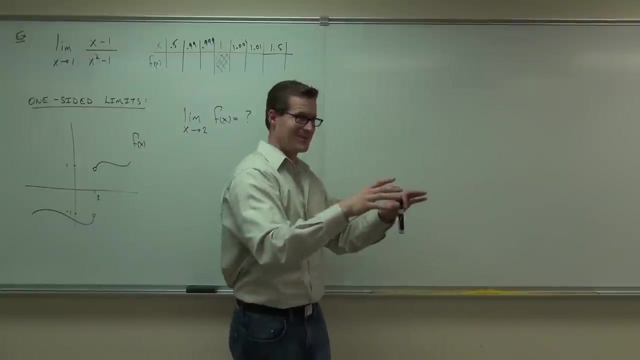 Okay, Okay, Okay, Okay, Okay. What did you get? if you're figure out your stuff, All right, I'll come back to you. all This side, Try this side, Try this side. Can you give me one point five? 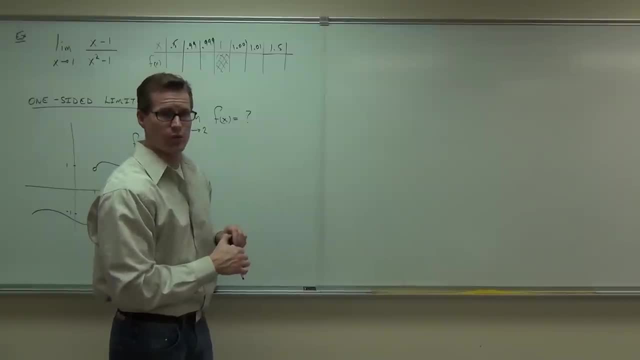 One point, How much? Point four, Point four: Yeah, Can you give me one point zero? one Point four. nine seven, How much? 0.497.. 99.7, I'll take it Okay. can you give me 1.001, please? 1.001.. 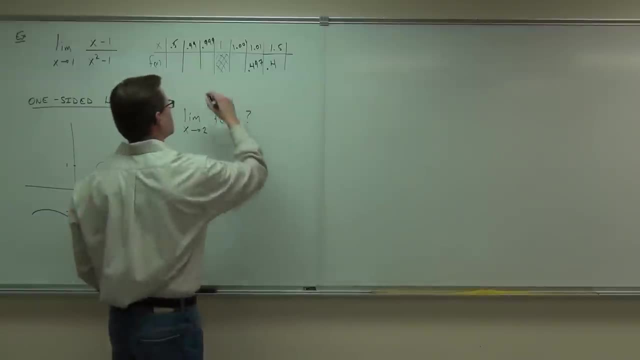 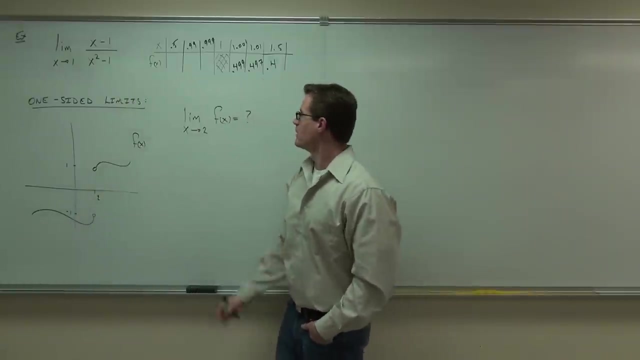 .499.. .499? Okay, Hm, interesting. I'm guessing the six was probably not all that accurate. Let's try that again. Ah, so .6.. Okay, give me .99.. Point, what .503?? 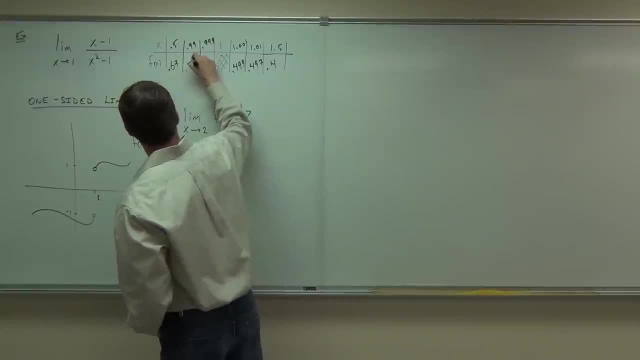 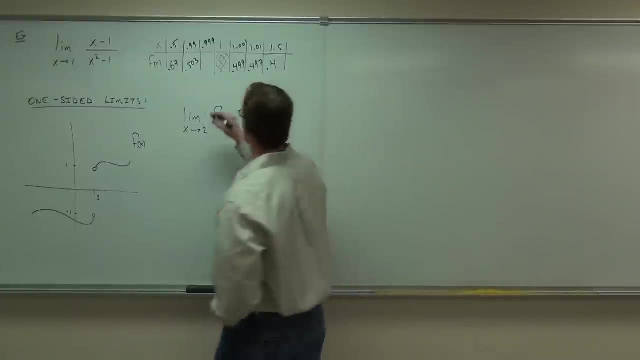 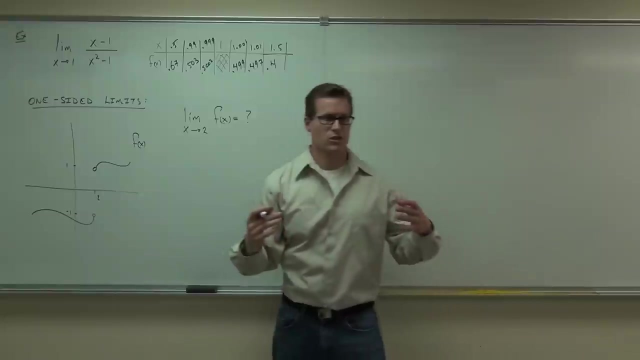 Give me .999.. .5002? Now, do you see the trend to which this function is getting close to? Can you see it? What number is it getting close to from the right? What number is it getting close to from the left? 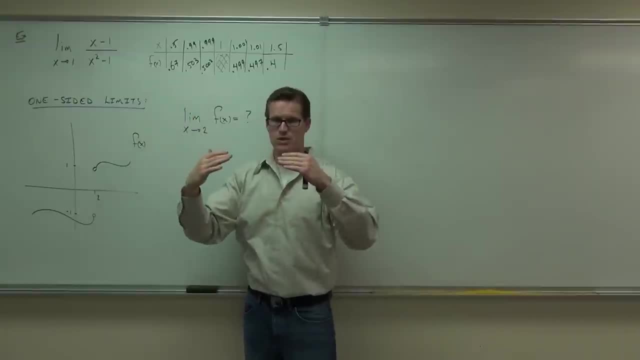 That's why you put it in this order, so you can see where it's approaching from the left and from the right. If it's the same number, if this is getting to .5 and that's getting to .5, you'd say okay. 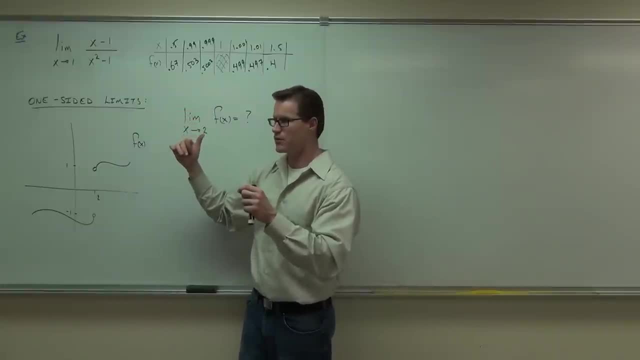 that limit exists and that limit is .5.. Are you following me on this? So the limit right here would be .5, and that's how you use a table to figure that out. Now, of course, this was a pretty mind-boggling right. 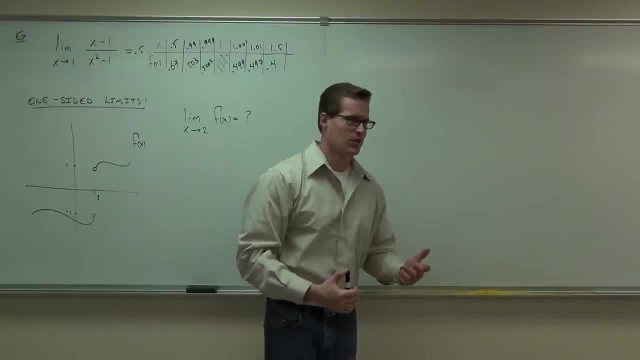 Who wants to plug in 1.001 and do all this for a whole bunch of numbers? Do you want to do that? No, I don't want to do that either, because it's boring right, We're going to find some better ways to do these limits. 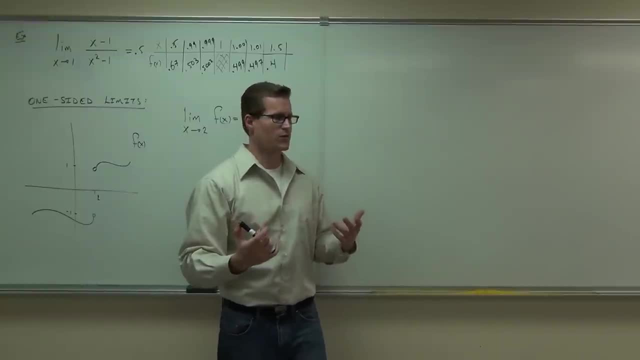 in the next section. For right now, though, I need you to get an understanding of what a limit is. A limit asks: what's the function? the value of the function, do as you get closer, as your x value gets closer to that. 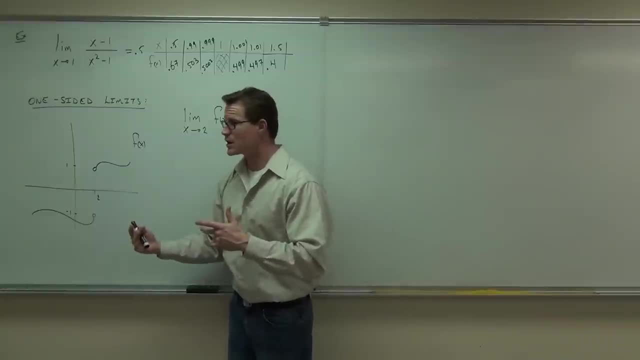 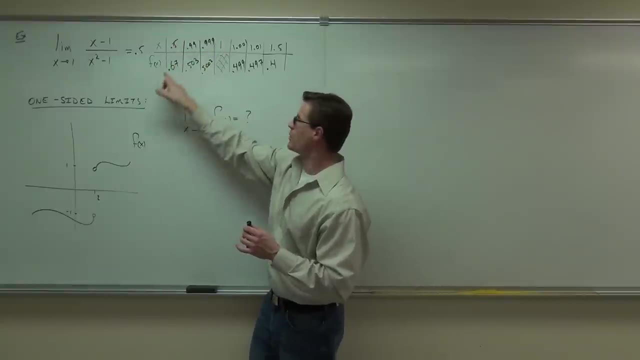 What's the function's value do? What's the function's value do as your x value gets closer to that from both the left and the right? 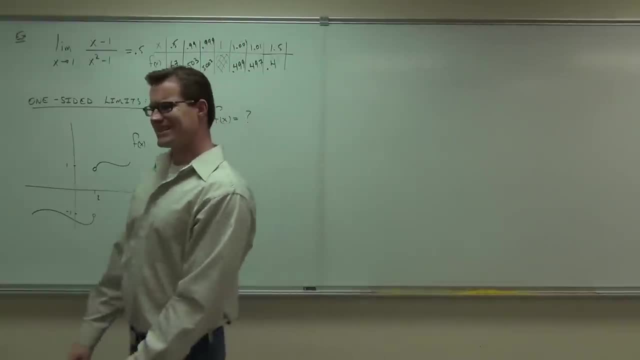 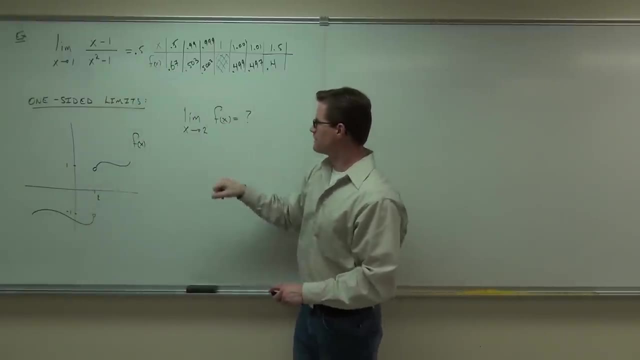 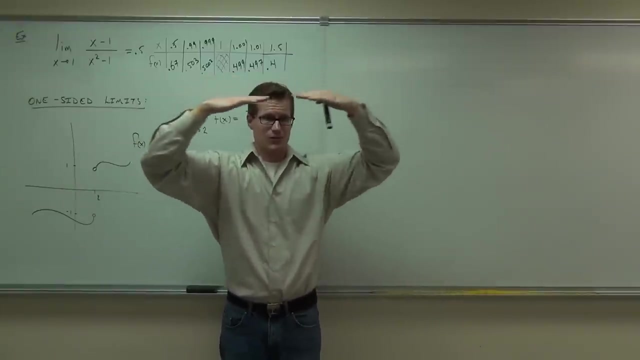 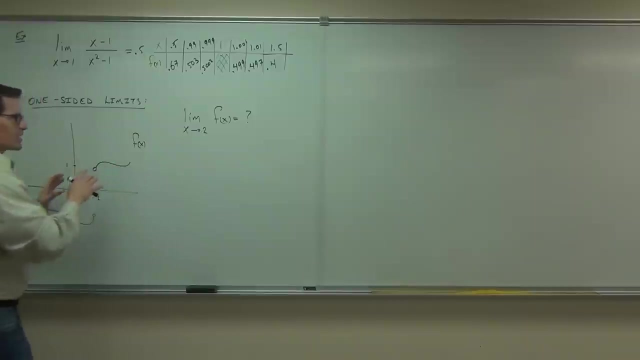 Which way would be? from the right over here or over here, Option one or option two? 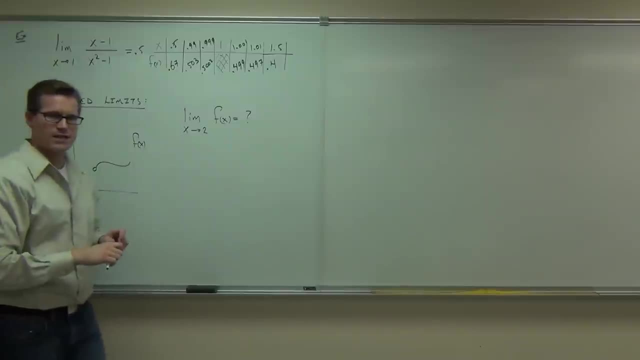 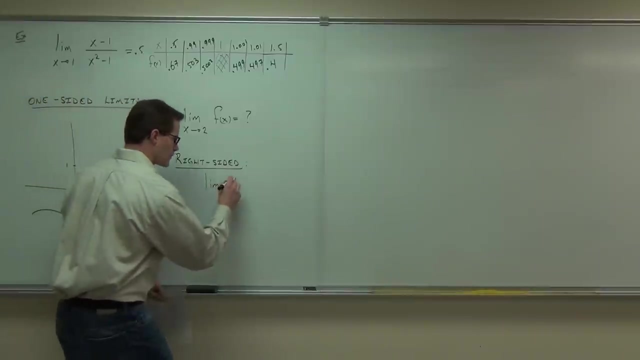 From the right would be this way? true, We can actually have right and left-sided limits. so here's how you write that A right-sided limit, in our case, would be a limit of our function as x approaches whatever value you're talking about. 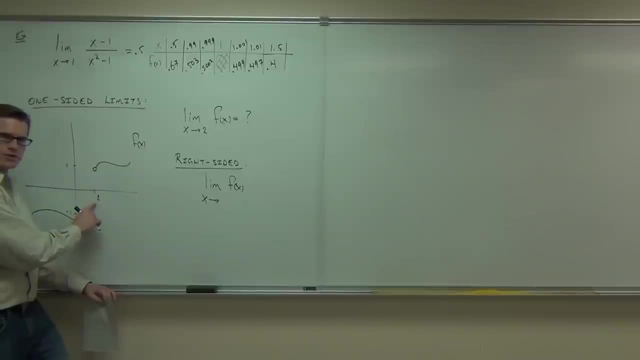 In this case, we're talking about the value two. Do you guys see where the two's coming from? in this case? We're gonna find out when x approaches two. And how you say from the right-hand side, is you put a little superscript plus? 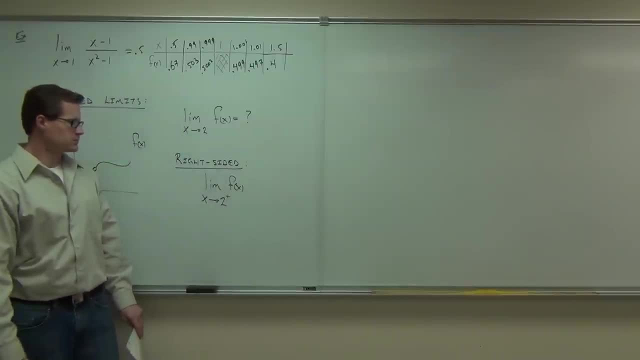 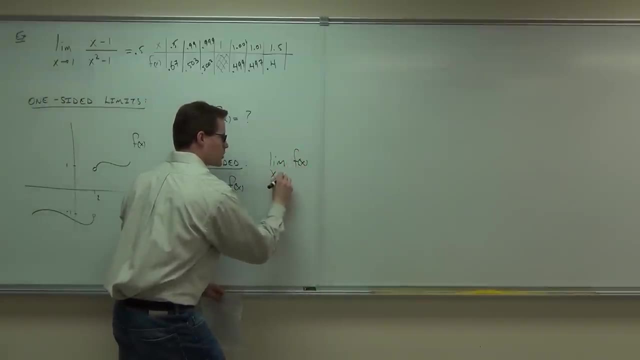 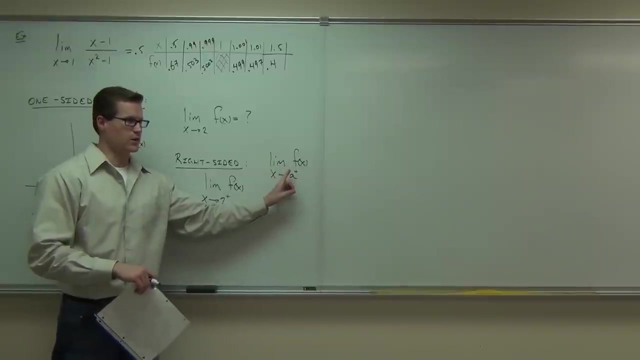 That means from the right. So in general you'd have this: You'd have a limit of F of x as x approaches A, some number that I give you from the right. That says a right-sided, one-sided, right-sided limit. Now, do you feel okay with that? 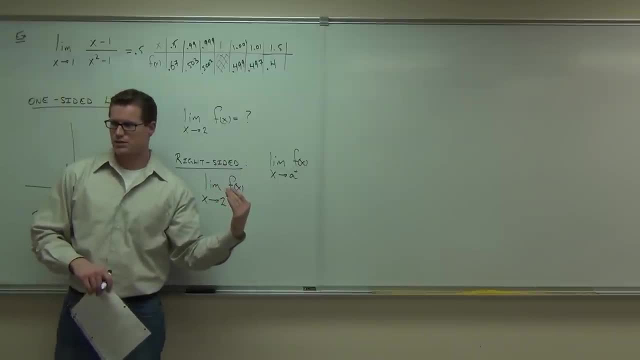 So plus means from the right. You all all right with the. plus mean from the right. What do you think a left-sided limit's gonna have, Right? Oh, you guys are geniuses. exactly, Yeah, a left-sided limit would be a left-sided limit. 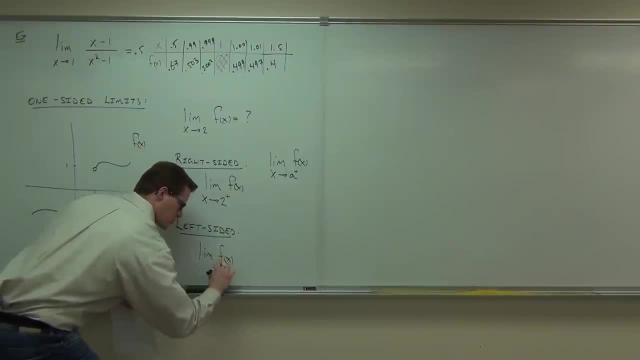 plus a right-sided limit Would be a limit of f of x. sure, as x approaches a certain number. In our case, our certain number is 2.. And that little minus or negative is from the left. In general we'd have the same situation only from the left. 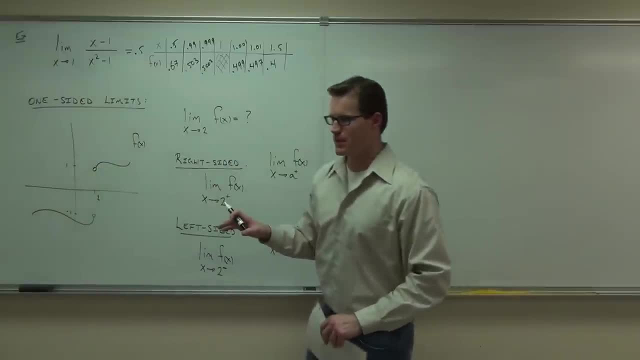 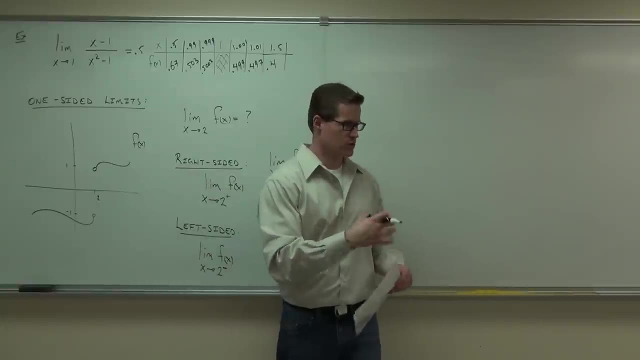 So let me ask you a question. Can you find the limits, both right-sided and left-sided, of this function? Let's try that together. Here's what the question. I'll go next so you can understand it. Here's what the question asks. 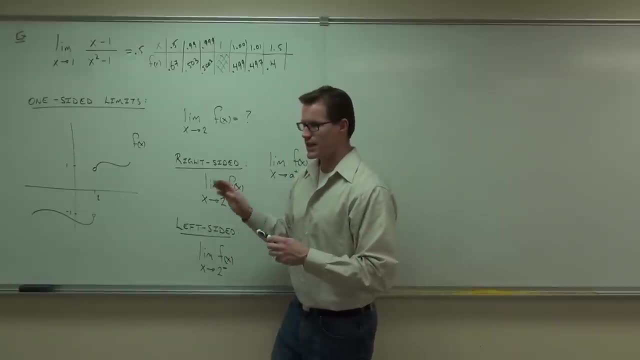 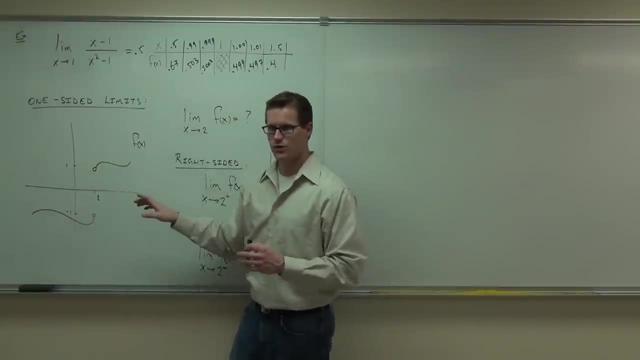 What is the value of the function as x approaches? 2 from the right for a right-sided and from the left for a left-sided. Okay, so follow the function along. I need you to tell me what the height of my finger is. What's the height of my finger when I get really close to this? 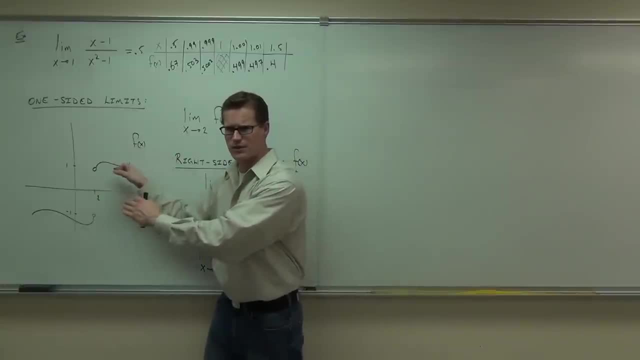 This is the value along this line. so this is from. am I going from the right or the left, in this case, From the right From the right? Okay, it's always from the. it's not to the, it's from the right. 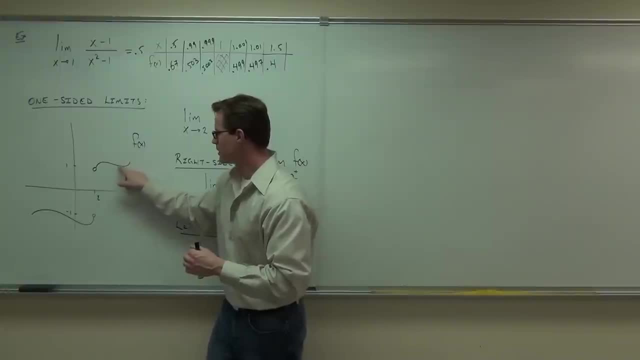 So, from the right, the height of my finger is okay. I'm a little above 1, a little above 1.. What's the height of my finger going towards as I slow down? I'm slowing down. what's the height of my finger trying to get to? 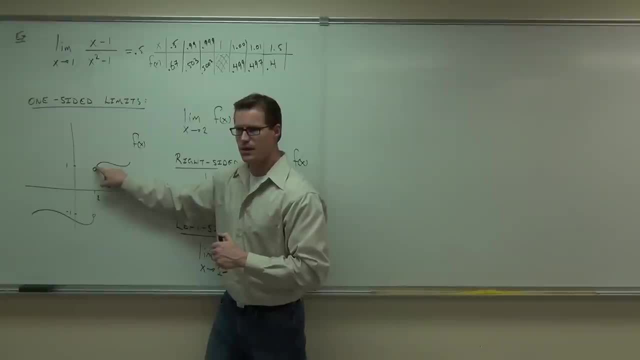 1. It's trying to get to. 1. Do you see that? It's not that my finger's getting close. it's not that the limit's going to be 2. It's saying what happens to the value of the function. the value is your y-axis. 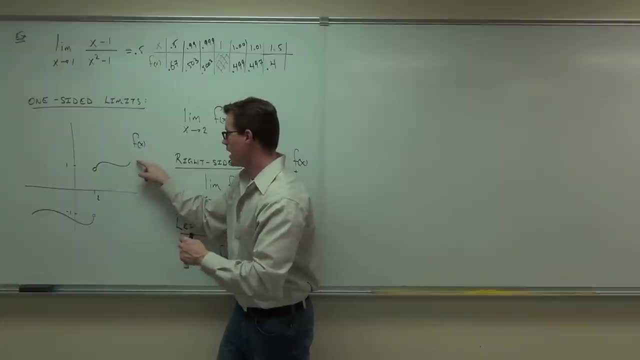 What's happening to the value of the function or the height of my finger as my finger is approaching in this direction, the number 2? Does that make sense to you? So here, the height of my finger is trying to get to 1 as I'm approaching 2 from the. 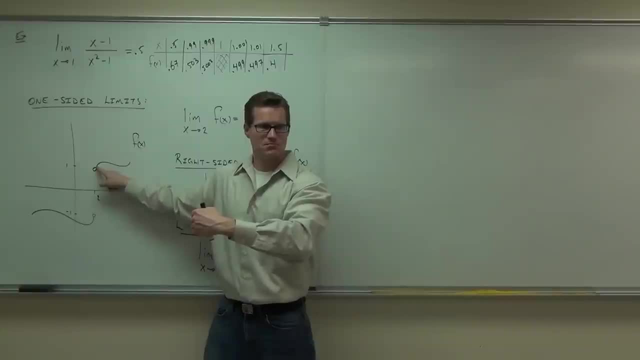 left From the right, From the right. That's what I said. From the right. I'll edit that out. you won't even know, Beep, Just kidding. I'm not going to edit that. it's going to be on there forever. 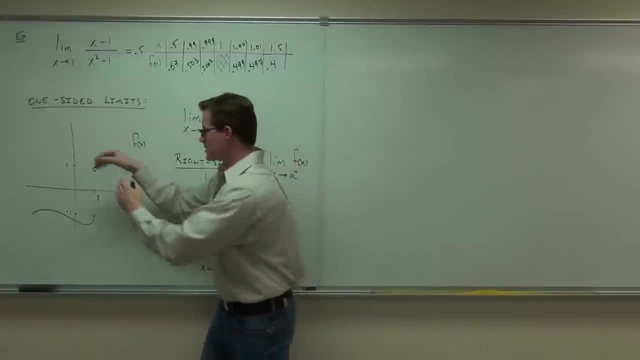 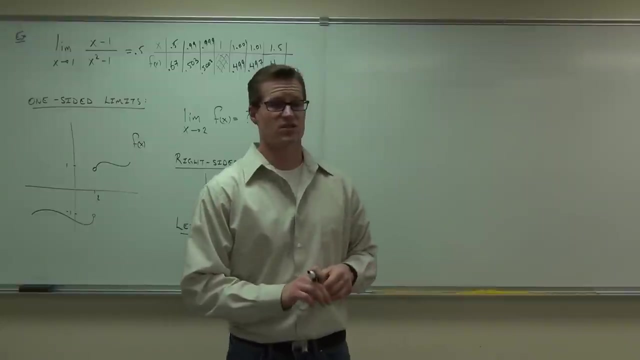 Yeah, so from the right. So from the right, it's going to be approaching 1.. Yeah, thanks for that. You okay with that being 1?? It's either yes or no. If you're not, that's okay. but I need to know. 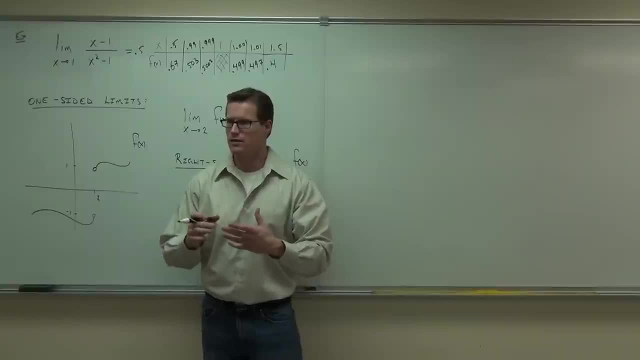 I need to have a question from you. if you're not, You guys. okay, with the height of that being 1, as this function's approaching an x value of 2?? So basically, you're asking: what's the y-axis, What's the y-value when you reach your x-value? 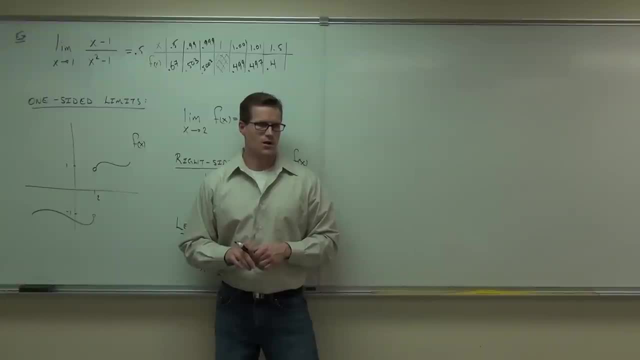 Okay, Okay, We didn't see you. All right, What's your y-value when you reach your x-value? So now we're going to do it from the left-hand side. What's the height of my finger, aka the y-value, as I approach the x-value of 2?? 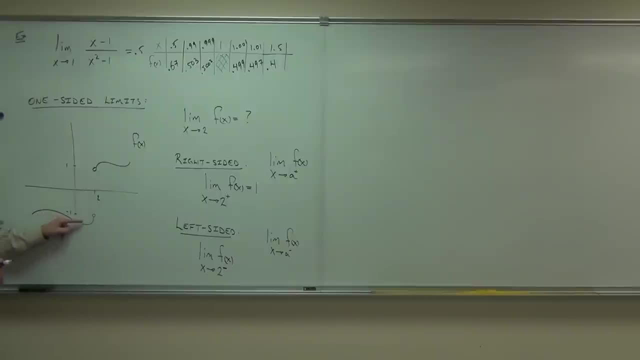 So what am I doing? where am I getting close to- as I'm getting to- 2 from the left-hand side? Where am I getting close to Negative 1., Negative 1. Yeah, absolutely. Now here's a little note. 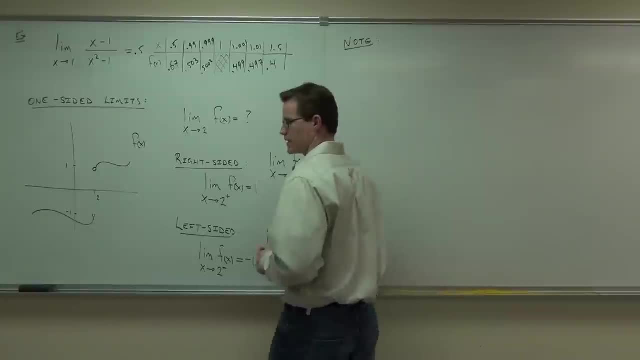 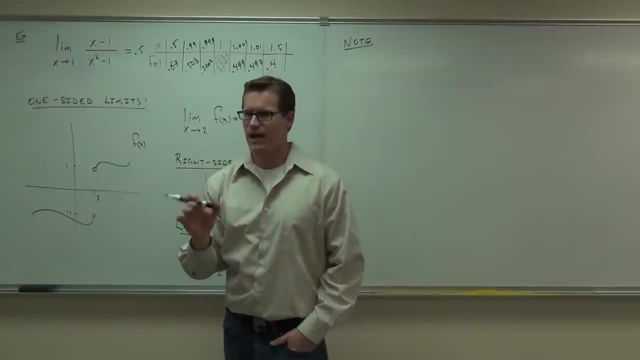 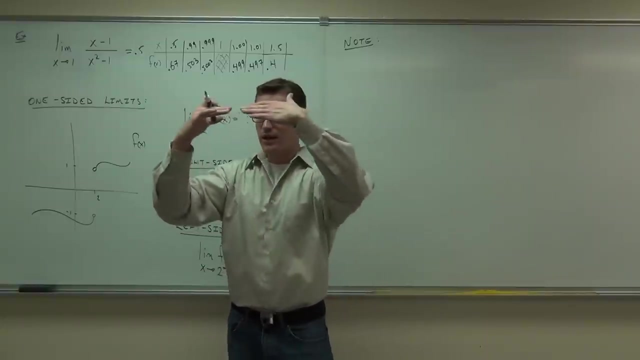 Here's a little note for you: In order for a limit to exist at a point, the left-side limit must equal the right-side limit. If it doesn't, then the limit doesn't exist. Does that make sense to you? It's got to go to the same place, otherwise the limit doesn't exist. 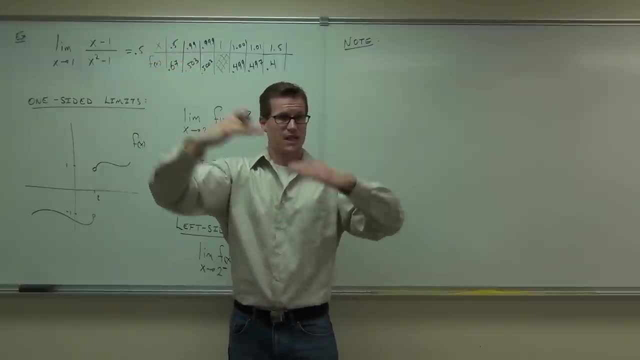 You can be one-sided, sure, here, here, but if it's not the same spot, then you'd say overall the limit. the limit means from both sides, the general limit means from both sides. So it's not going to the same thing. that limit doesn't exist. 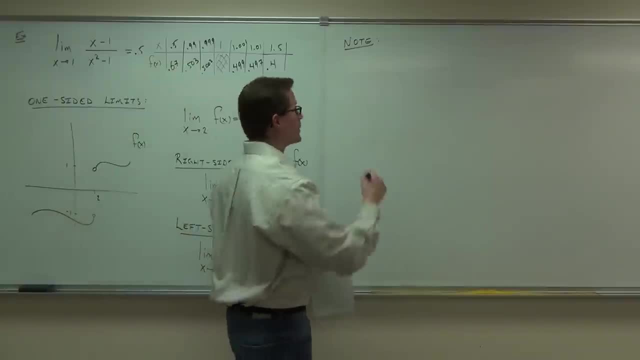 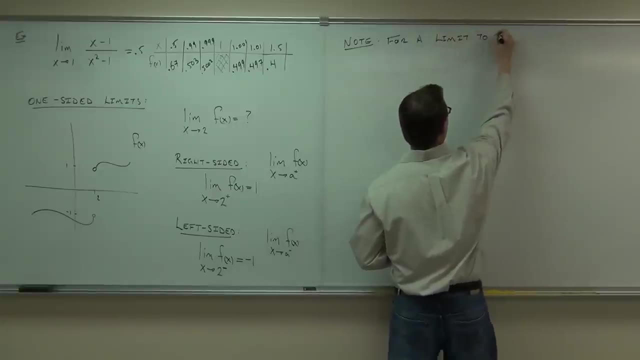 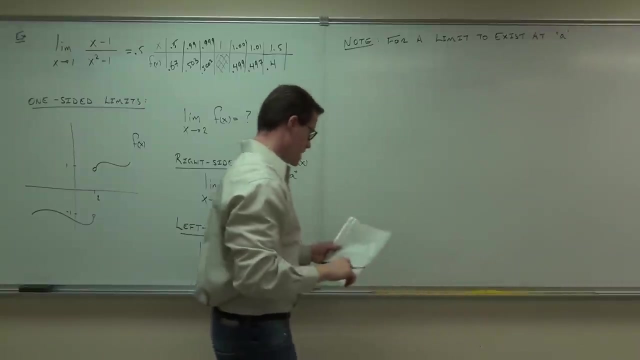 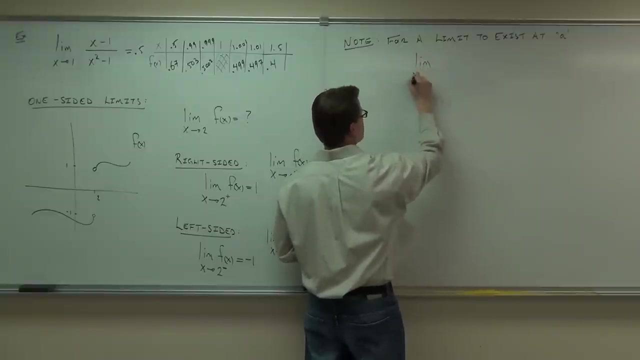 So let me write that out for you and I'll explain it. For a limit to exist at a point, we'll call it A. For a limit to exist at A, in other words, for this to happen, Okay, Okay, Okay. 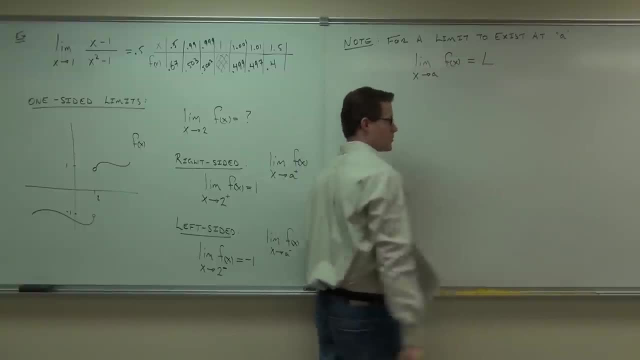 Okay For you to be able to say: the limit as X approaches A is some number. for that to happen, you must have this: The limit of F of X as X approaches A from the left must be equal to the limit of F of. 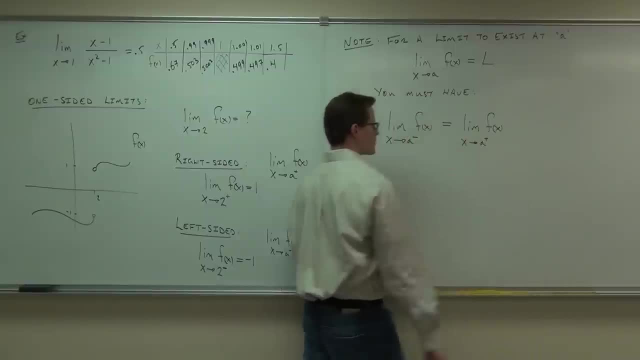 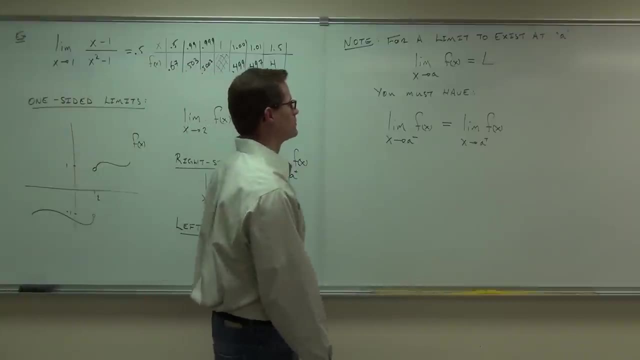 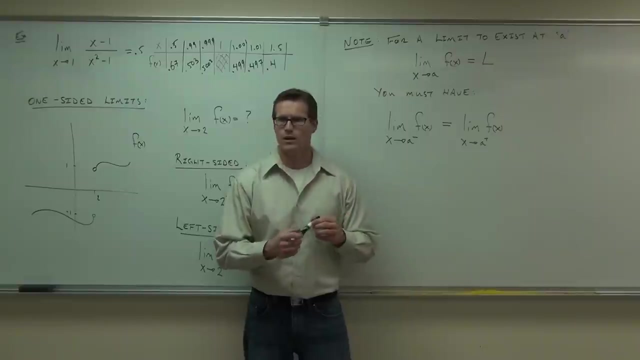 X as X approaches A from the right. It's got to happen. So let's see, if that happens, what it says in plain English. is this Ready for the plain English part? Here's the plain English. The function from the left and the function from the right have to have the same value. 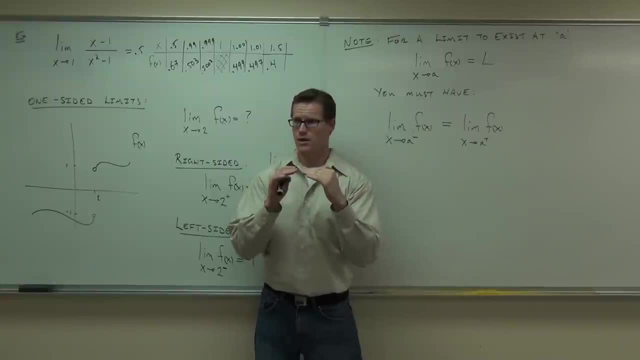 Basically, they've got to meet up somewhere. You with me on that. So let's check this out: Does the function from the right and the function from the left meet? from the left meet up? what do you think Do those lines meet up? 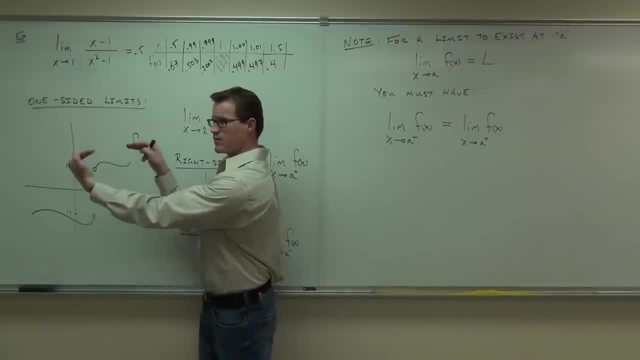 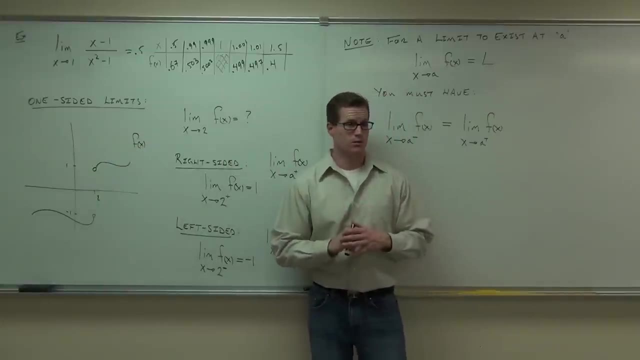 They do, they meet up, they come to the same point: Same value, same height. Well, let's see, This limit was one, this limit was negative one. Is one the same as negative one? So does both the one-sided limits have the same value? 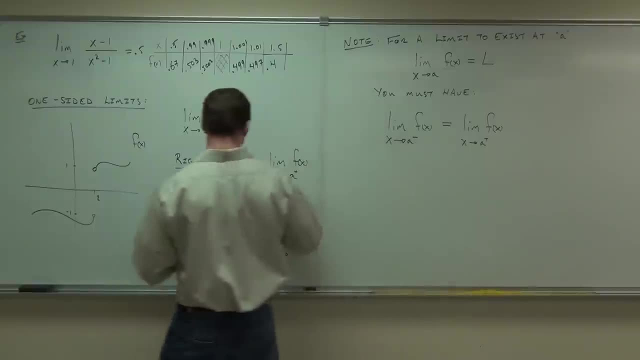 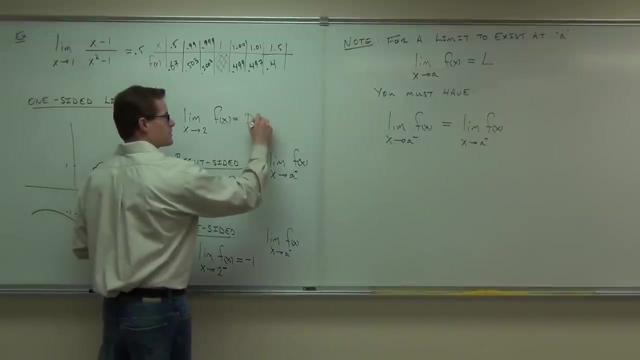 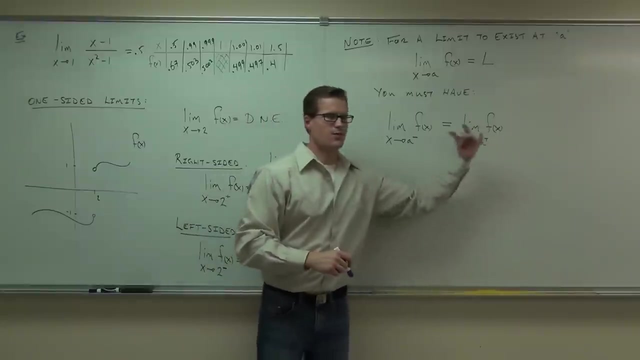 No, you'd say this limit does not exist. So we'd say the limit as x approaches two of f of x does not exist. This says why This says the limits from the left and the limit from the right must be the identical number. 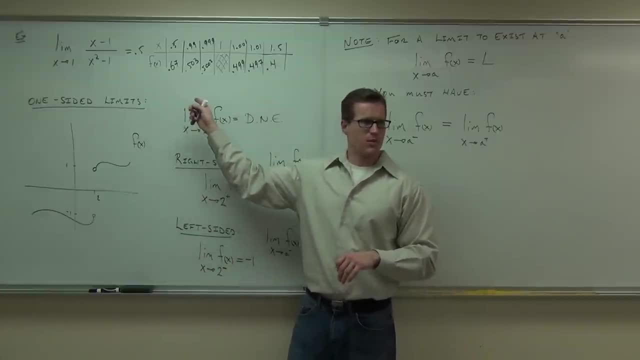 Remember this example? Look up here on the board. Remember this example. They said the limit existed because that's .5 and that's .5, basically It's coming to .5.. You with me on that? What if this was .5 and that was seven? 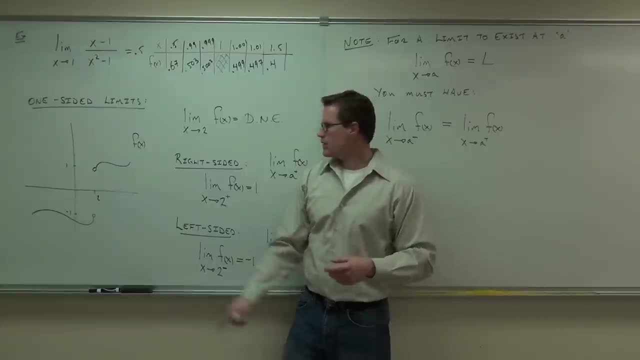 Would that be the same number? No, This one's one. this one's negative one: Is that the same number? That limit doesn't exist. It says that you have to have the same function value on both the left and the right, both. 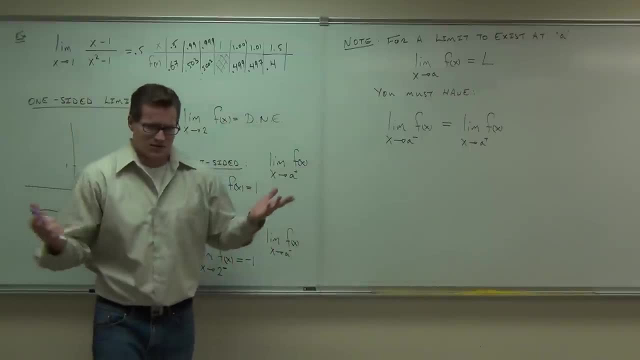 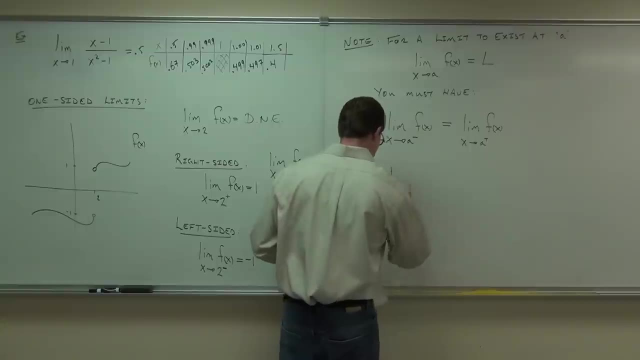 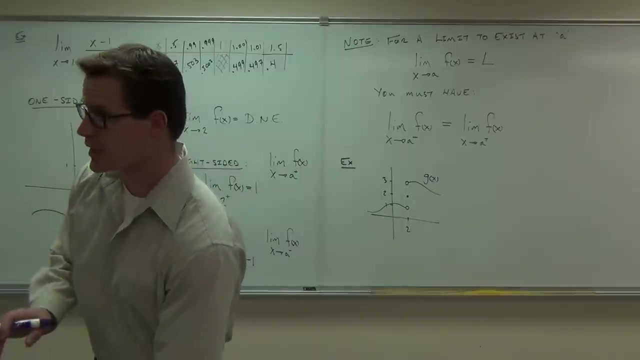 Would you like another example of this? Sure, Why not? It is long, We have time. Hmm, Let's practice. Let's do some good practice. If you're not getting it, I need some questions out of you, because you really do have to understand this before we go on to the next part. 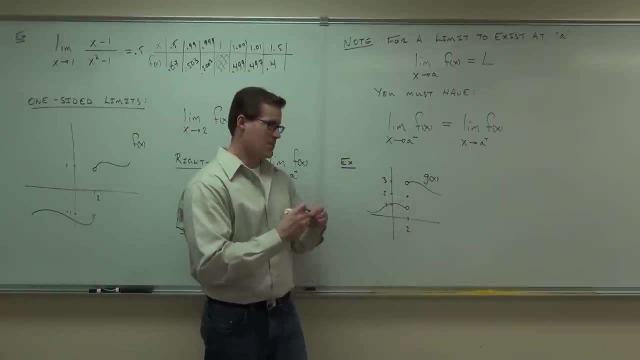 Let's practice before we go any further. so here's the idea: In order to find the limit at a certain value. in this case, we're gonna talk about two again. Do you see why? that would be the interesting case here? 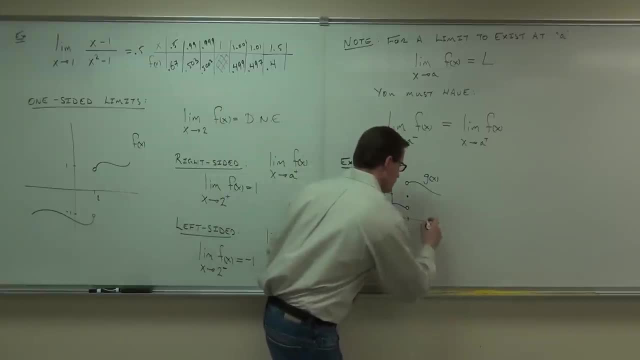 I wanna break it down to you all right, If I asked for the limit of three, it's not very interesting because look it, here's the value of three. Does the limit exist? at that point? The answer's clearly yes at three. at three, yeah. 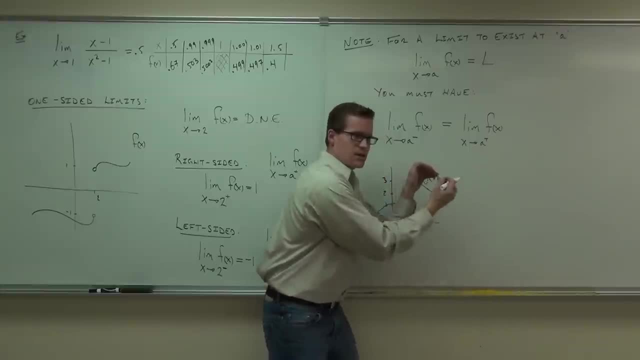 Look it, the function's there, the function's there, the function's there, it's all the same. Do you get me on that? That's not an interesting example. That's boring. They just said the function is completely there. 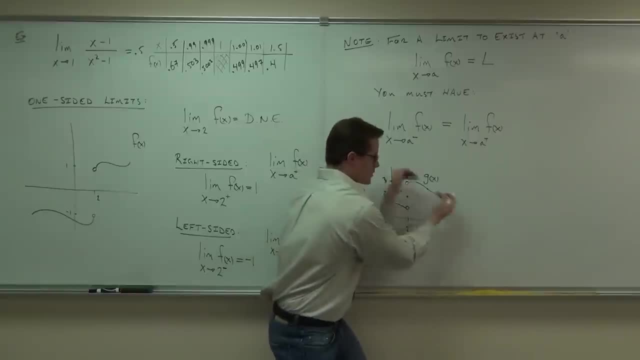 therefore, the limit must exist From the right and from the left. you're coming to the same exact point. Do you get me on that? That's not interesting. If I ask you about two, though, that's more interesting: You need to be able to find the limit from the right. 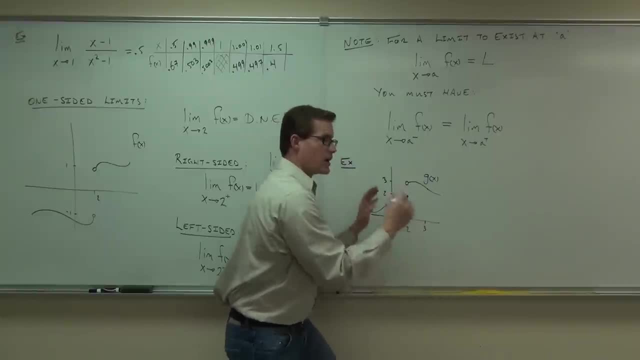 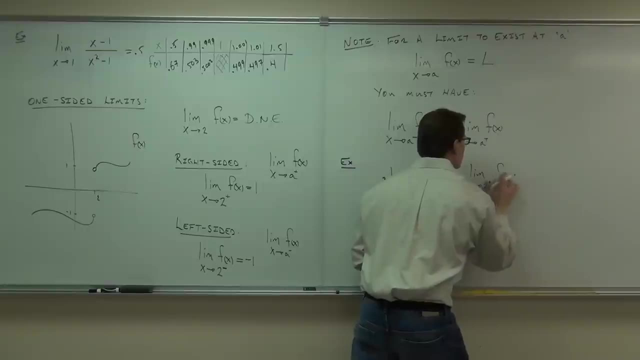 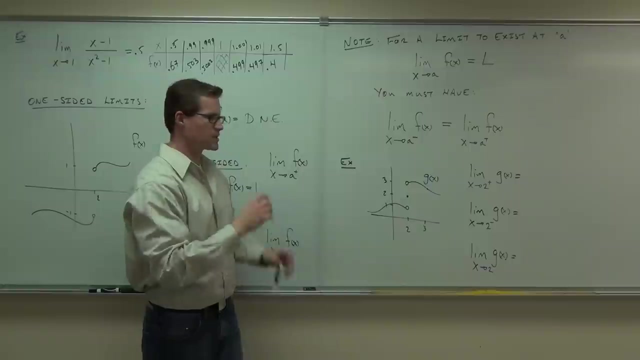 and the limit from the left, as we're approaching an x value of two. In math, that means this: Can you do this, Can you do this, Can you do this And can you determine this? Let's see if you can. 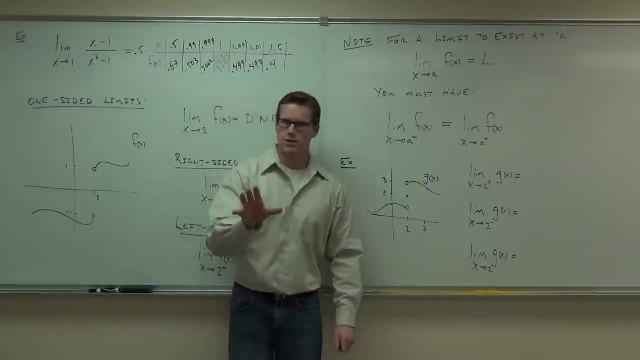 Let's see if you can. I'm gonna give you about five seconds between each problem to see if you can get it. okay, So right now, to determine on your own, can you tell me? don't say it out loud, okay, let everyone do this. 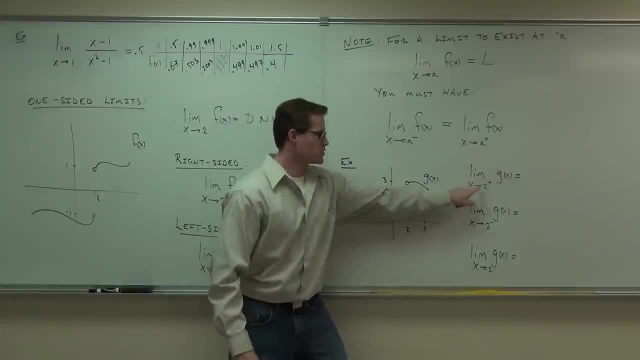 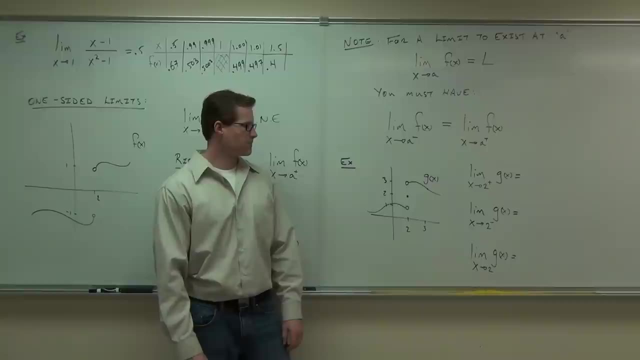 can you determine on your own the limit of g of x as x approaches 2 from the right? Do it on your own. don't say it out loud. Give it five seconds. The question in English asks this: what is the y value when x gets really close to 2 from the right? 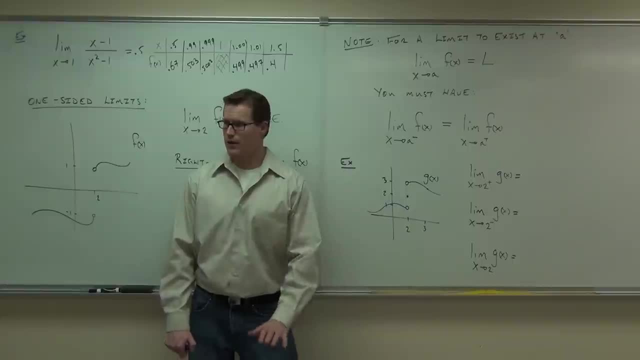 That's what the question asks. What is the function value or the y value when x gets really close to 2 from the right? Well, that was like four people answering. Do you all not know it, or do you know it? 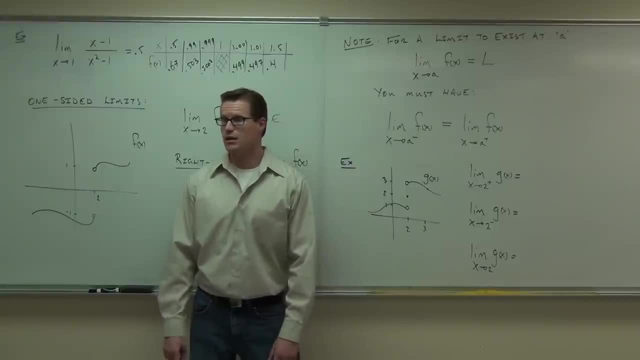 If you don't know it, then that's fine, but you need to tell me. If you know it, then say it. Can you find out that the function value, the y value, is about 3, or is getting close to 3, when x is getting close to 2?? 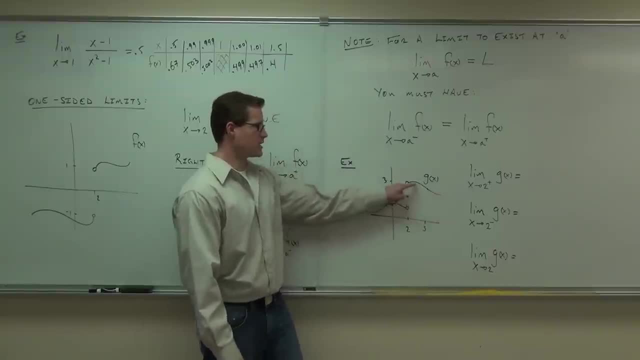 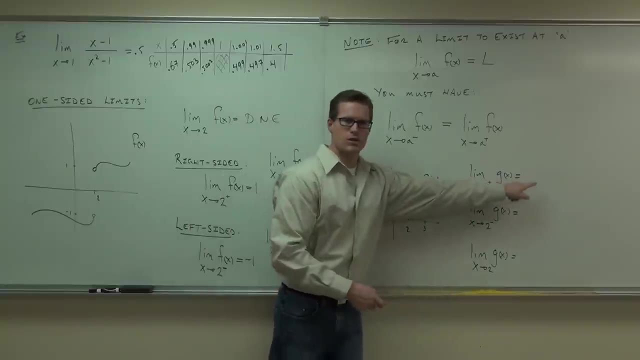 Can you see that, Because you're following this along, right, You're going. okay, what's happening? as I'm getting close to the value 2 along the x, The y, The y is getting close to 3, so this is how much. 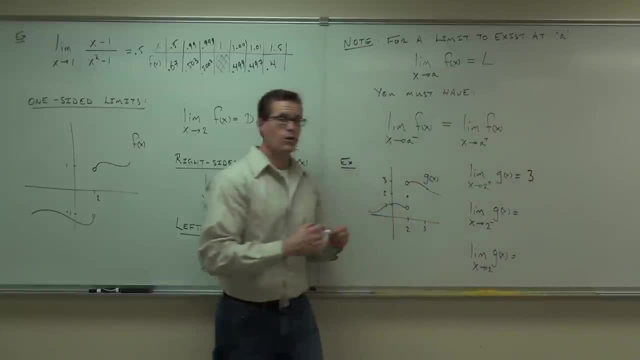 3. Okay, now I want you to do this on your own. don't say it out loud again. Find me the limit of g of x as x approaches 2 from the left. Write it down on your paper. don't say it out loud. 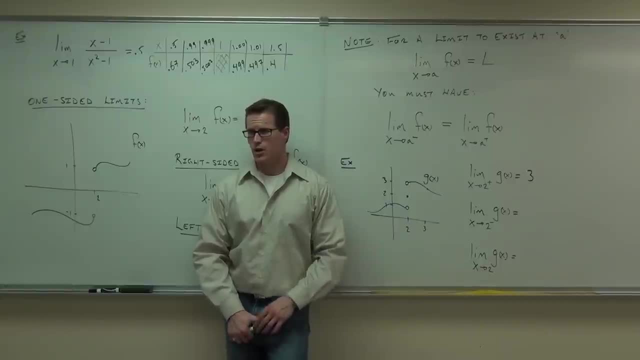 From the left. Basically in English that says: what's the y value when the x value is getting close to 2 from the left? Starting from the left, What's the y value when the x value is getting close to 2 from the left? 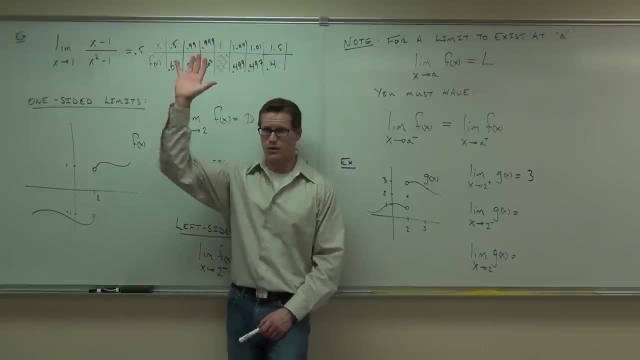 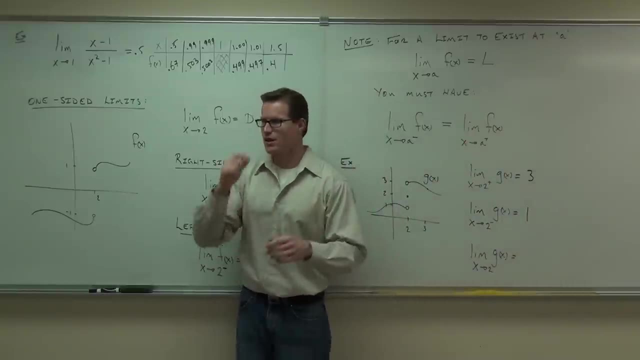 1. 1. 1.. Did y'all get 1?? How many of you were able to find 1?? Good, okay, Here's how you tell if the limit exists or not. Here's how you tell You. look at these ones. 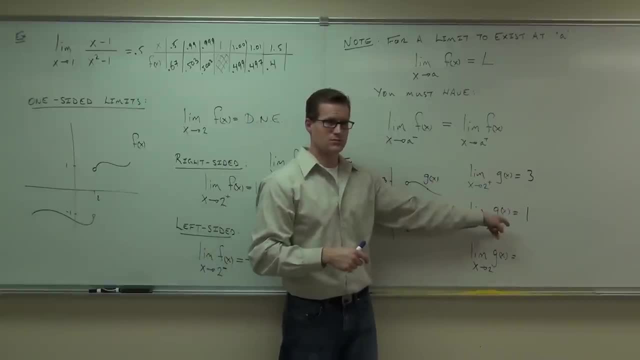 Are they the same? No You sure? Yeah, 1 is 3,, 1 is 1.. I mean, how much more sure can you be? If those aren't the same, does that exist? If those are the same, does that exist? 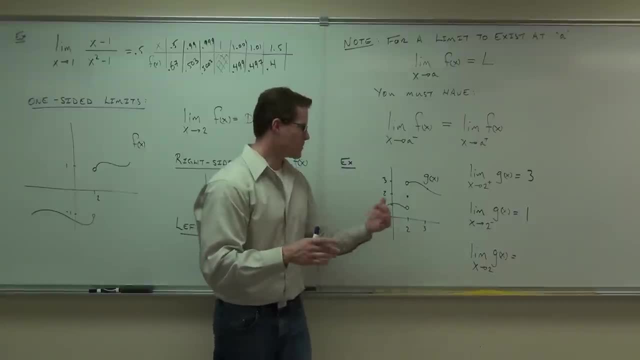 Yeah, I want you to know something really cool. I want you to know something really cool too about limits. Does it matter at all that that point was right in the middle of nothing? We don't care about that point. We don't care at 2.. 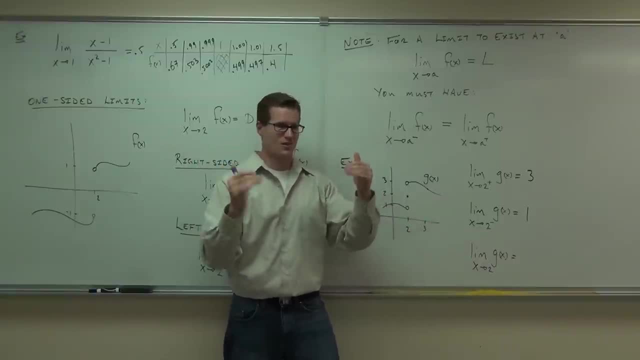 We care what's happening to the function as we're getting close to that. You see the difference. I don't care about that. It could as well not even be there, It doesn't matter, We don't care about that point. We care about the function value, the y value, as we approach the x value. 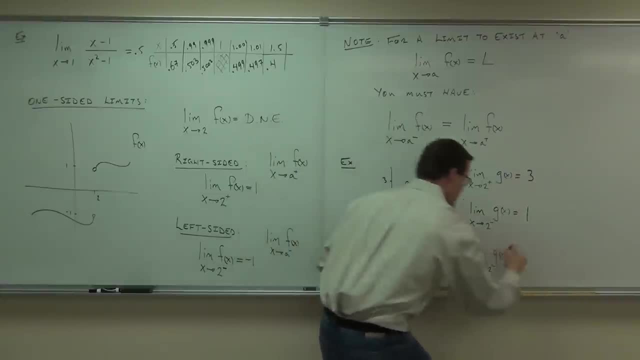 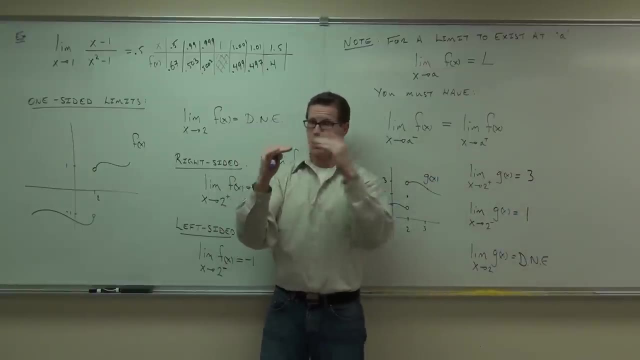 So if this does not equal that, does that exist? Can you put gain? You can really see it, though, can't you? If the lines don't match up, It's not there, It's not going to happen. The limit doesn't exist. 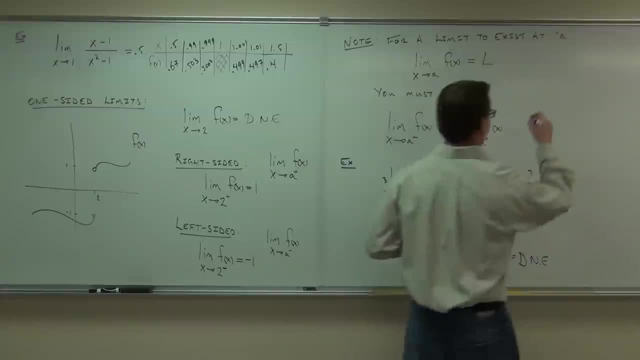 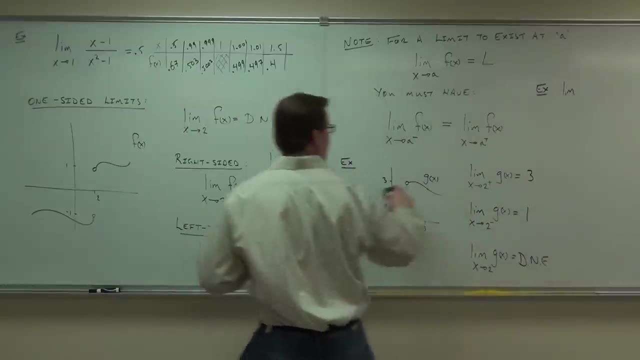 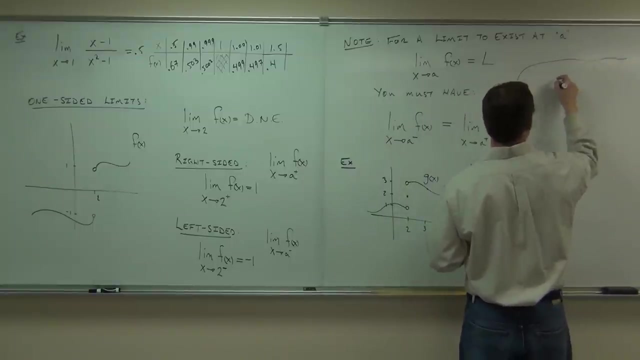 Let's do one more and we'll call it good on this stuff. Here we go: Let's do one more and we'll call it good on this stuff. Let's do one more and we'll call it good on this stuff. 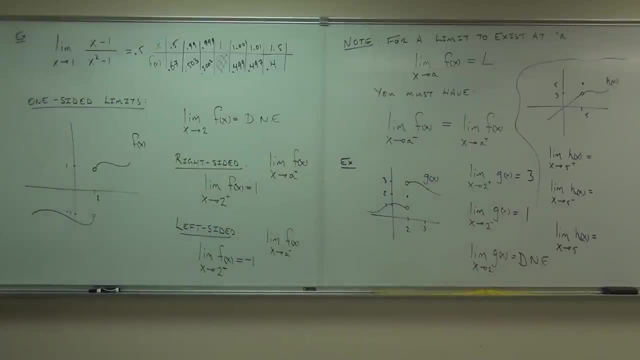 Okay, last picture, Last picture for us. I want you to try to do that one completely on your own. okay, This is h of x. I want you to find the limit of h of x as x approaches 5 from the right. 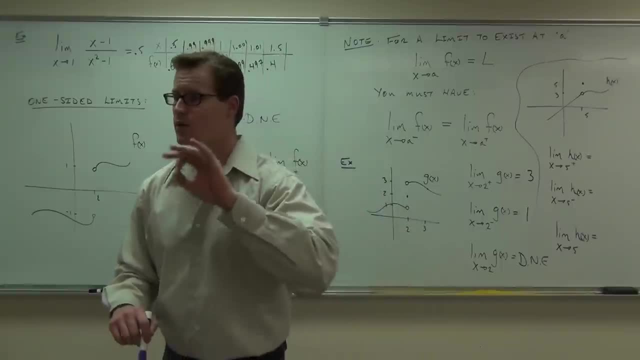 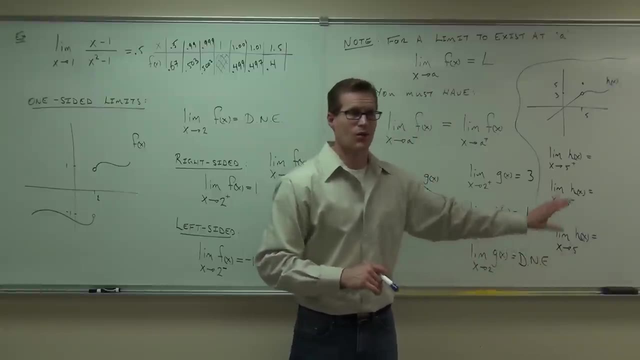 I want you to find the limit of h of x as x approaches 5 from the left, and then I want you to determine whether or not that limit exists at x equals 5.. Do you follow the questions? Okay, go ahead and do that and see what you get. 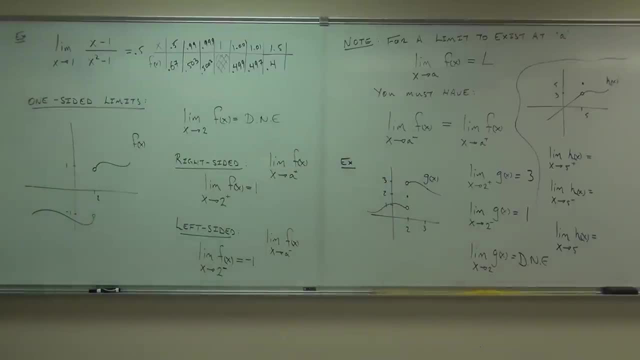 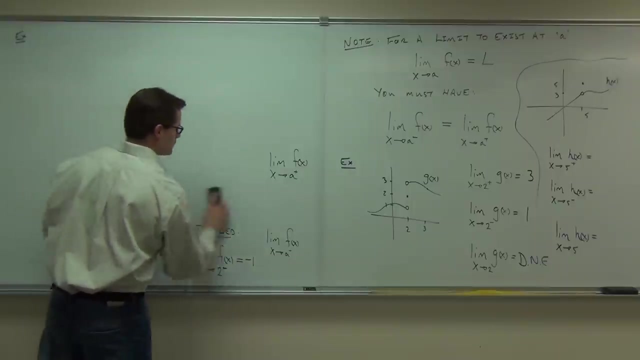 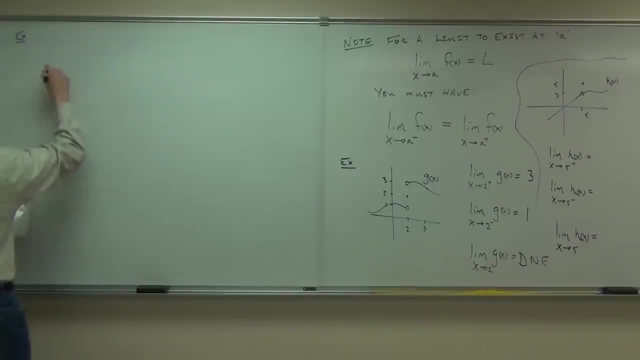 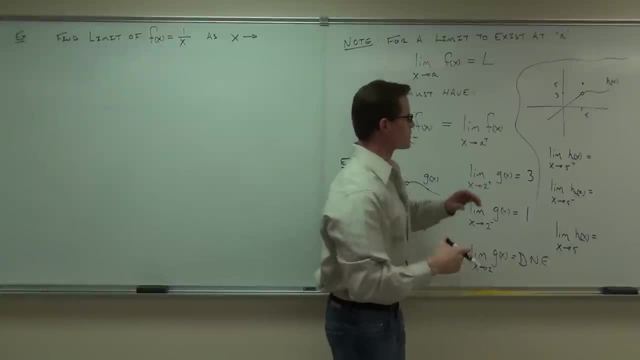 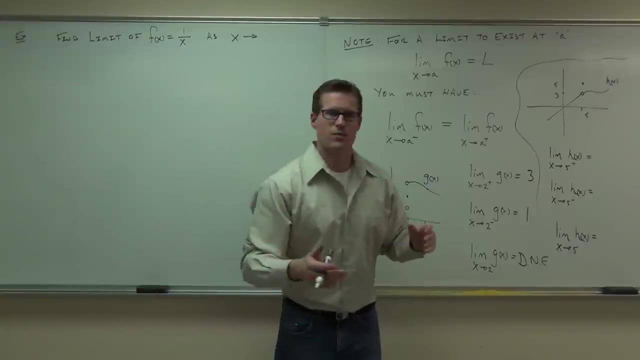 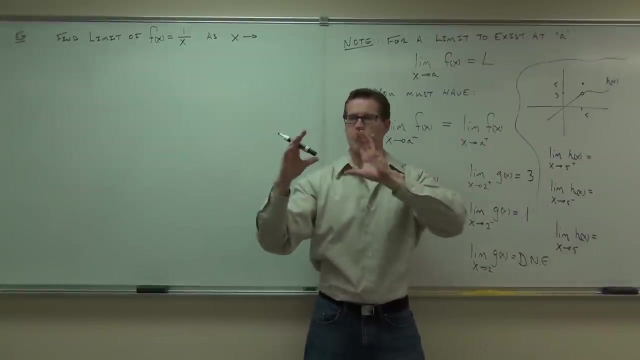 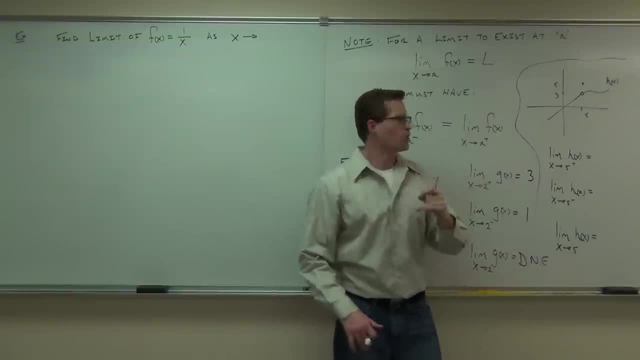 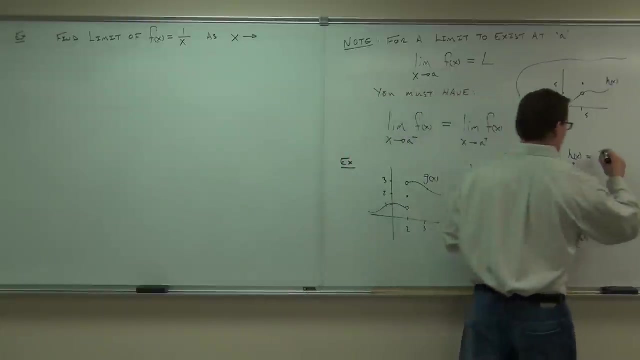 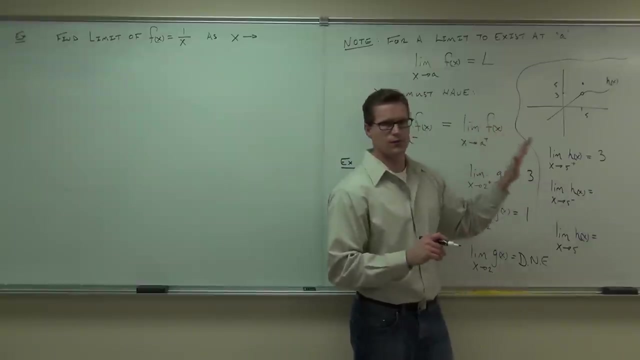 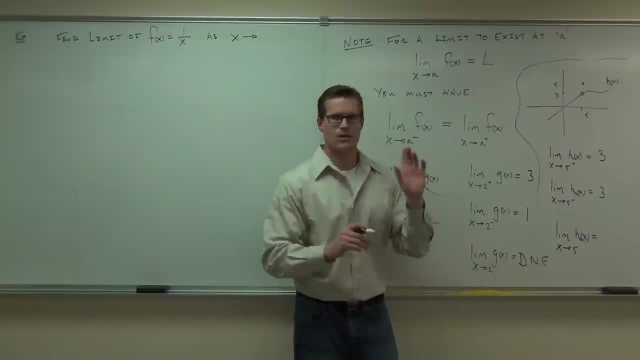 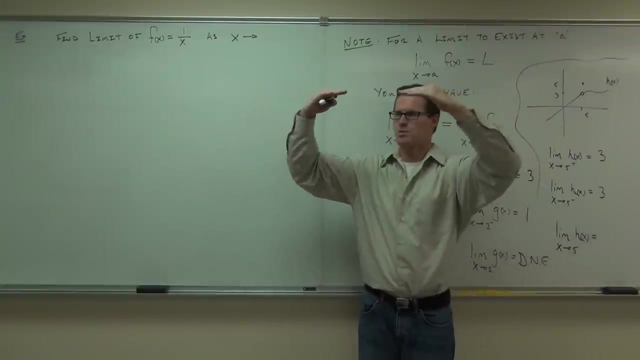 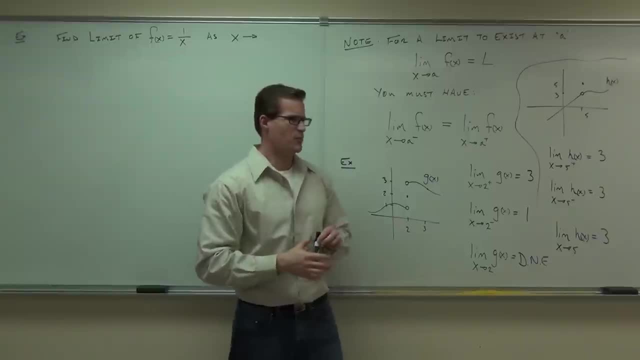 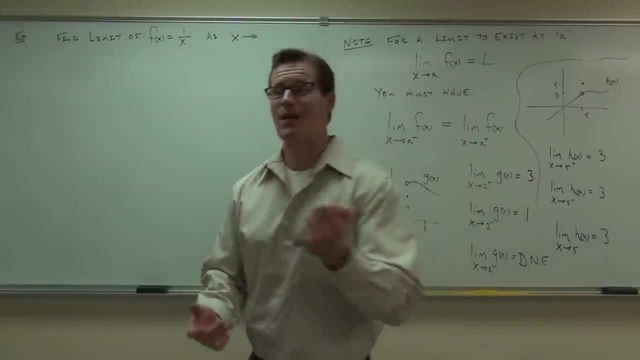 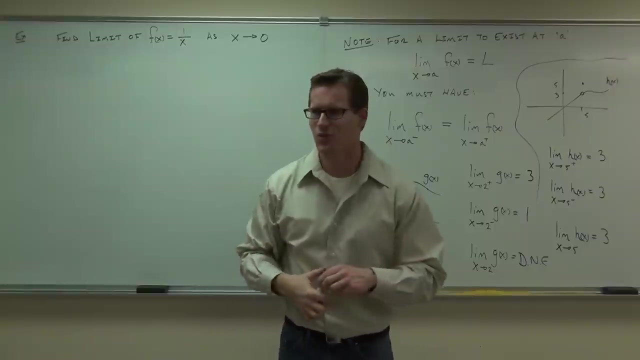 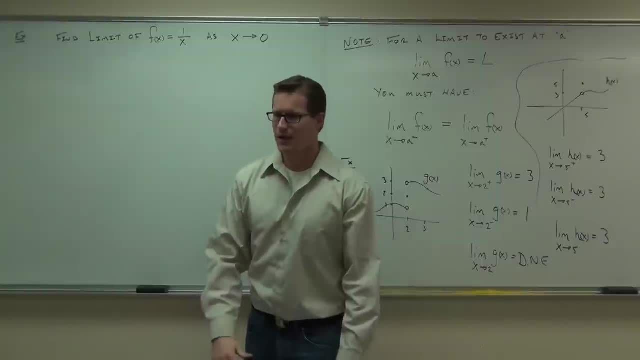 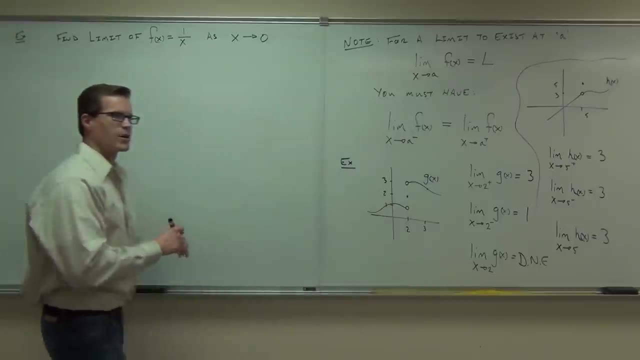 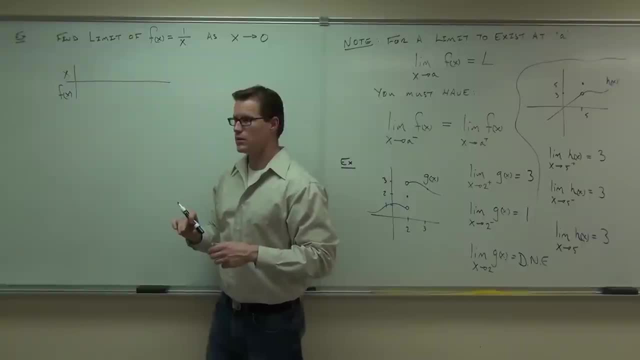 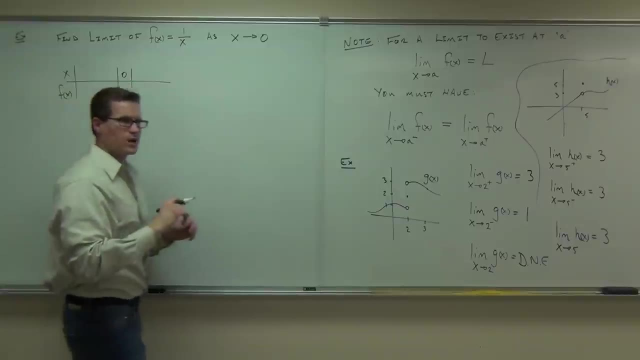 Where does the zero go on our table? To the left, to the right or in the middle Middle, Because that's the number we're trying to get to. Are we ever going to be able to get to the zero? No, 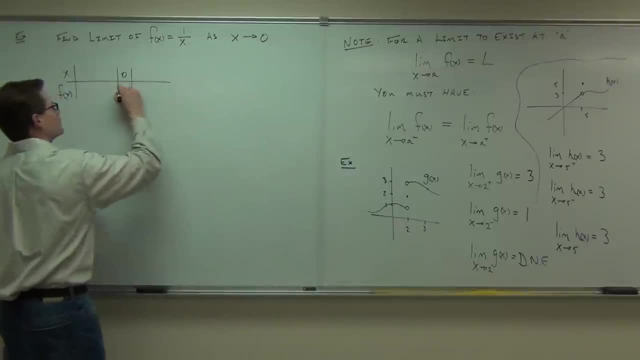 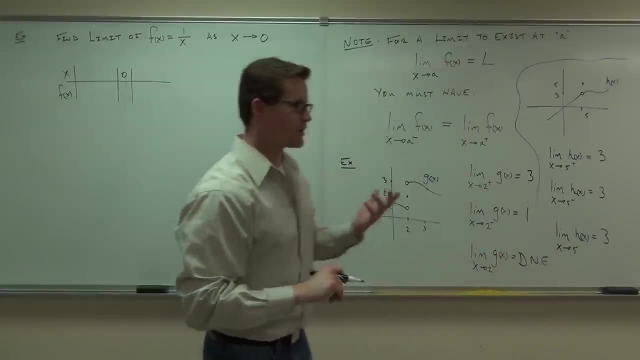 No, we can't plug it in because then it's undefined. That would be a problem. So Now let's pick some numbers that are getting close to zero from the right. Let's start at like: oh, I don't know, .5, and we'll work our way down. 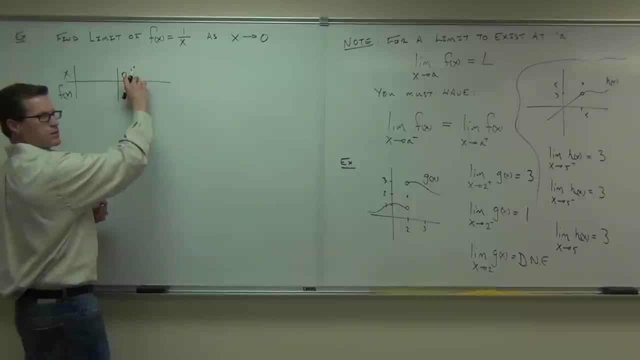 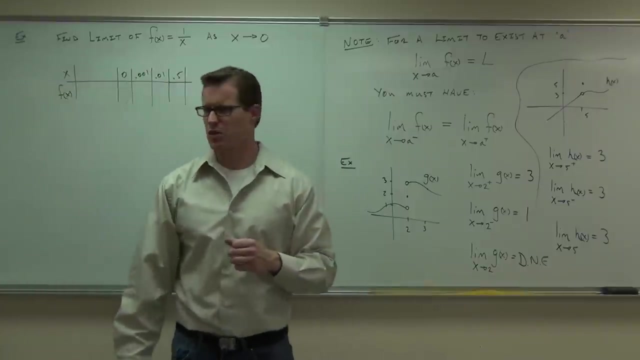 So .5,. is .5 supposed to go here or here, The right or the left Right, Right Right? So .5,, all right. .01, and .001, would you agree? those are numbers that are pretty close to zero. 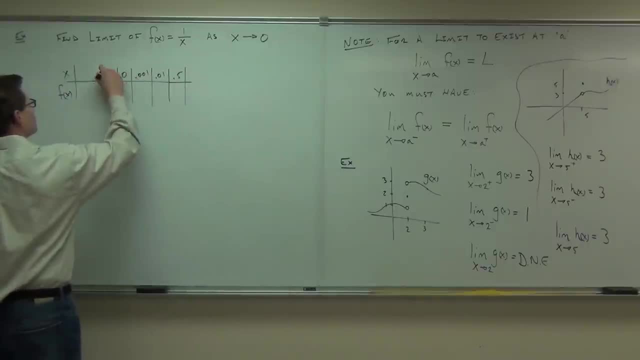 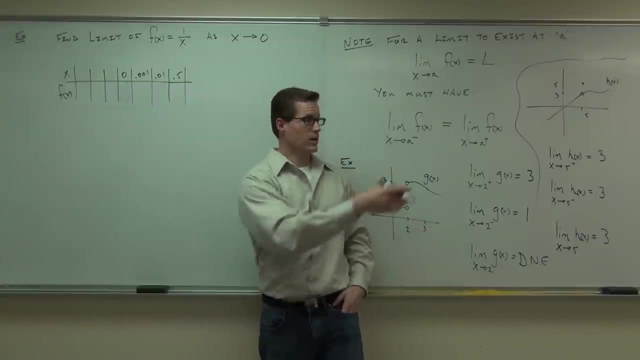 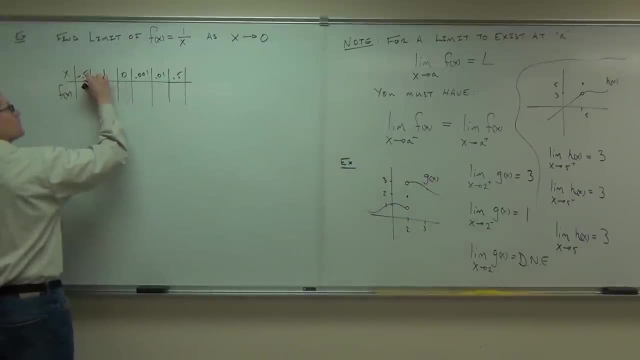 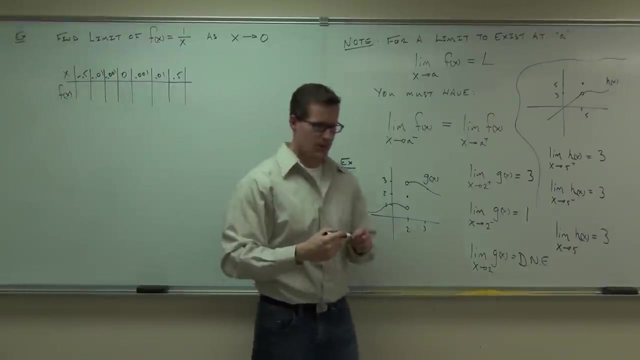 So negative .5,, that'll work, And negative .01, and negative .001.. So let's use those numbers Again. left side people do left side, Right side people do right side. These ones should be a little bit easier to plug in, yeah. 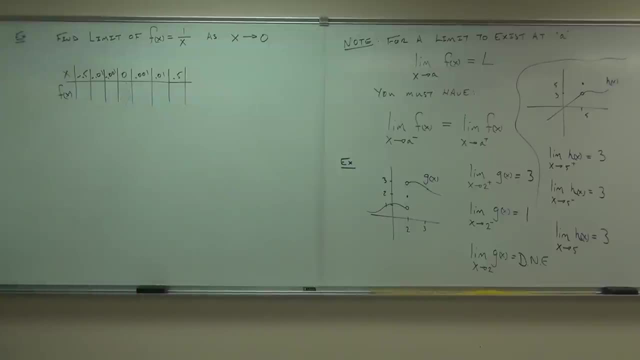 By the way, this is going a little bit out of the scope of this section. at this point, We're talking about something a little ahead of time. It's interesting to me, so we're covering this right now. It will come back at us later on, right? 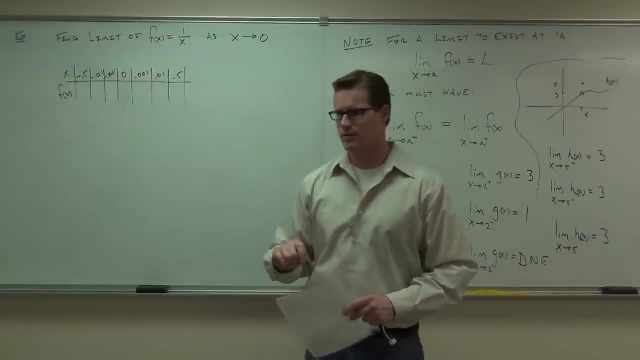 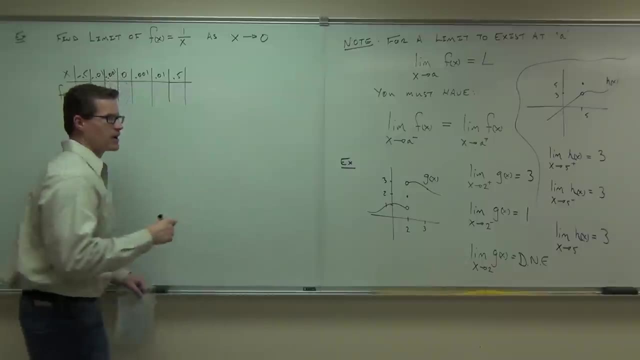 But I'd like to make sure you see it in limits at least once or twice before we get to that section. So if you take 1 and you divide it by 0.5, I'm hoping that you got 2.. Did you get 2?? 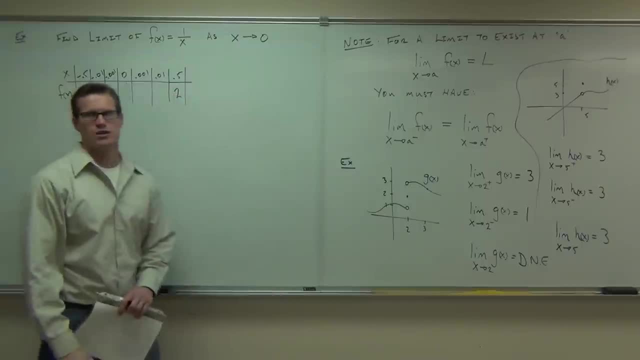 And over here you probably got- well, I'm going to be a genius about that- negative 2.. Did you get negative 2? No. Did you say 0? No, I divided it by 0. Okay, good. 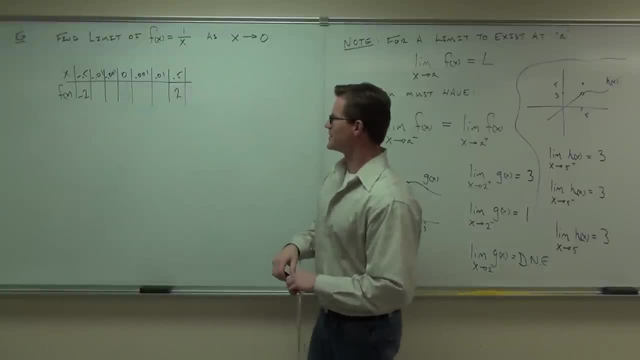 I scared myself for a second. So 2 and negative 2, very good. Now how about 0.01?? If you divide 1 by 0.01, you should get. let's see, move the decimal place. 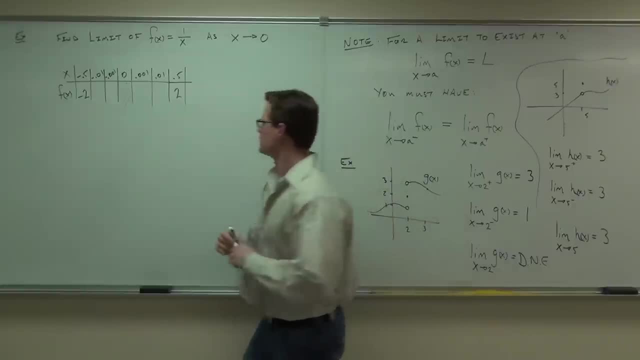 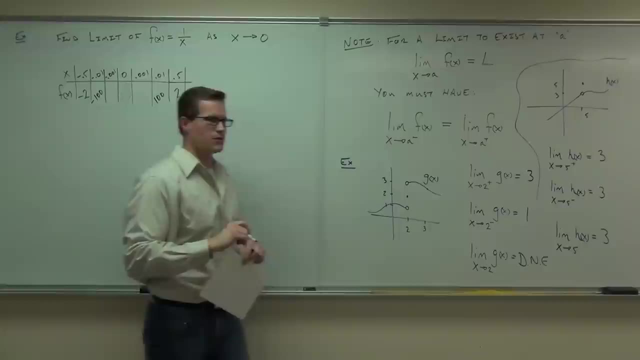 You should get 100. And I'm going to hope this is negative 100.. Yes, If you divide by 0.001, that's let's see 1,, 2, 3 decimal places, You're just dividing 1 by decimal places there, ending in 1.. 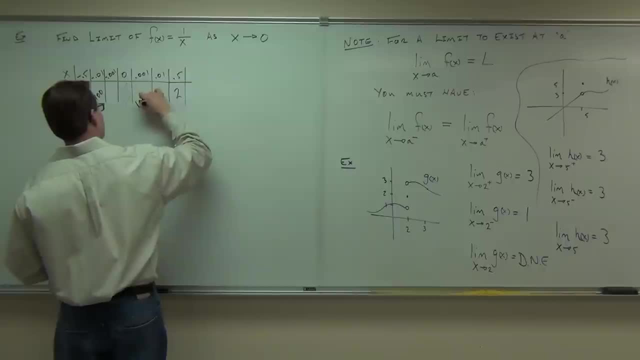 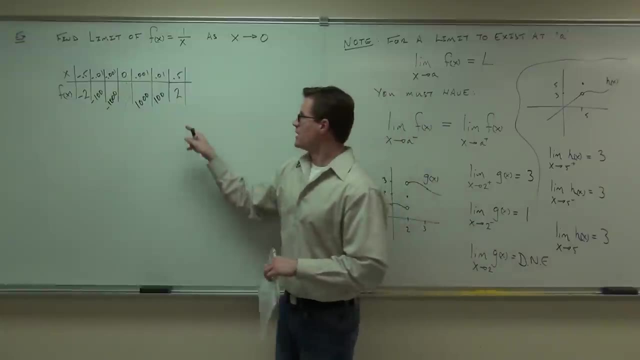 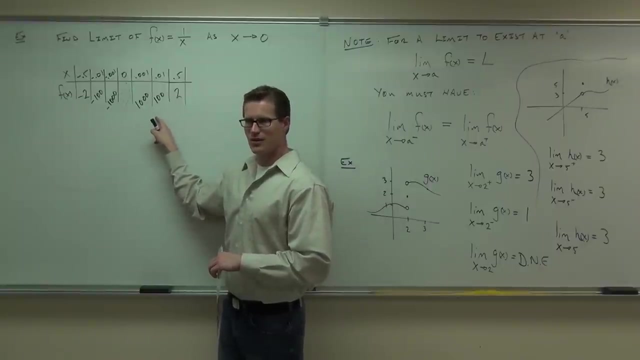 This should be. Let's do a little critical thinking here, all right. First question is: is this number getting bigger or smaller As we're approaching 0 from the right? Is it ever going to stop getting bigger? 1 divided by 0.00001 is going to be really, really, really, really, really big right. 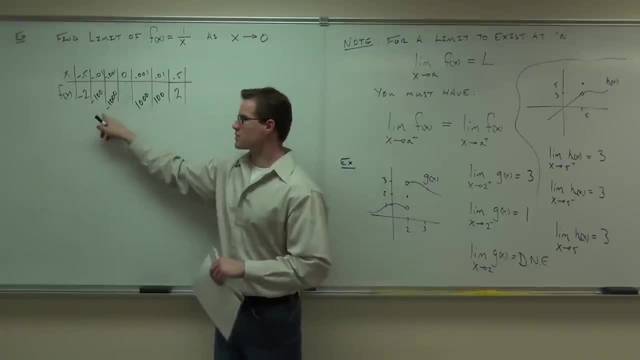 And it's going to be positive. How about this way Is it getting bigger or smaller? Way smaller, And it's never going to stop getting smaller. It's not going to a certain number. Now the second question is: does the limit exist? 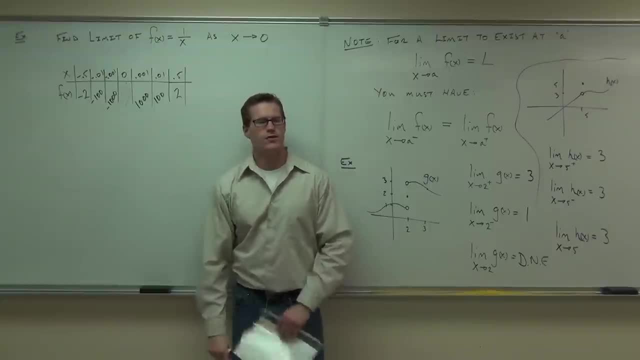 Are they going to the same exact number? No, in fact, as we're going from the right. where would you say this is going? Because if you draw the picture, it's going like that. It's going where Infinity If you divide by smaller and smaller numbers that are approaching 0,. 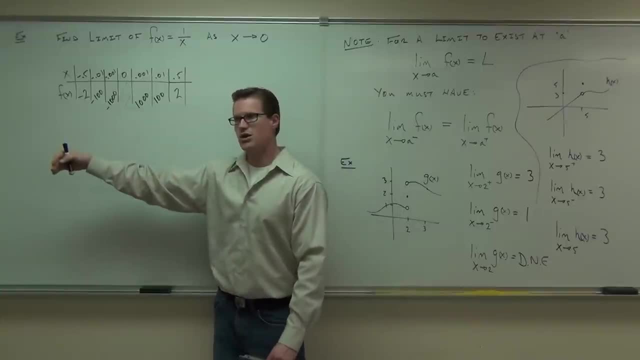 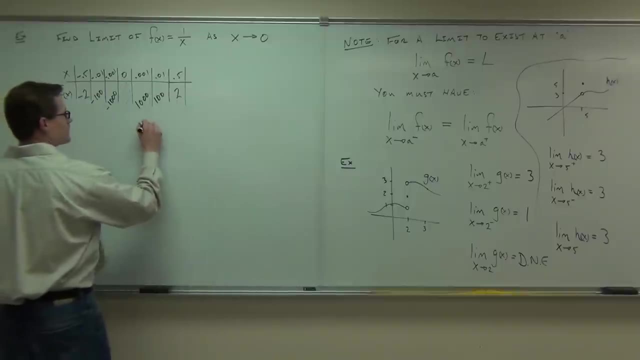 keep dividing by 0.000000 forever, and then a little 1, you're going to get really, really huge numbers, right? And you can keep getting smaller and smaller still. So what we would say is the limit as x approaches 0 from the right of our function. 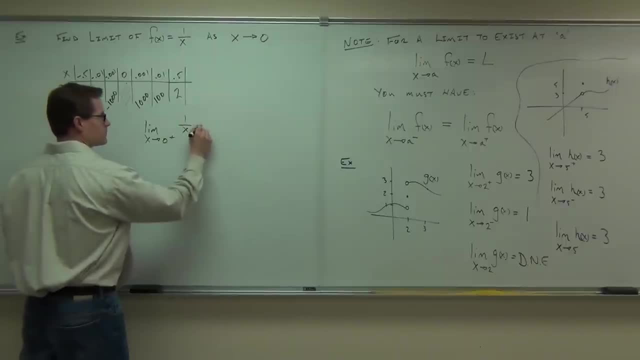 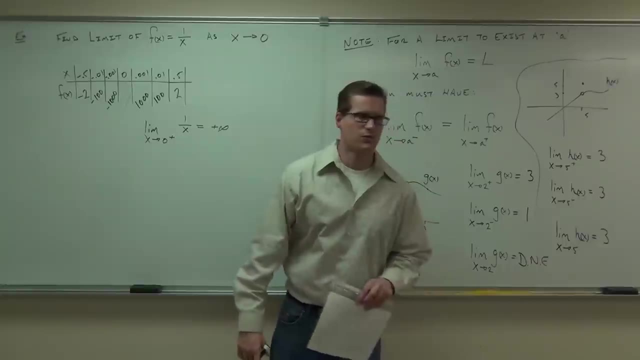 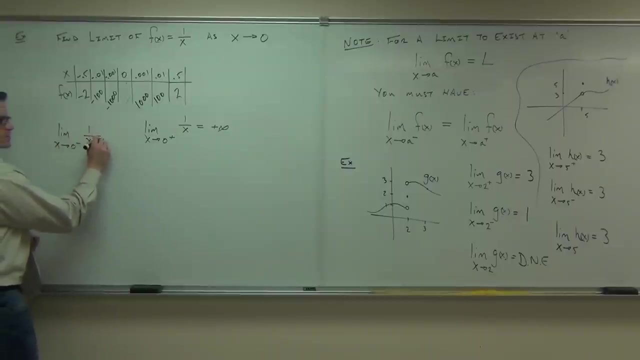 which is 1 over x is positive And you technically don't have to put the plus, because infinity without that plus still means positive infinity. but I want to show the difference Limit as you approach. I'm sorry, as x approaches, 0 from the left is. 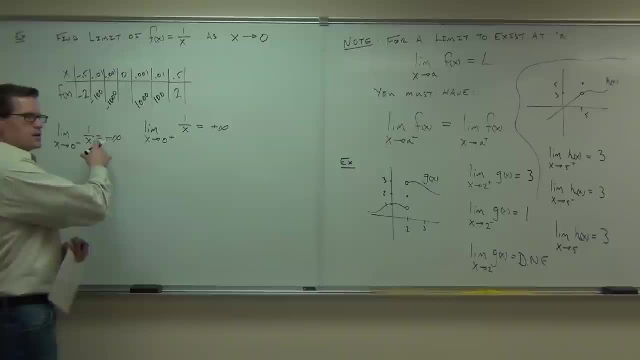 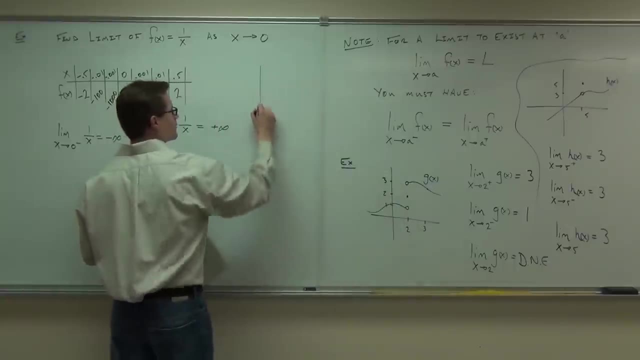 what would you say that would be, Is negative infinity the same thing as positive infinity? So limit clearly doesn't exist. In fact, you can see this from the graph. If you graph 1 over x, your calculator, you graph it on a similar way, like this: 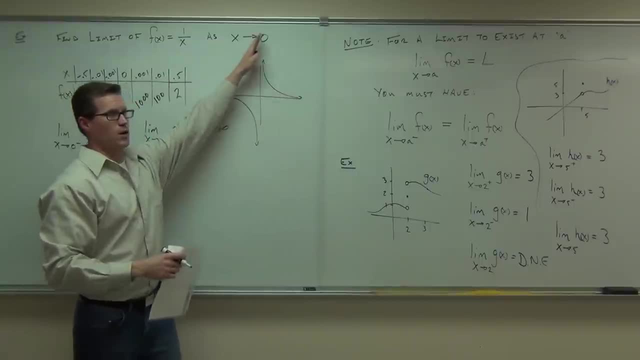 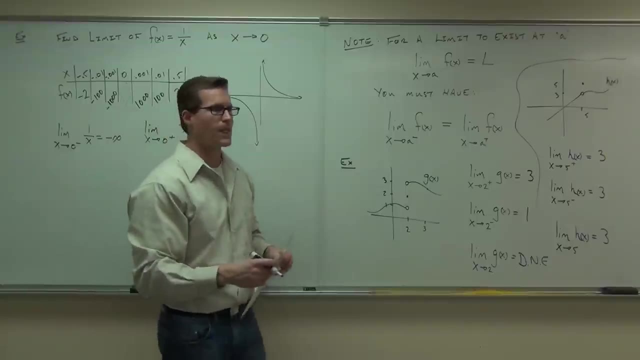 That's it. You can see, as we get towards 0, it's skyrocketing. As we get towards 0, it's really going into an abyss, right. So it's not going to be the same thing. But this leads us to a couple ideas. 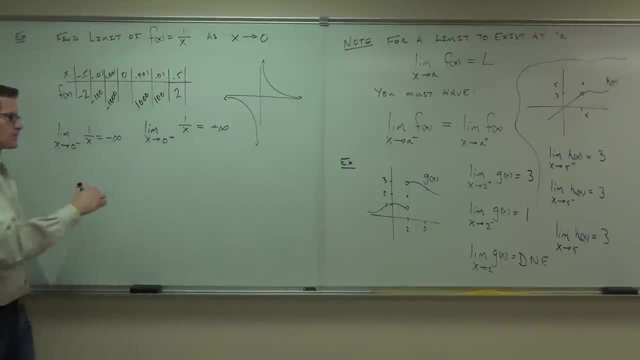 Whenever we have a limit, I'll write this out for you. If you have a limit, as x approaches a from either the right or the left of some function and you figure out that it's positive or negative infinity, I'll say it again. 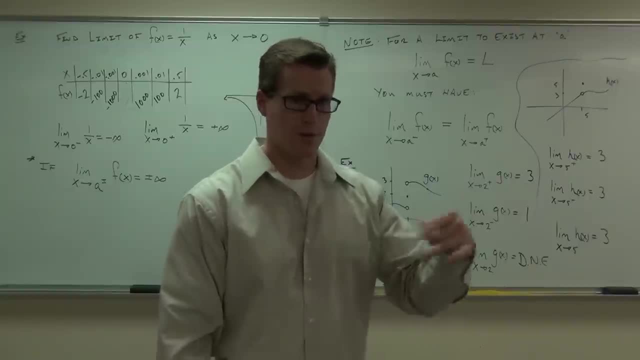 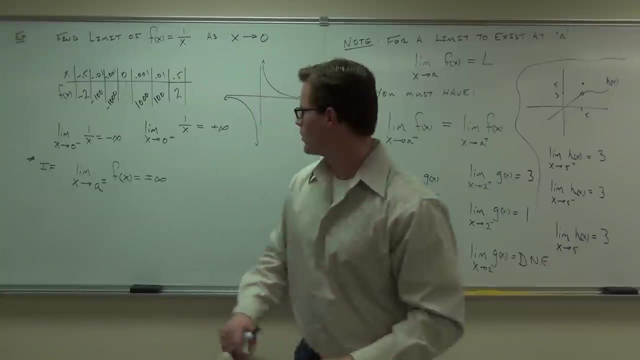 If you are approaching a number right from either the right or from the left, and it's going to infinity, either positive or negative, what that does for you is: it gives you an. what's this thing called? It gives you an asymptote. 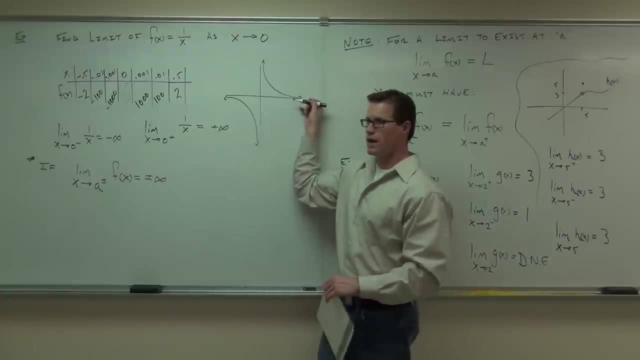 It gives you an asymptote, Because you say, okay, if we're going towards infinity as we're reaching- as if my y value is going to infinity as my x value reaches a number, that means I have to be shooting up. 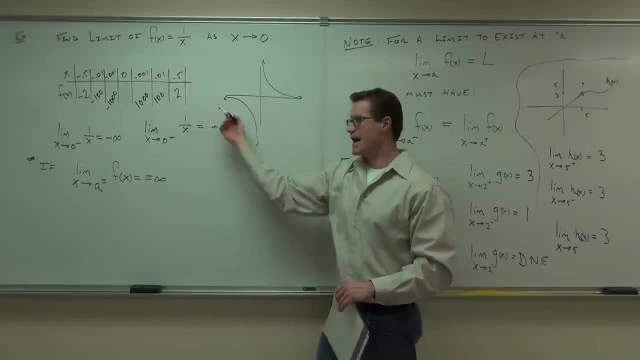 If my y value is going to negative infinity as I reach a certain number, that means I have to be shooting down. So one of those cases it's going to be some sort of asymptote. You're never going to actually get to that point. 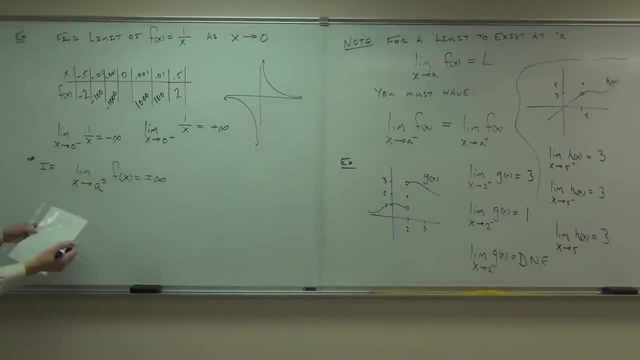 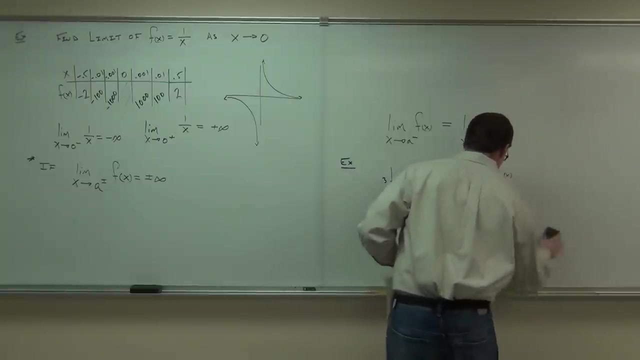 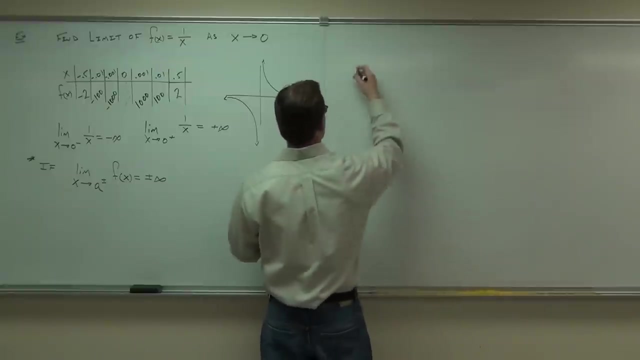 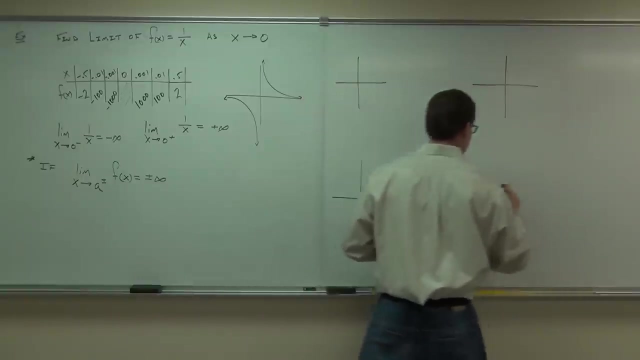 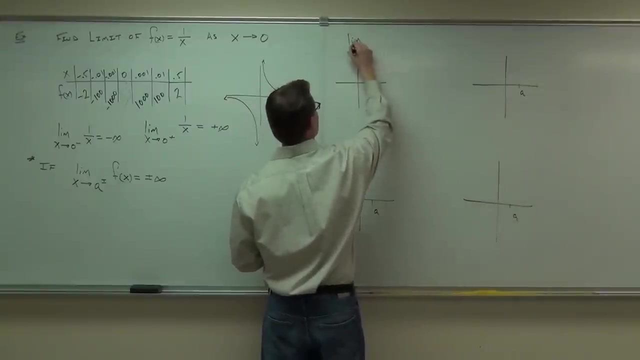 You can't, You can't. So there are really four cases. I'll draw them over there so you can see them: Four cases of asymptotes and their relationships to their limits. So the one case is what happens if we approach a from the right. 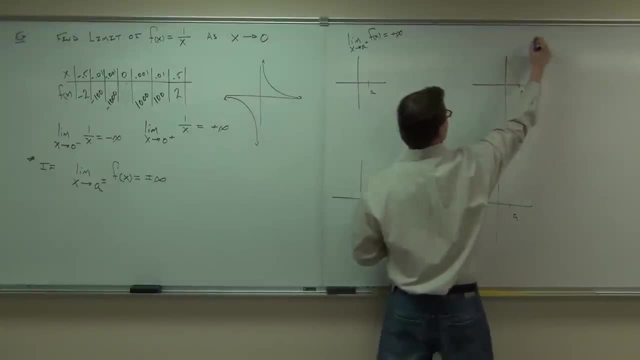 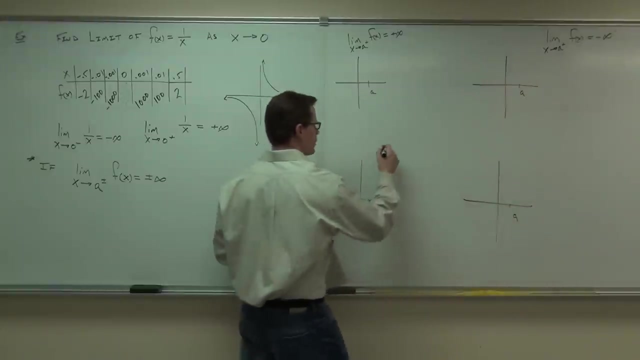 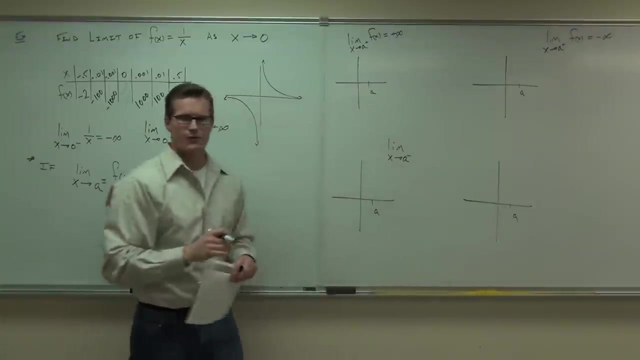 and we're going to positive infinity. Another case would be what happens if we approach a from the right and we go to negative infinity? Another case would be: well, what would happen if we went, if we did- the both rights, right from the right, if we went to a from the left? 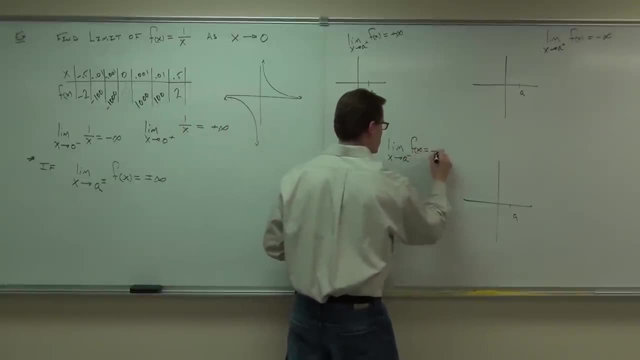 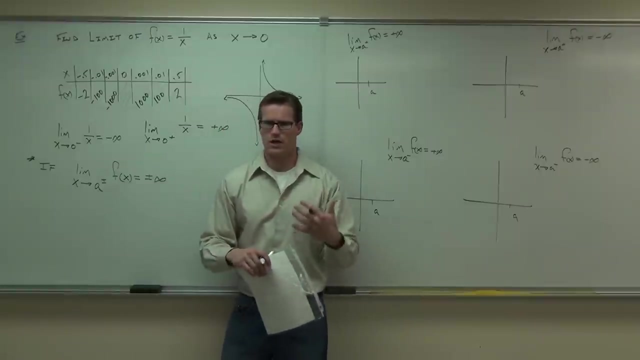 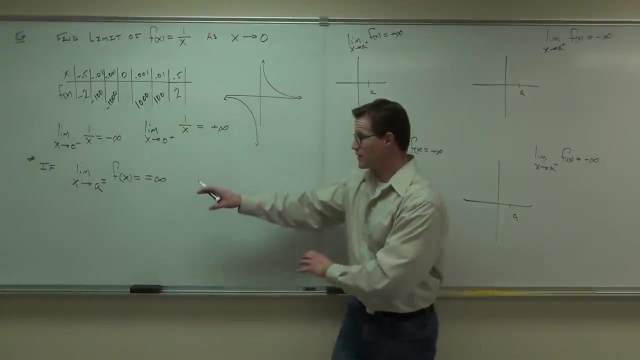 and went to positive infinity? or what would happen if? if we went to a from the left and it gave us negative infinity, Would you agree? those are all four permutations, all four cases of this. In either case, we just talked about this- if your function is going to positive infinity, 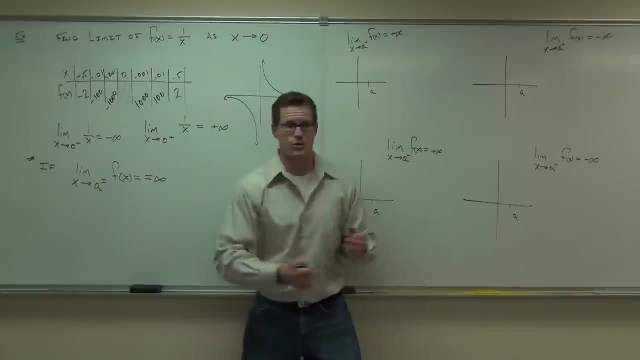 when x is going to a from the left or the right, you're going to have an asymptote. So every one of these is going to be an asymptote. Oh, that's the worst asymptote I've ever drawn. That's the one we've got to experience. 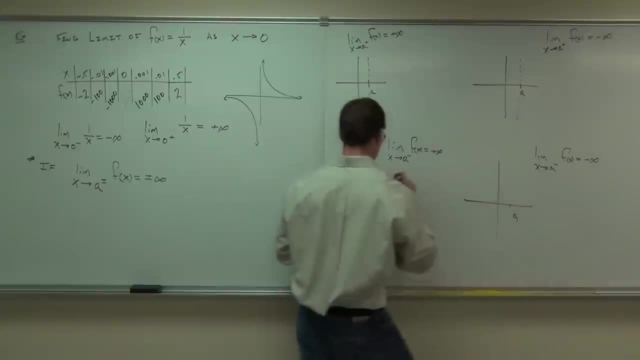 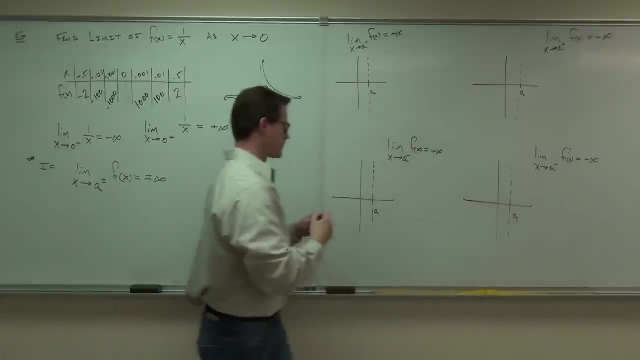 That's the second worst. Oh, that's not bad. That's not bad. Let's kind of diagnose what these things would do. I want you to really think of what these limits should do to our function here. OK, Now, if I say x is approaching a from the right, 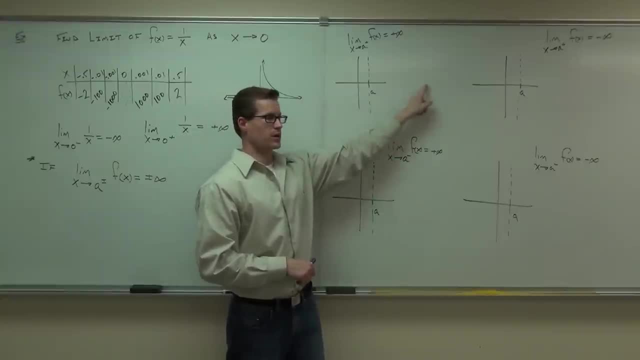 should I start with a from the left? Should I start with a from the right? Should I start here or start this way? Am I going this way- option one- or this way? option two: Option one: So if the function is approaching a from the right and it goes to positive infinity, 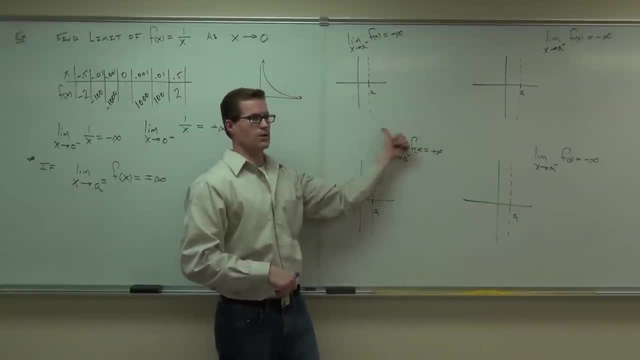 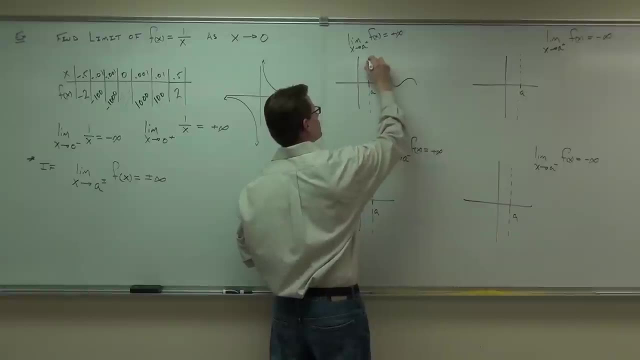 should I be going up or should I be going down? So this would be this type of graph. It can do whatever it wants over here, No problem, but when it gets to here it shoots up. This is not going to be. this isn't going to. 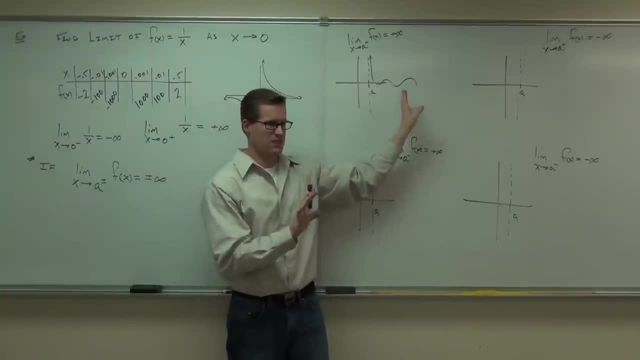 this isn't going to be told by our limit as we approach a. all right, It has nothing to do with it. It's what happens as we get close to a. It's going to be going towards positive infinity. Let's talk about this one. 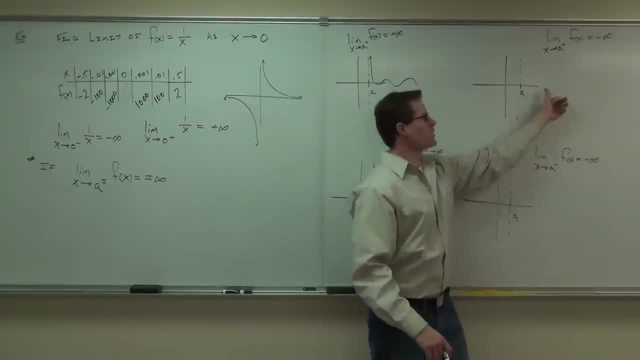 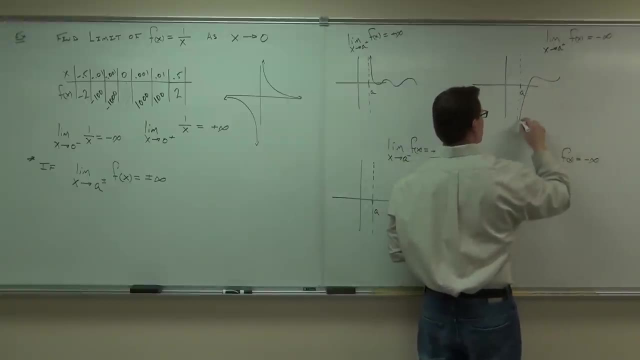 Now I know we were just coming from the right-hand side. This one's going to be going well, not up, not positive infinity. It's going to be going down- negative infinity. Do whatever you want over here, but it's going to drop. 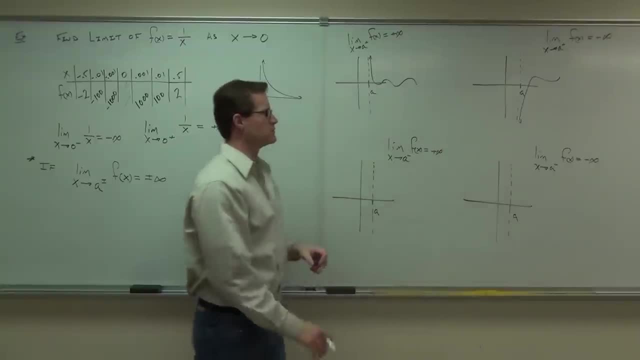 It's going to be asymptotic to that line. How about this one? Can you picture what that one does in your head already? Draw a graph if you want to. right now You should be able to draw something with that. Are we going option one from the right or option two from the left? 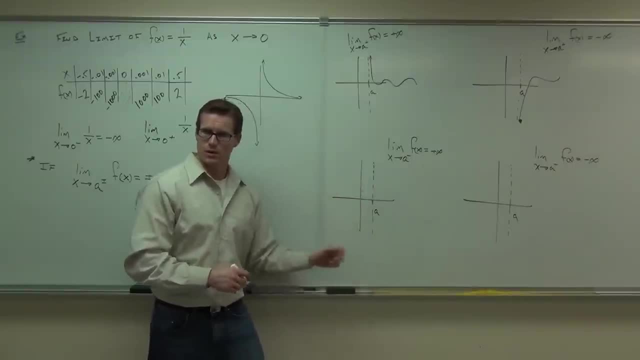 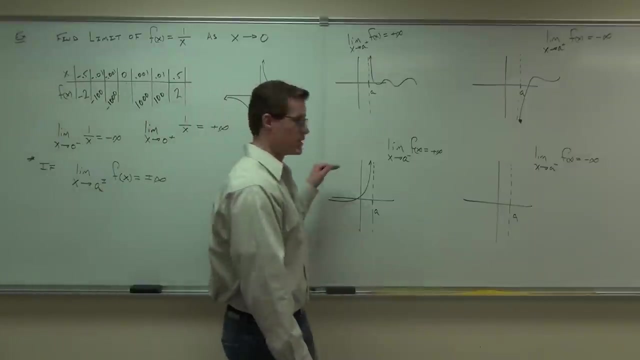 From the left, and should we be going up or down? Which one Up? It's going to positive infinity. up or down? Up? Lastly, the only case we have left is from the left going down to negative infinity. It looks something like that: 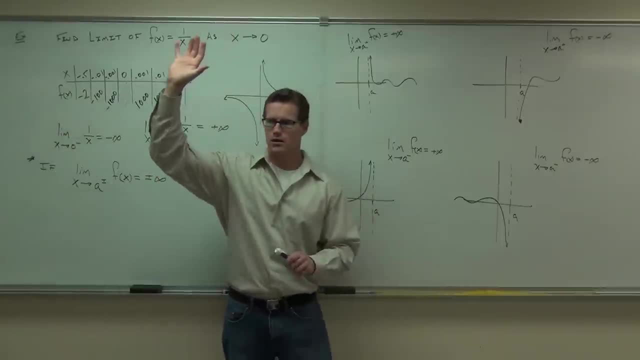 Would you raise your hand if you feel okay with what we've talked about so far today. All right, That takes care of, kind, of our introduction to limits. We talked a little bit about that. Now for the rest of our day, I'm going to teach you how. 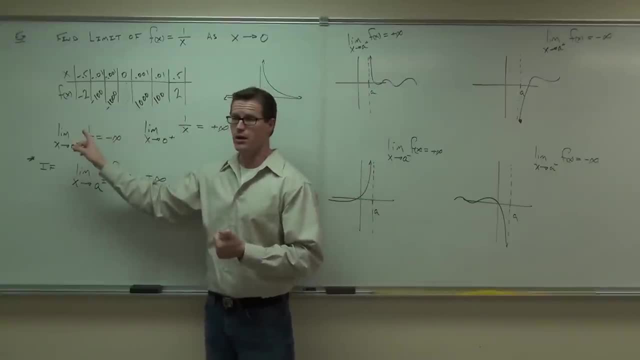 to compute limits, Because, if you hadn't noticed, this isn't all that fun. I'm going to show you some better ways on how to do that. Would you like to learn that? Cool, Any questions before we go on? Yeah, just a quick one. 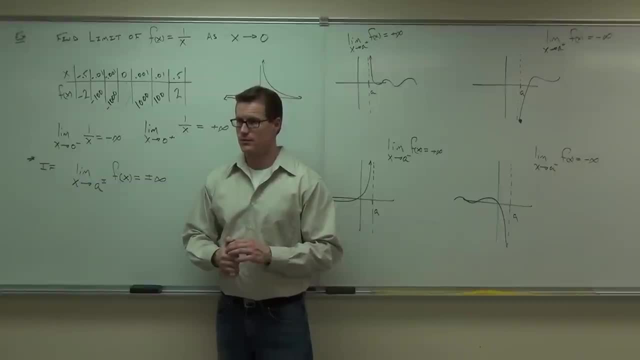 The two limits, for both the present and infinity, as they go towards the same point. what would it exist? The limit would exist, Yes, it would. So if we have a one-side limit this way and a one-side limit that way and they both go to positive infinity, yeah sure. 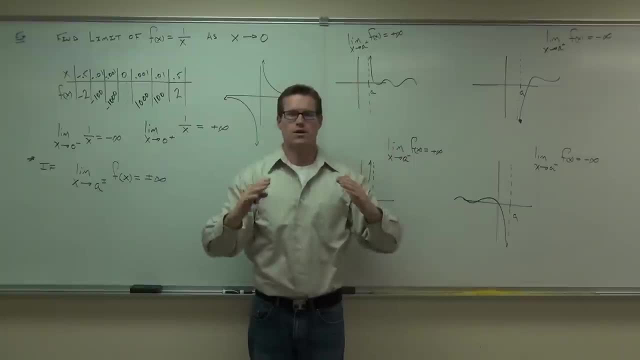 We'd say the limit is positive infinity because it goes from both sides. Or if the limit is going both, negative infinity that would exist. So let's see This way, yes, This way, yes, This way, no, This way, no. 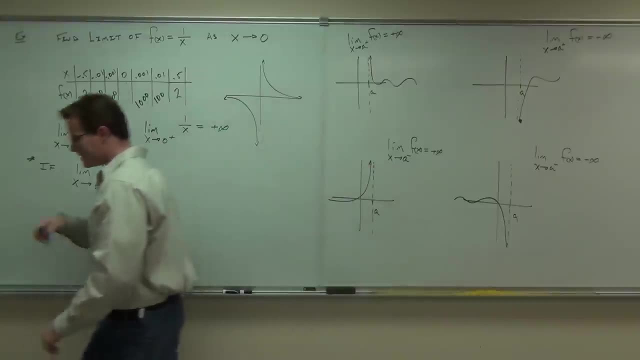 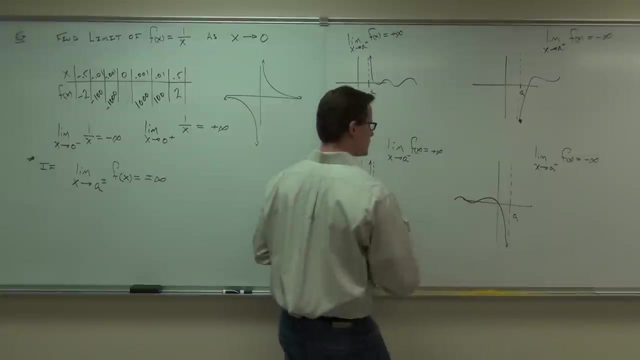 It takes practice to do that. by the way, I showed you that already. Just one question about this one. Yeah, It's approaching from the right. Should it be approaching from the left This one? No, the one above This one? 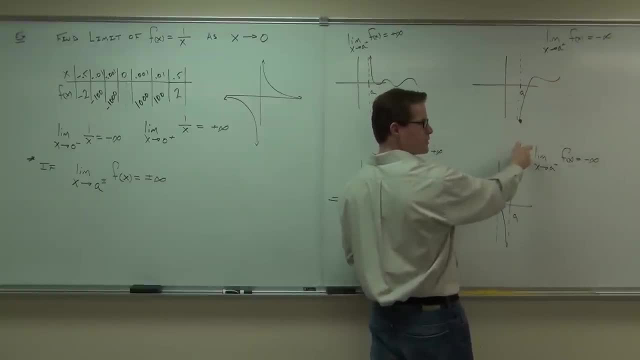 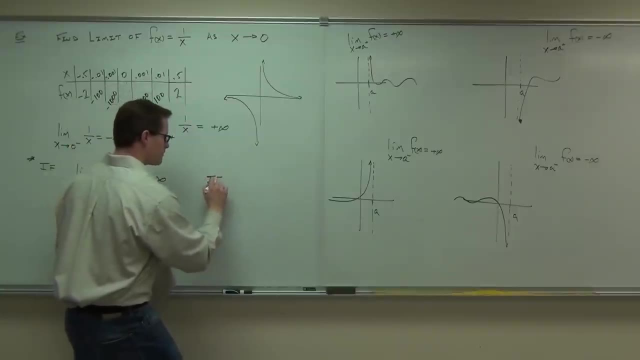 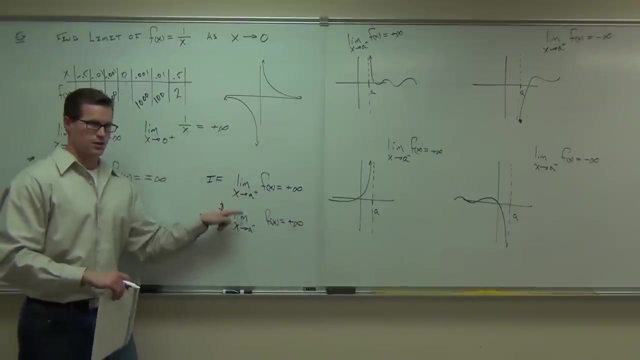 This is approaching from the right going to negative infinity. Oh, I see the plus now. Oh, never mind. Okay, Yeah, you know what? Let me write that out too. If this and this, do you see the thing here? 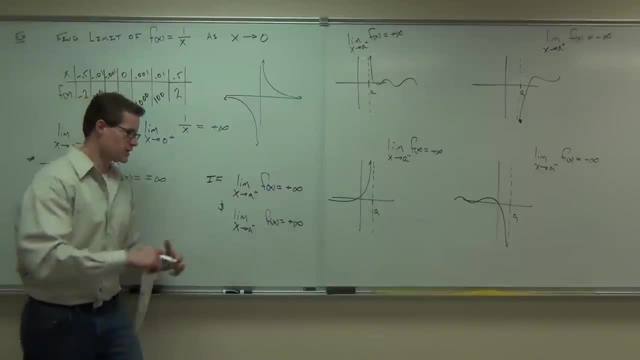 If we go from the right and from the left and they both go to positive infinity, then Okay, This was your question. Yes, Sure, If the two, if this works all the time, If the left-sided limit and the right-sided limit go.